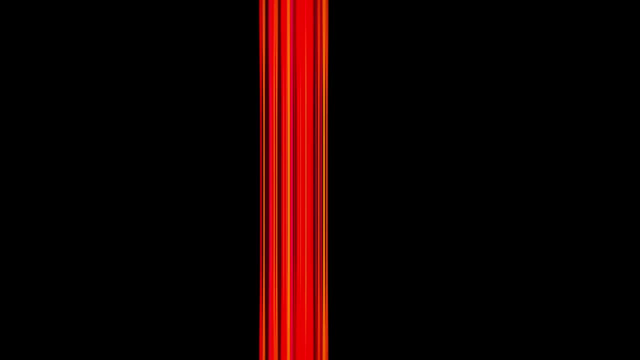 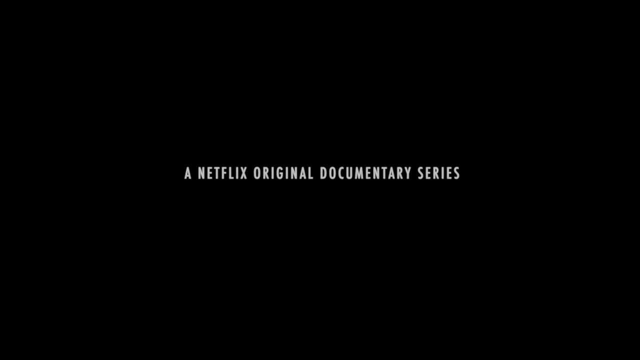 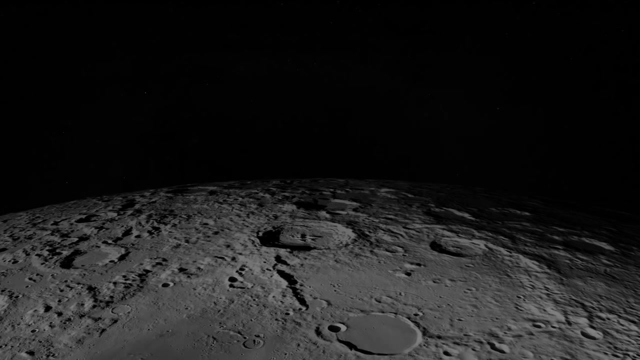 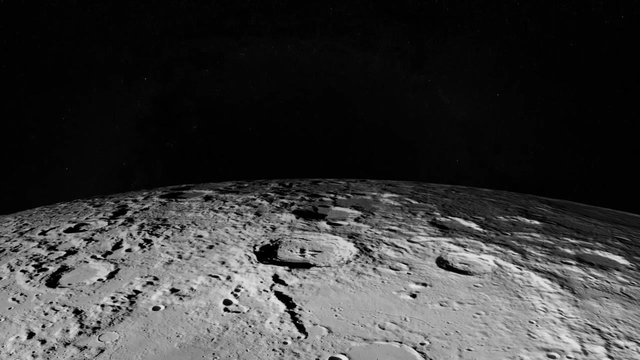 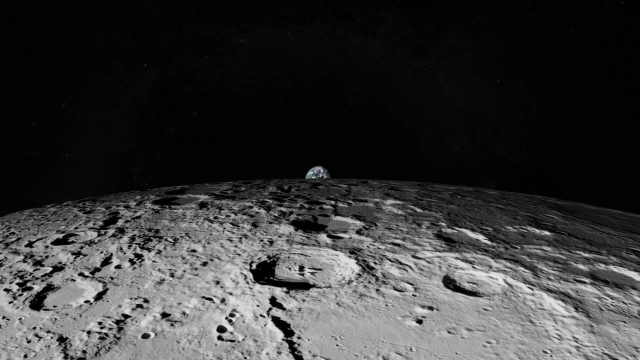 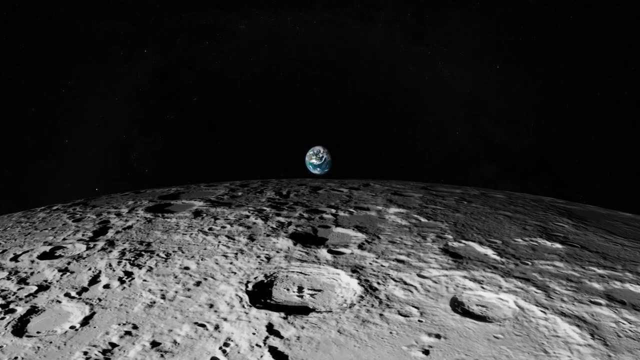 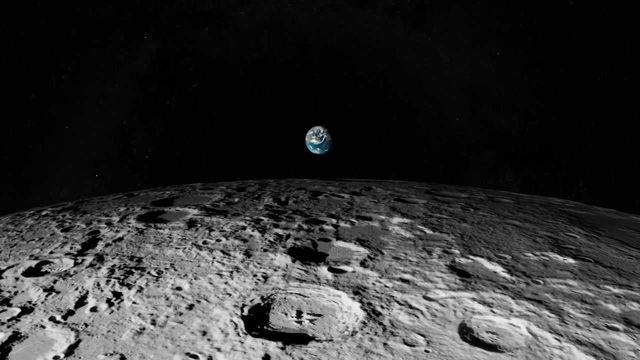 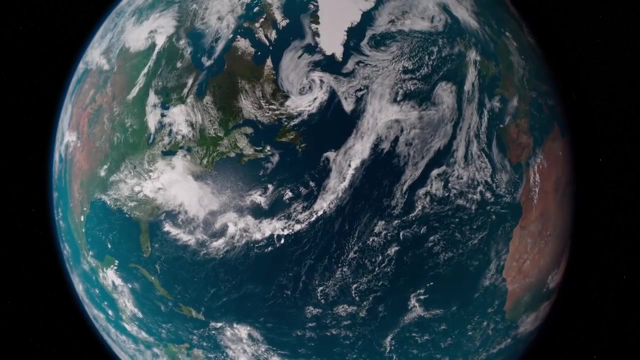 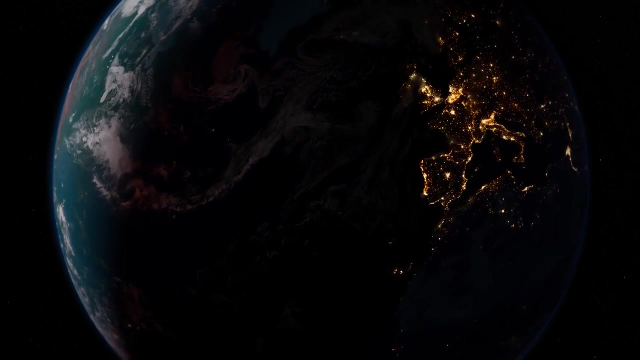 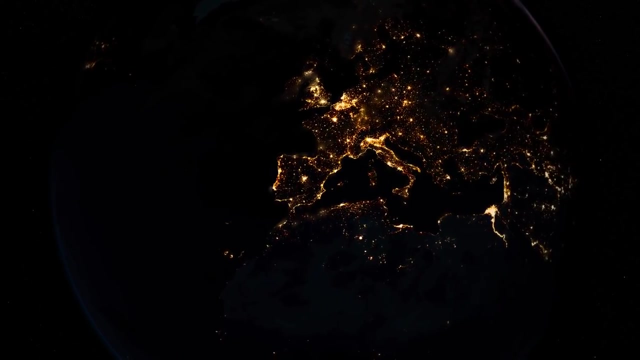 Just 50 years ago, we finally ventured to the moon. For the very first time we looked back at our own planet. Since then, the human population has more than doubled. This series will celebrate the natural wonders that remain and reveal what we must preserve. 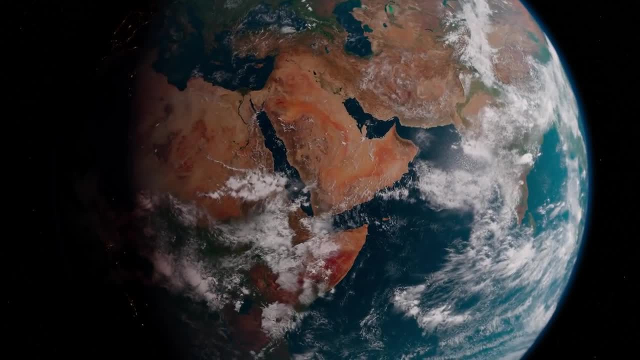 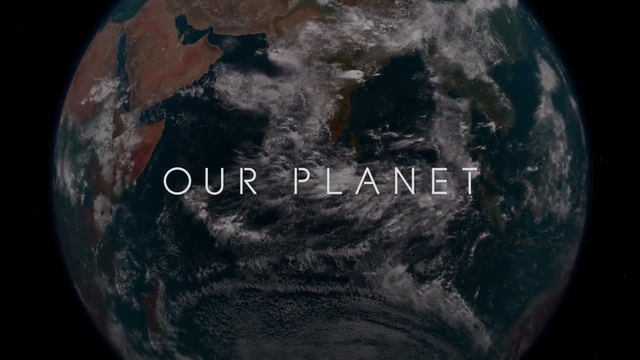 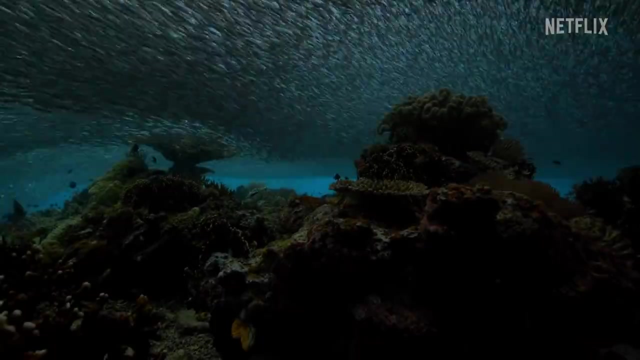 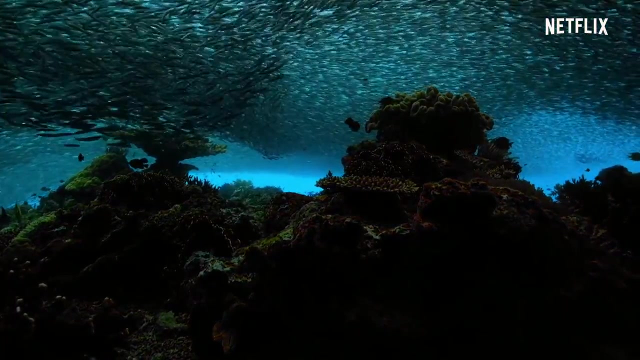 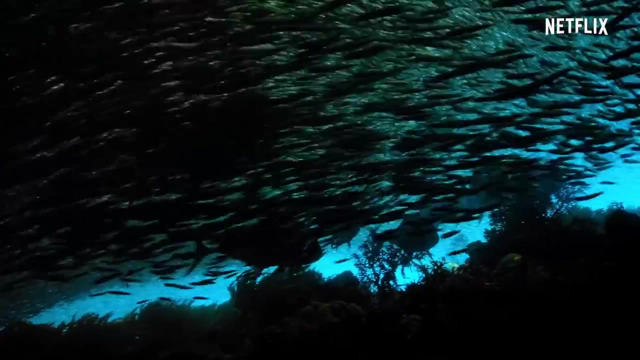 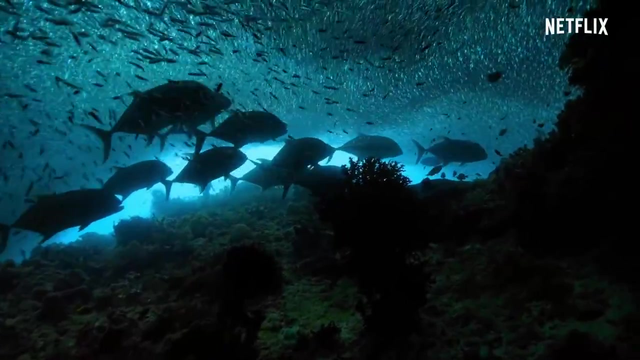 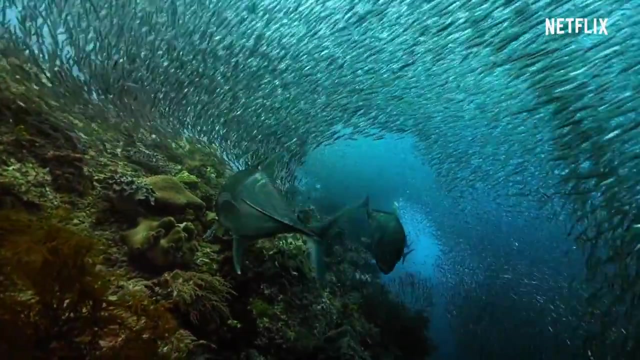 to ensure people and nature thrive. Immense shoals of fish throng our shallow seas. These are anchovies. Small fish in turn sustain bigger ones. Hunters: The fishers, The seafarers, The searchers, The hunters. 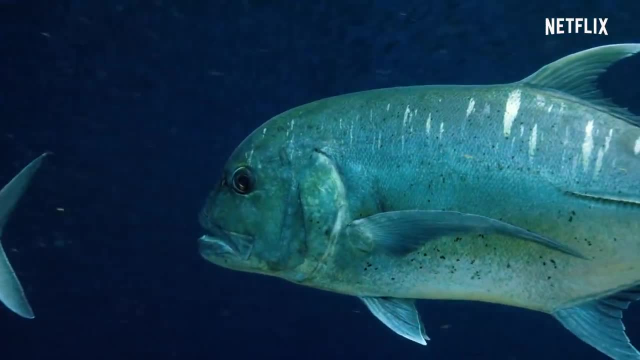 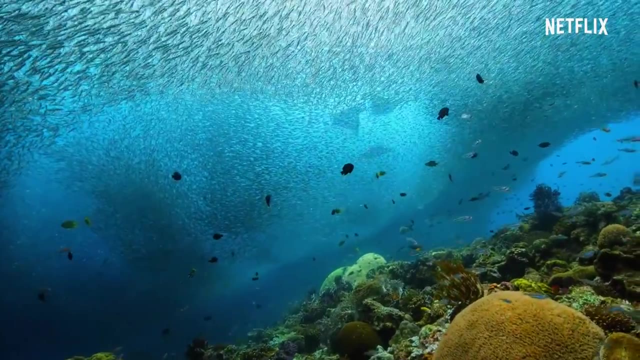 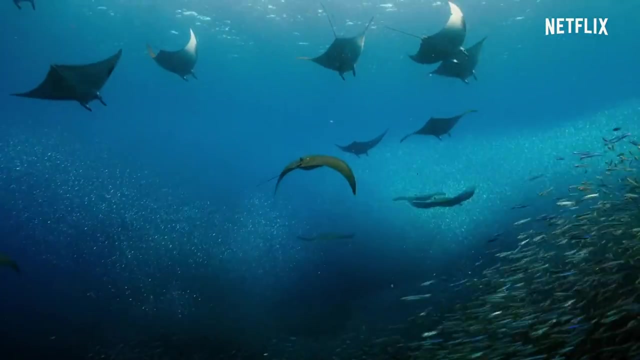 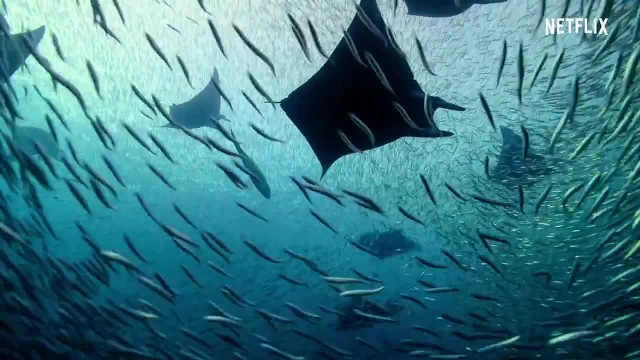 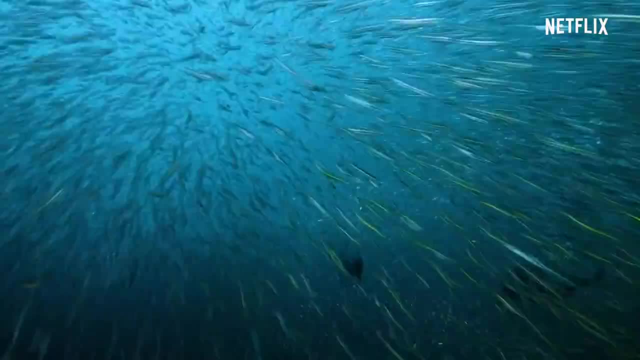 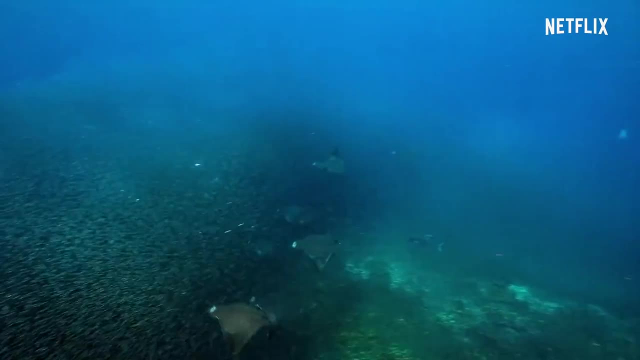 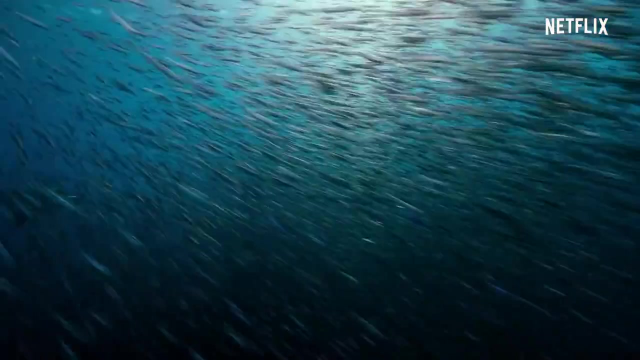 they become extremely efficient. It's the most important tool in the game. It'll give the hunter a unique environment, which is a place to break the ice. I found something here. I think I've been through this a lot, Touching the ice in a journey. 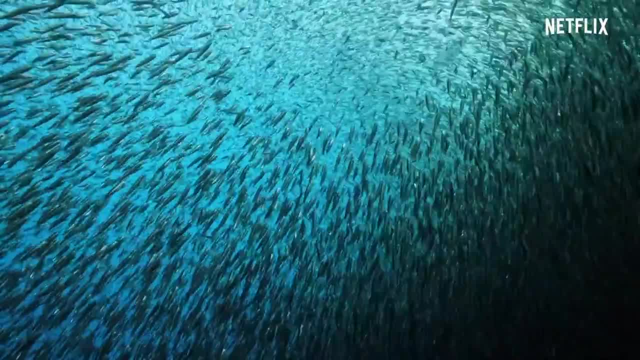 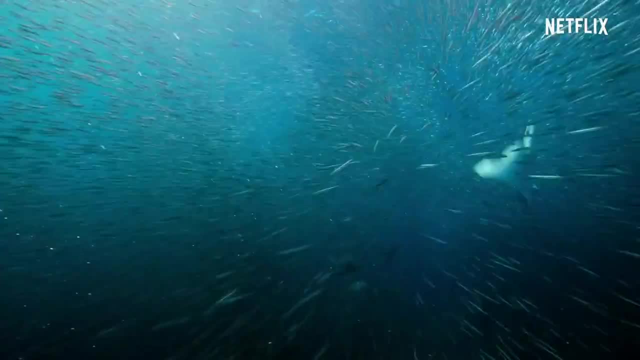 is the key to discovering new ways to survive, But it's not just about the hurtful. In order to survive, you need to know how to be a hero. You need to know how to be a hero. That's why I'm here today. 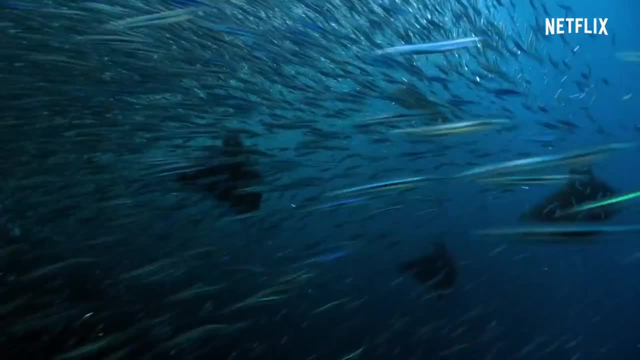 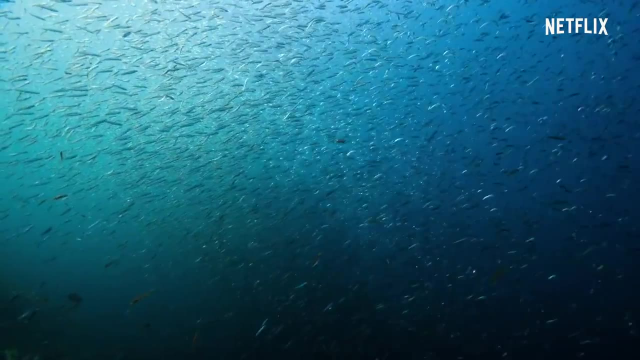 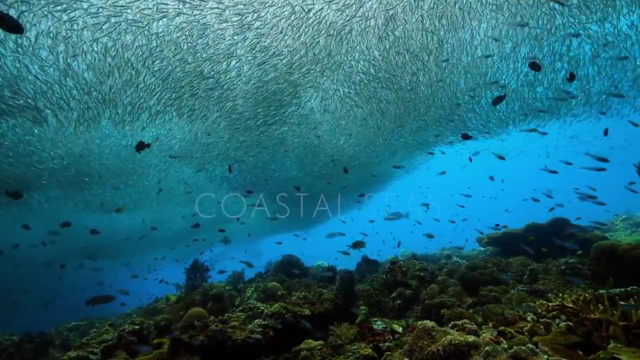 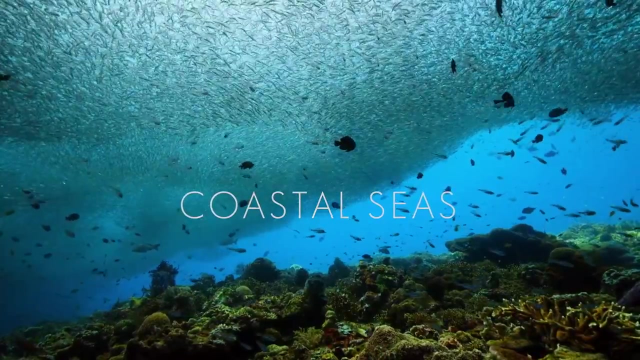 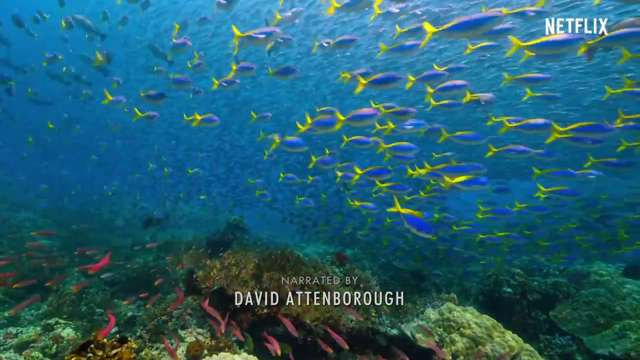 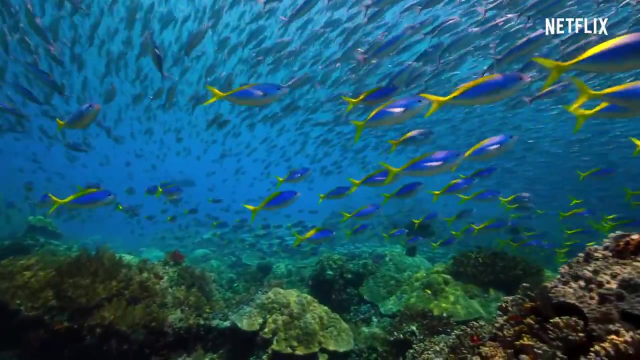 Because I know you can be a hero. The rich coastal seas are the fishing grounds of our planet and can provide an abundance of food for wildlife and humanity. The sea's fringing land make up less than a tenth of the world's oceans, Yet, astonishingly, 90% of all marine creatures live in these coastal waters. 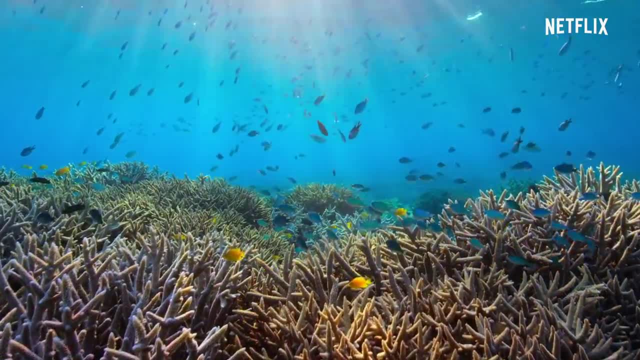 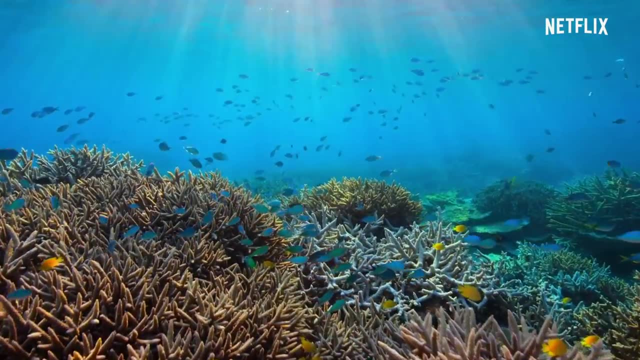 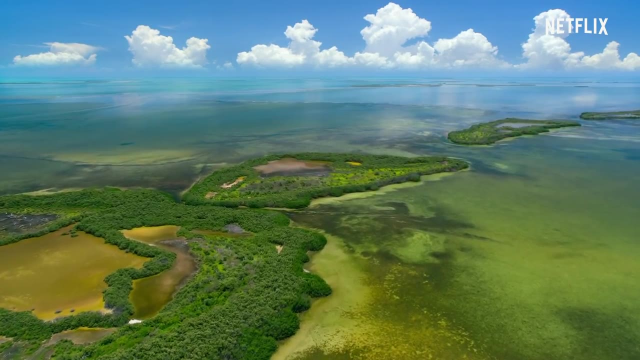 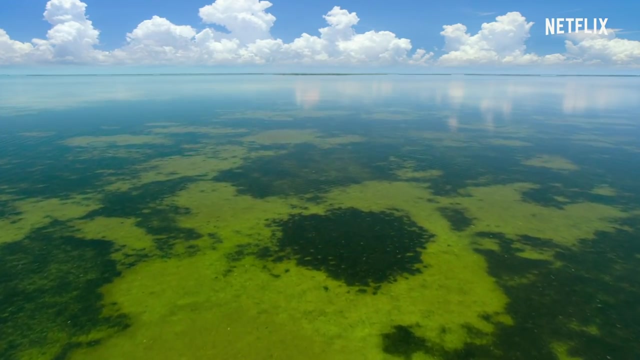 This superabundance is due to the fact that the seafloor here is within reach of sunlight. Everglades National Park in southern Florida, Fields of seagrass carpet the shallow tropical waters. The sea is a place of peace and tranquility. 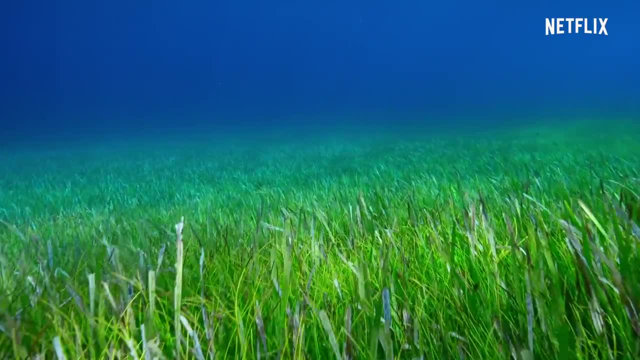 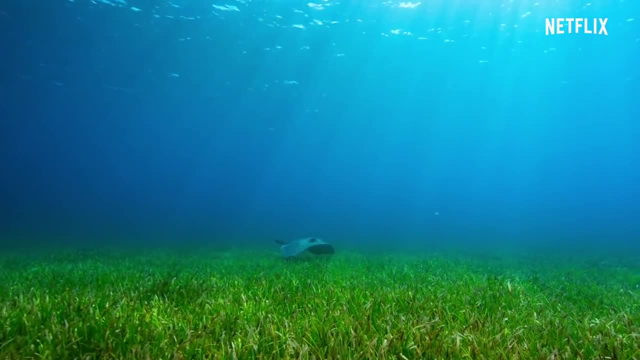 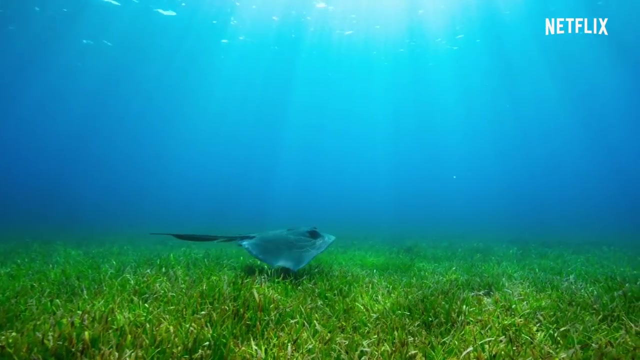 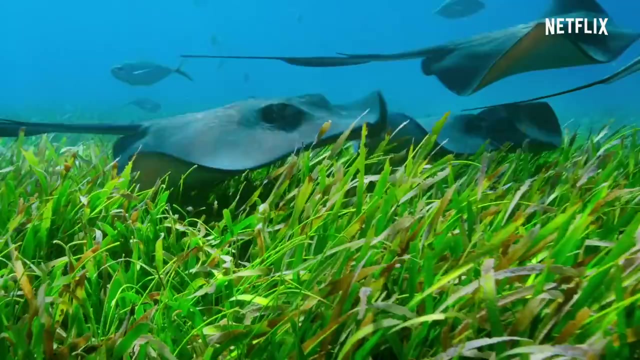 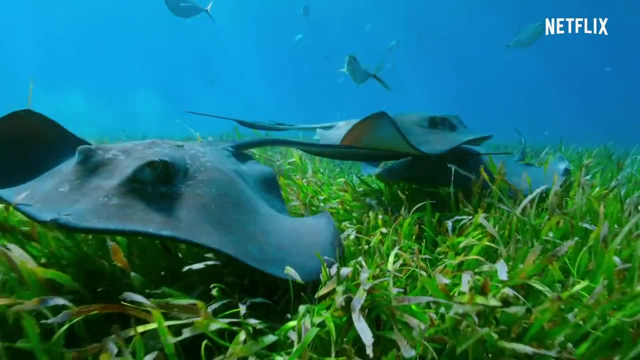 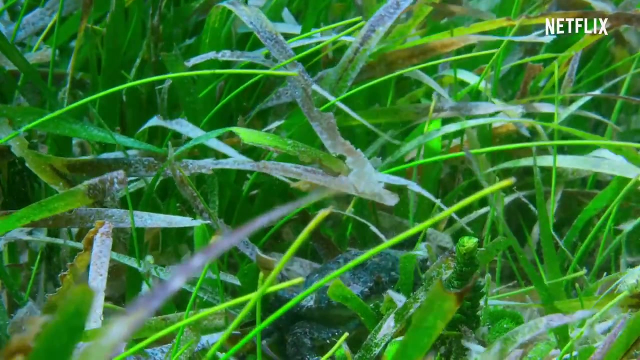 The sea is a place of peace and tranquility. Like savannas on land, these lush marine meadows support a great variety of animal life. Stingrays search for prey hiding in the seagrass. Stingrays search for prey hiding in the seagrass. 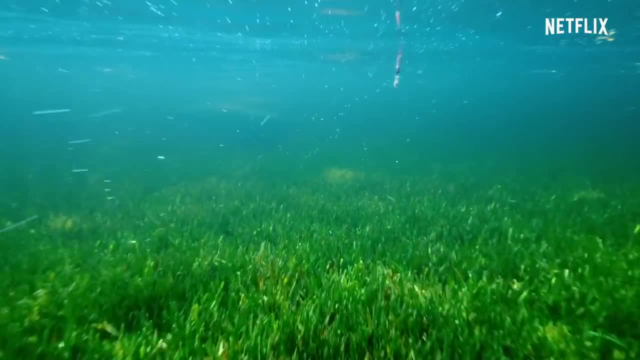 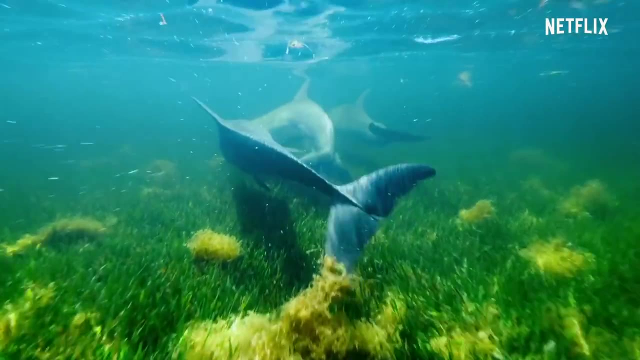 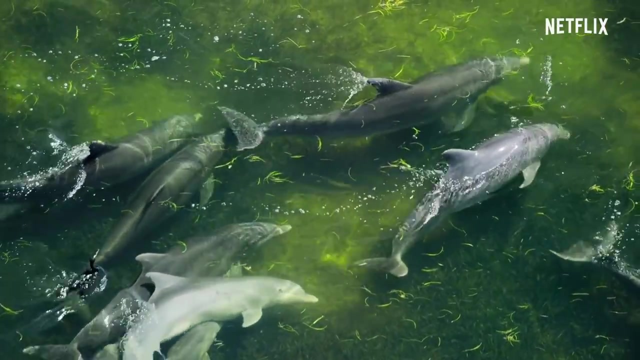 The Everglades are also the hunting grounds of the coast's most ingenious fishermen, Bottlenose dolphins S İşq'alqqqqqqqqqqqqqqqqqqqqq. They search for food using echolocation, a type of sonar. 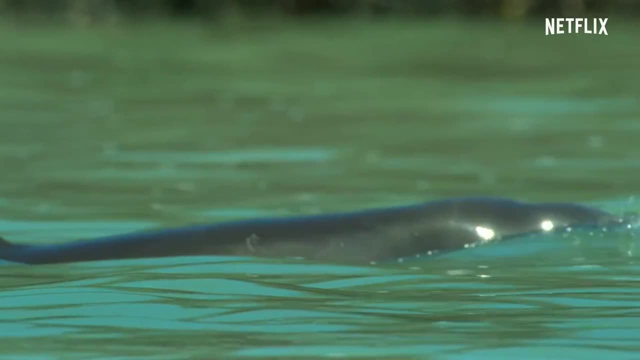 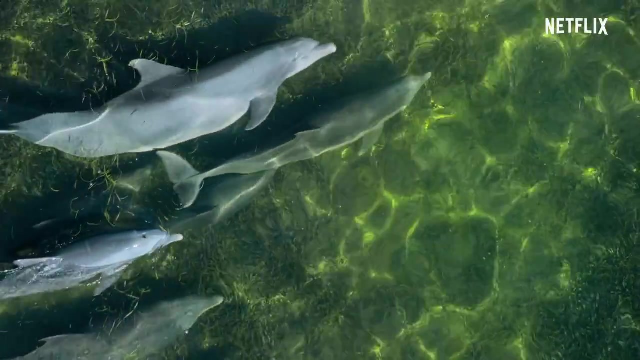 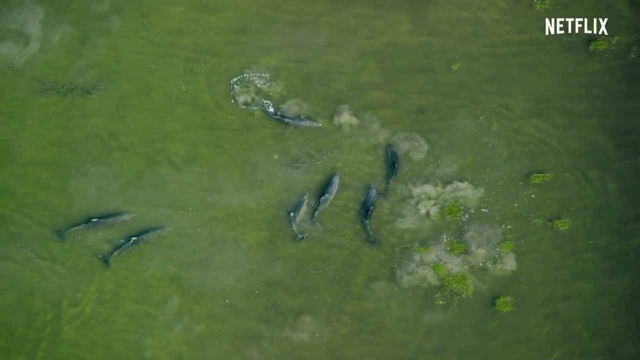 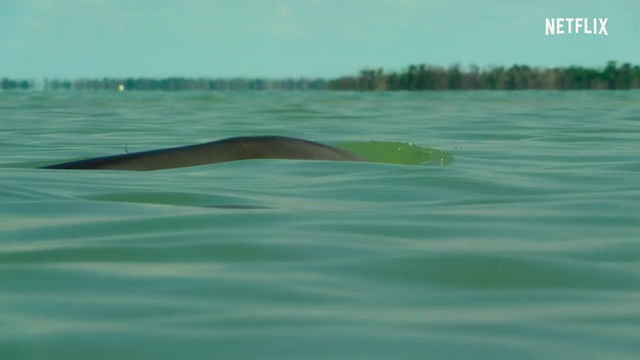 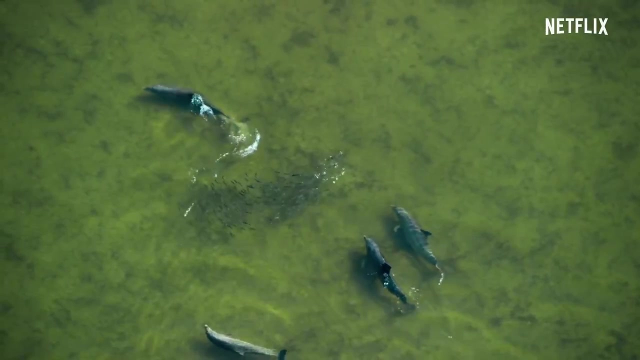 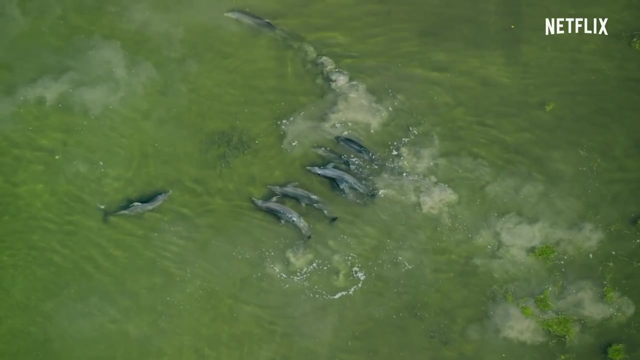 Ahead of them, a shoal of mullet. A shoal of mullet. These particular dolphins have developed their own special way of catching their prey. They carefully herd the fish into just the right place. Then one dolphin stirs up a ring of mud that encircles the shoal. 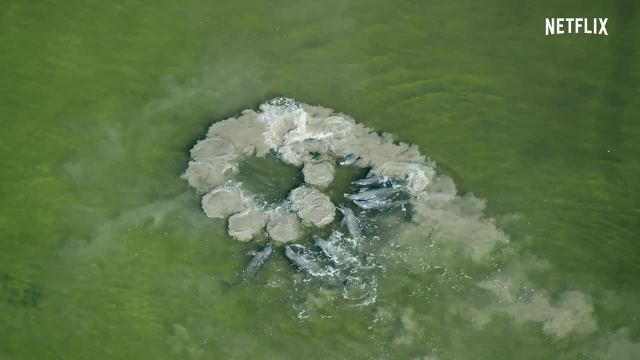 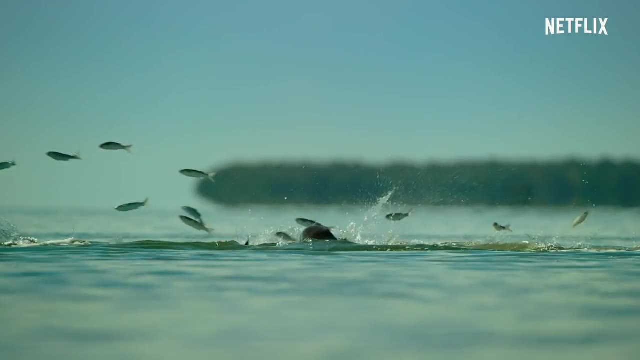 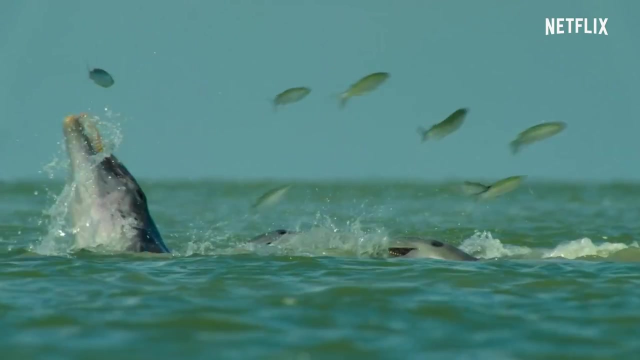 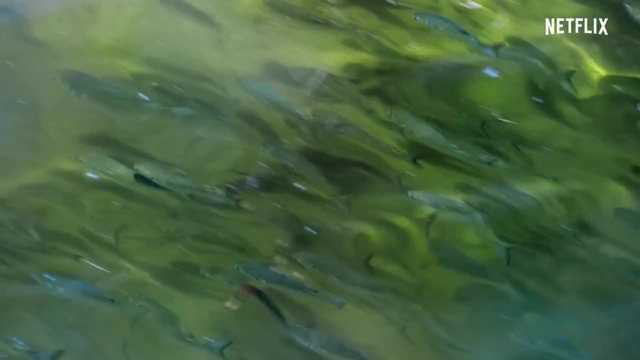 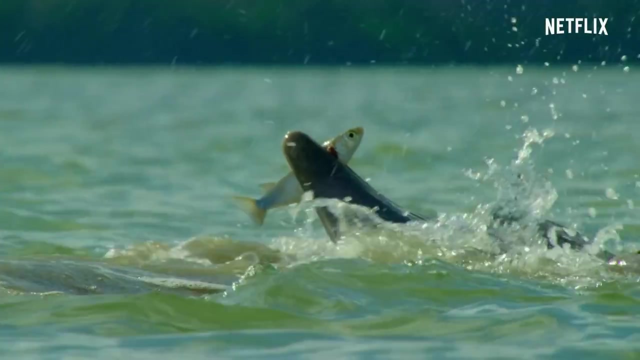 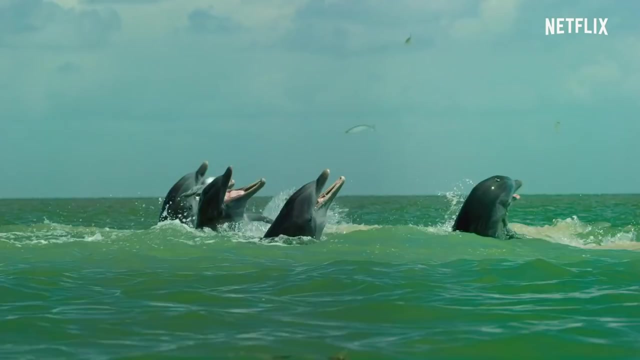 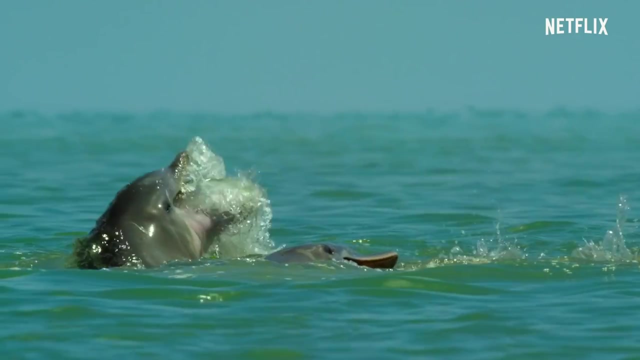 The fish panic and take to the air Most escape. Catching flying fish isn't easy, But the dolphins move on and take another, helping A little bit of a spin And a little more. A good spin, A good spin And a good spin. 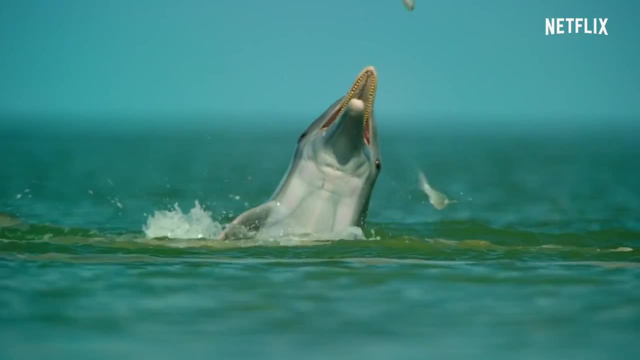 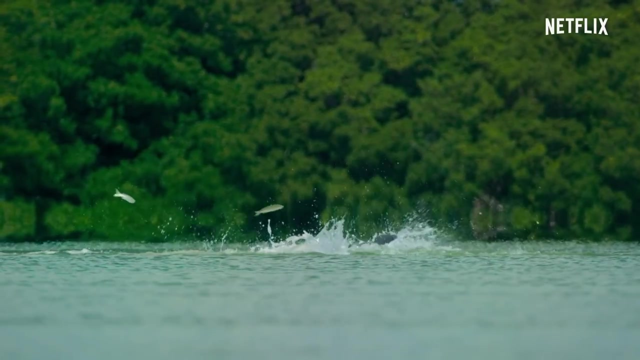 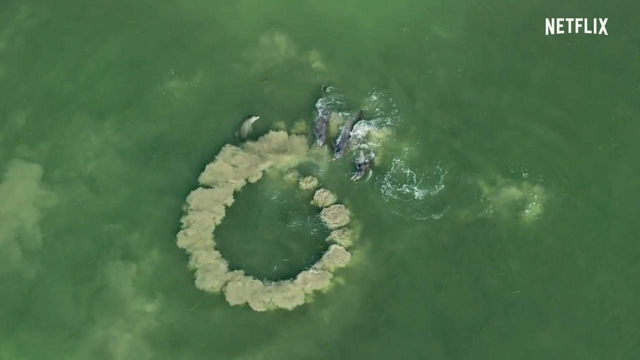 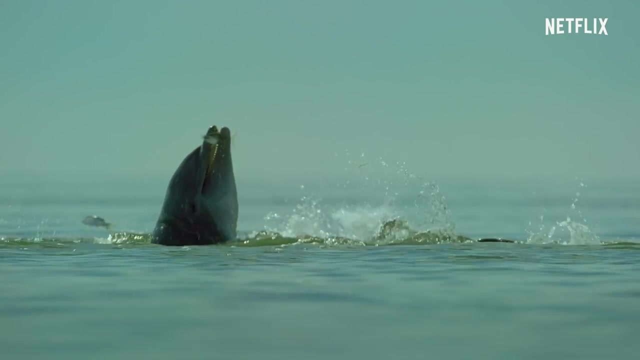 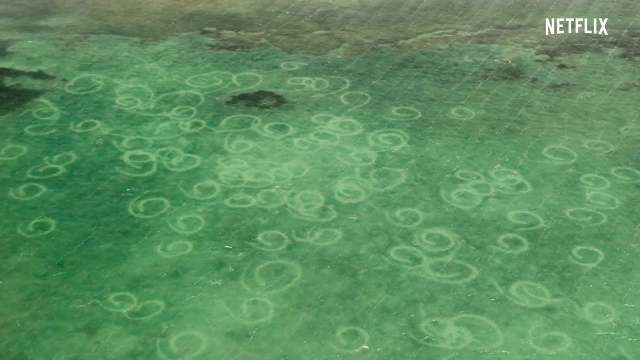 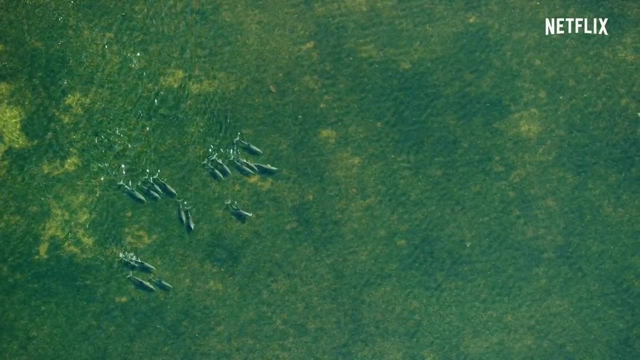 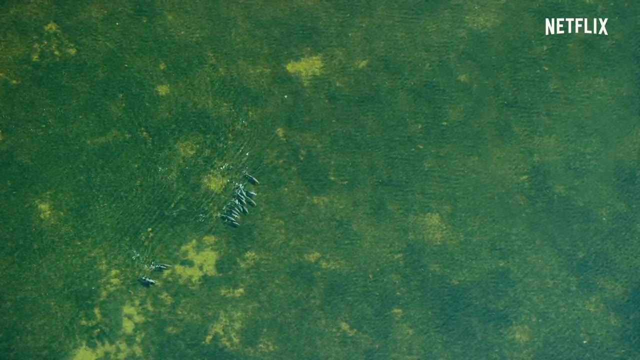 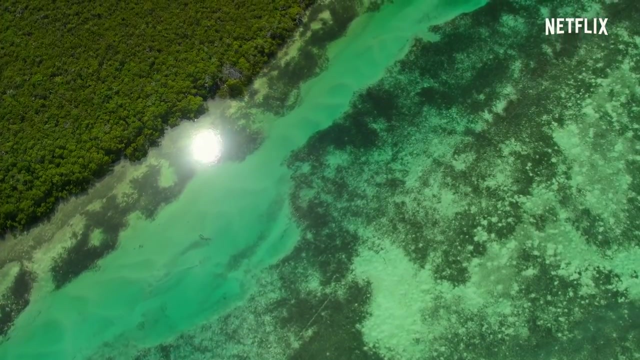 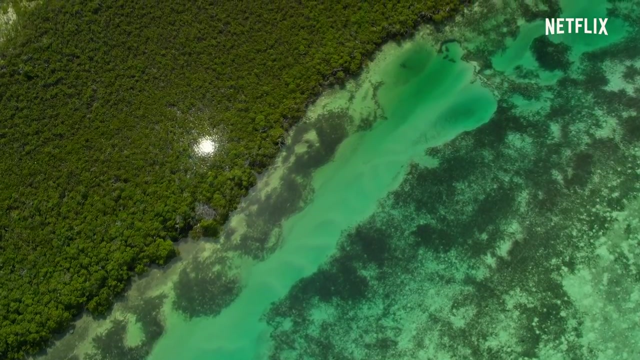 the shallow seas are vitally important in the fight against climate change. seagrass absorb 35 times as much carbon dioxide as the same area of rainforest, and that reduces the damage caused by the recent warming of our seas. mangroves often border the seagrass meadows. 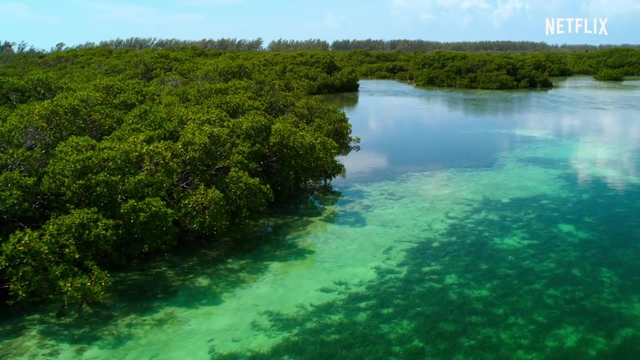 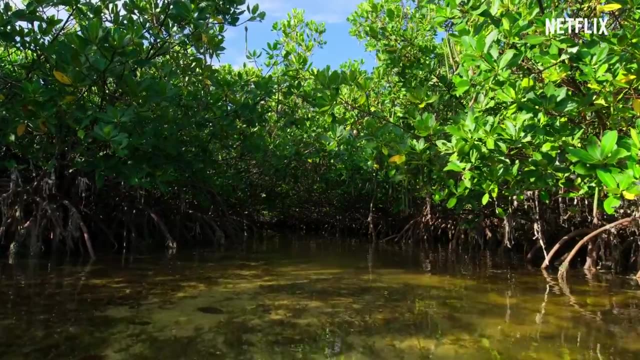 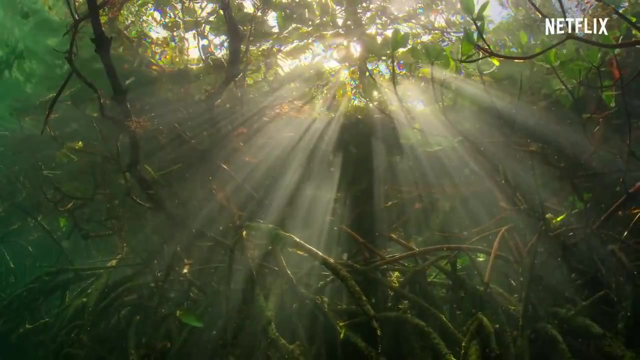 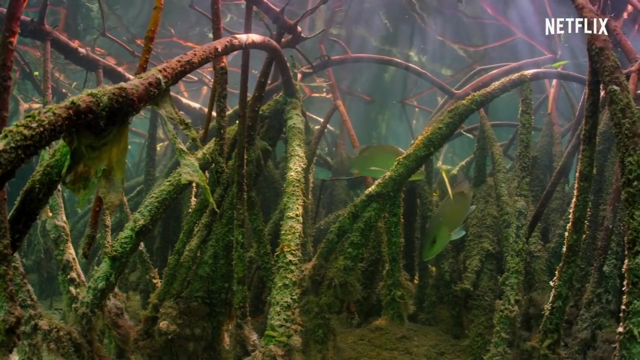 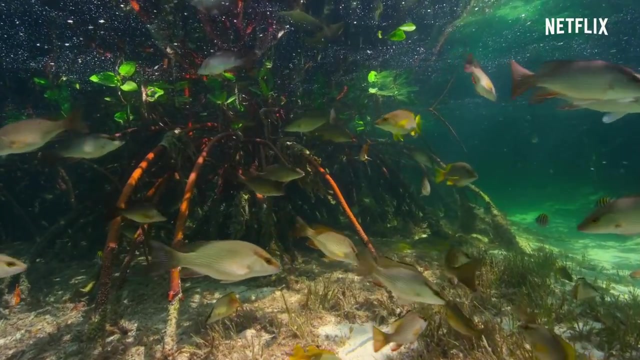 these remarkable trees are the only ones that can cope with the varying saltiness of coastal waters. they not only protect our coasts from the destructive forces of hurricanes, but also, like seagrass, capture carbon dioxide. they, their tangled roots, create safe nurseries for young fish, which will eventually leave the mangroves. 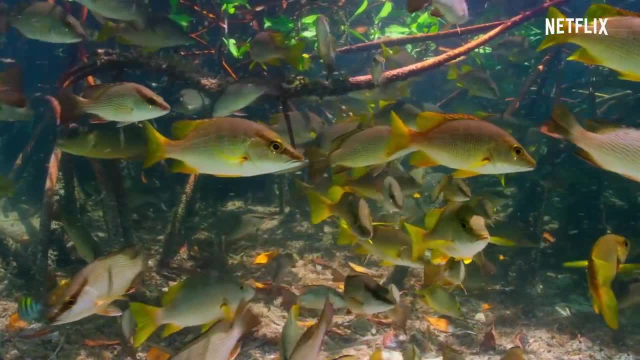 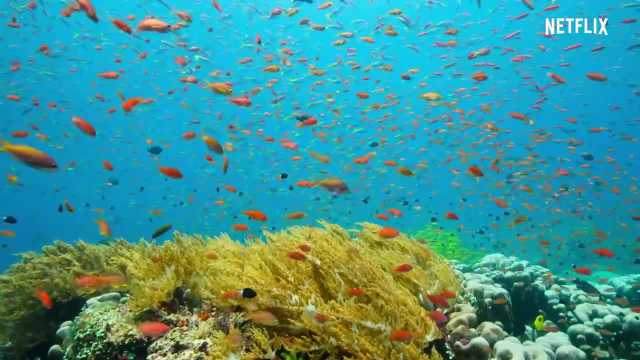 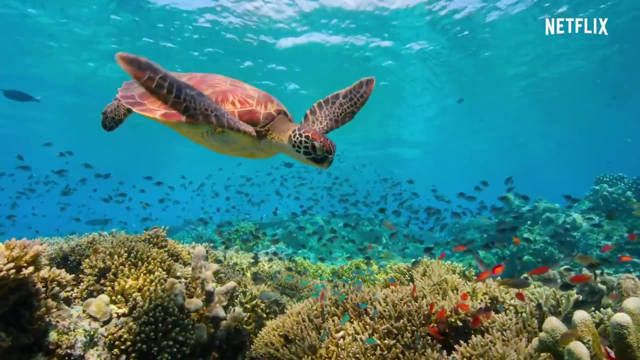 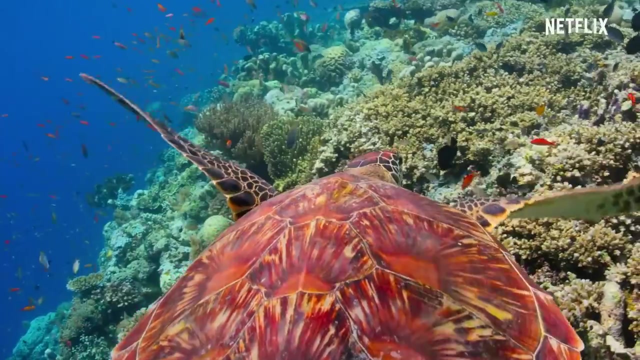 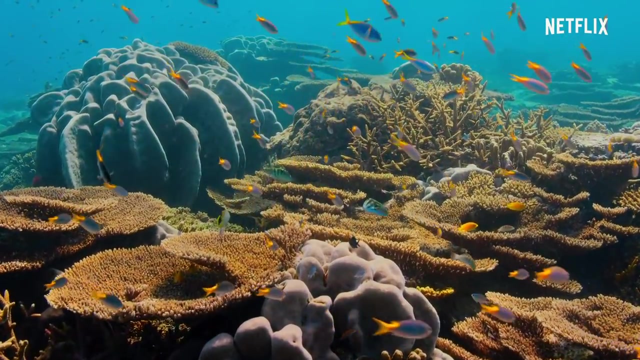 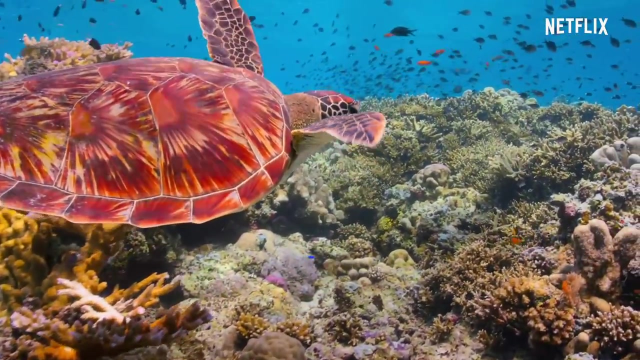 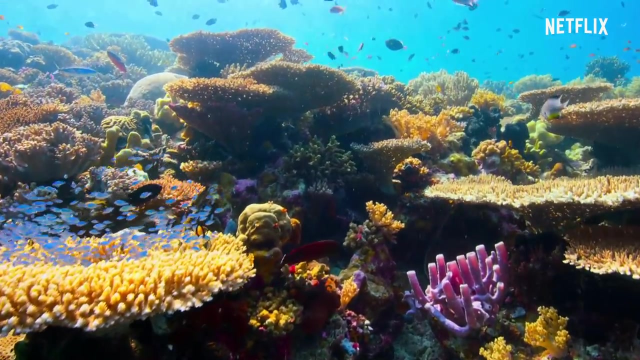 and make their homes in the tropical seas most magical wonderlands: coral reefs. these reefs cover less than one percent of the sea floor, yet they are home to a quarter of all marine species. none of these creatures would be here were it not for the coral. corals create the structures that provide food and shelter on which the entire community depends. 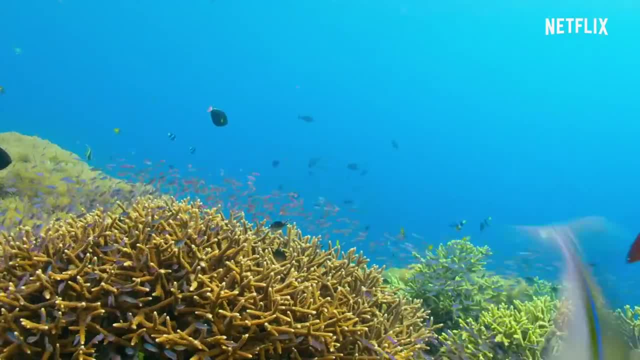 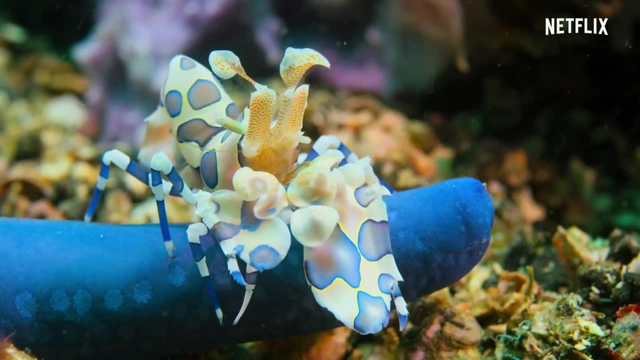 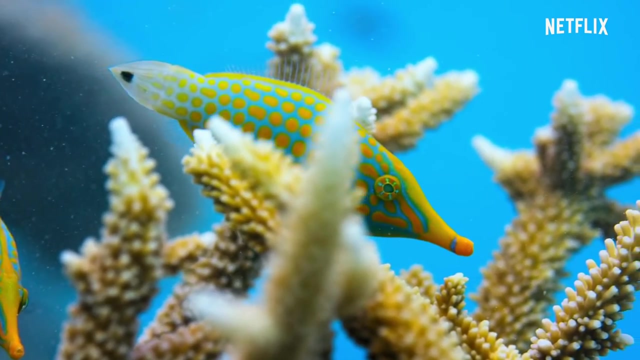 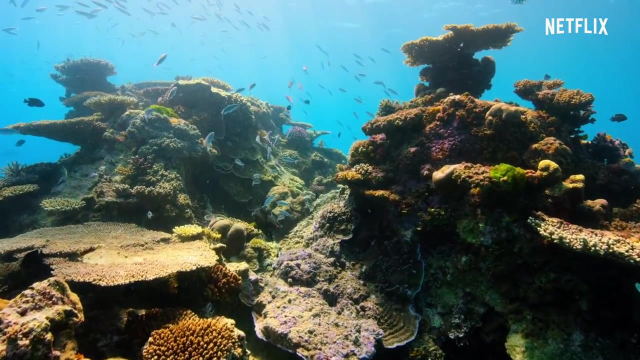 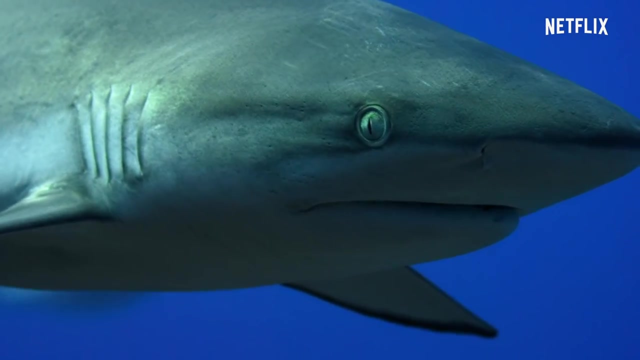 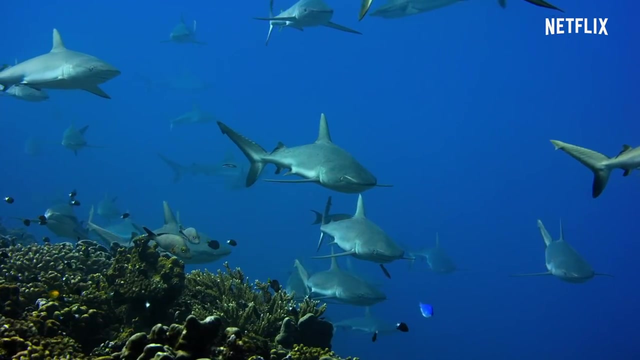 every resident has a role to play in maintaining the health of the reef. unfortunately, few reefs are as pristine as they once were and most are now missing. one extremely important member of the community: sharks. relentless overfishing has reduced shark populations around the world by over 90%. 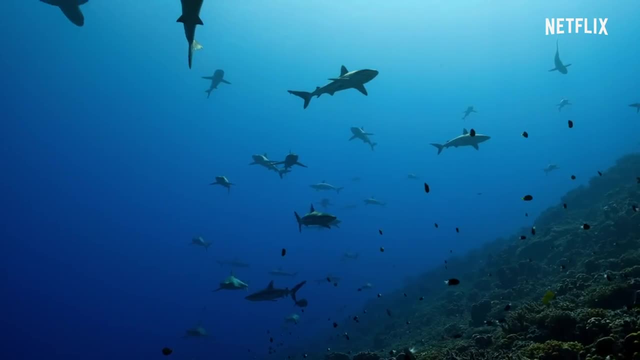 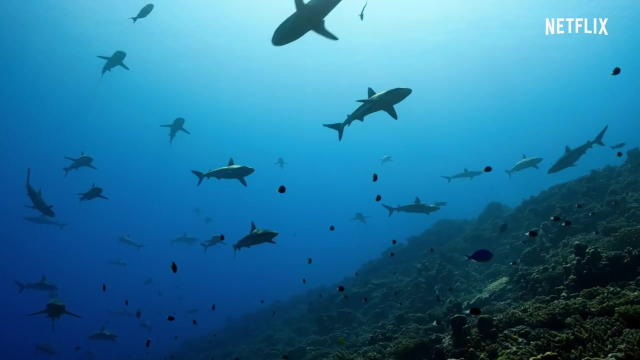 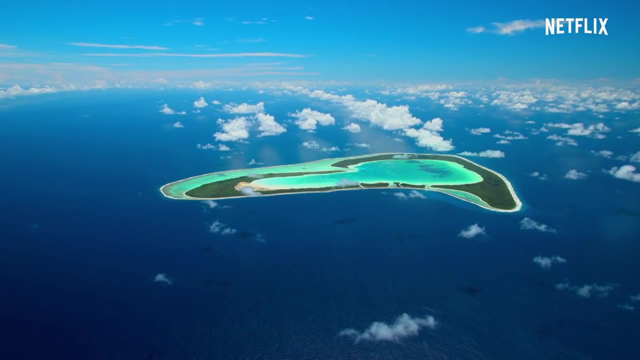 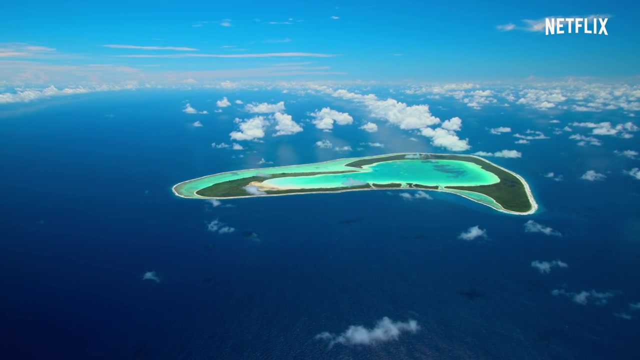 today they only thrive in anything like their former numbers on the very remotest of reefs. French Polynesia, in the middle of the world, in the middle of the world, in the middle of the world, in the middle of the pacific ocean. here at least, sharks are fully protected. 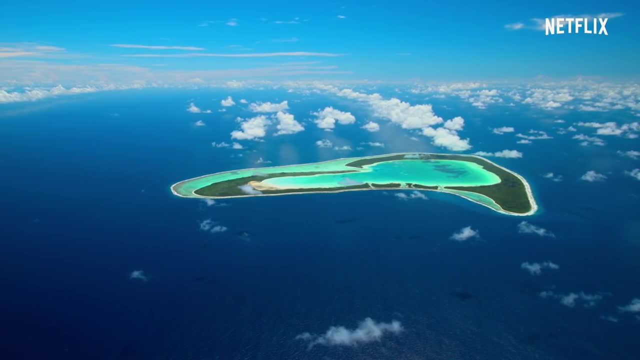 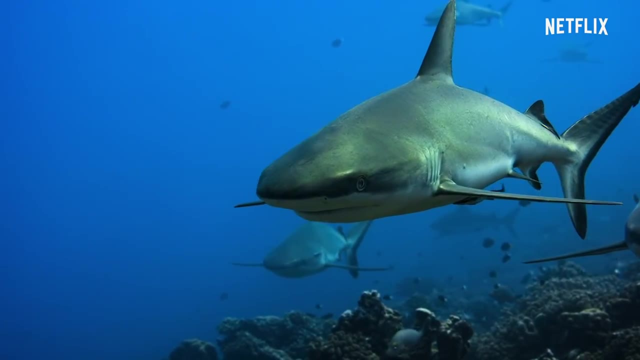 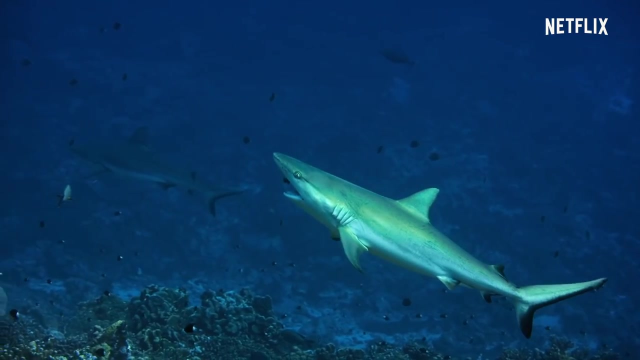 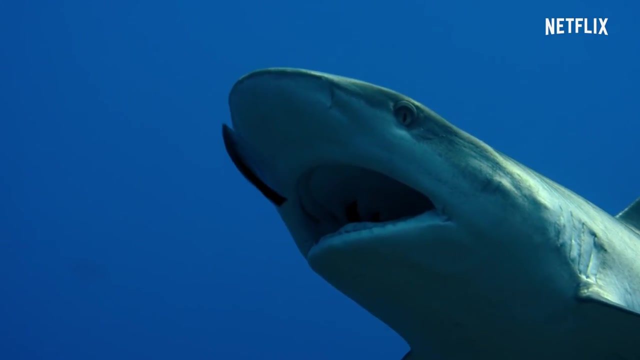 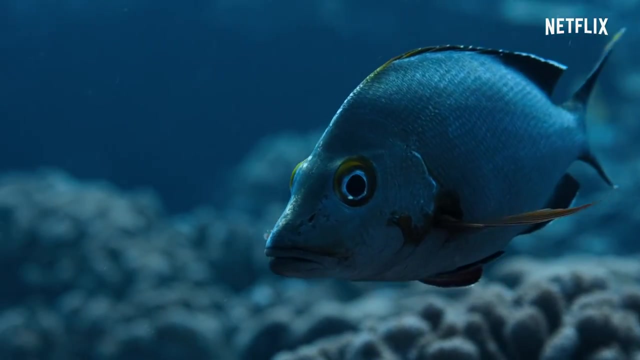 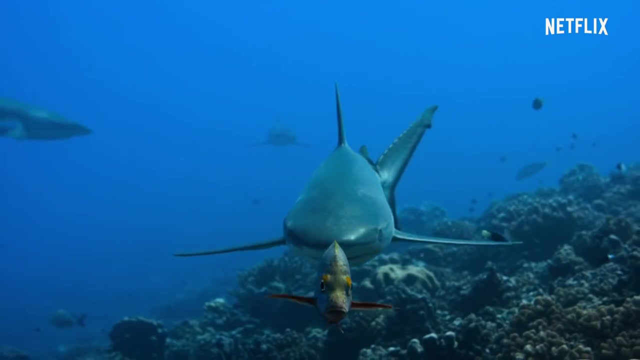 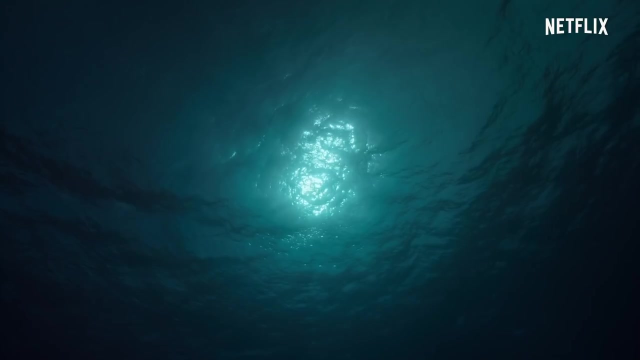 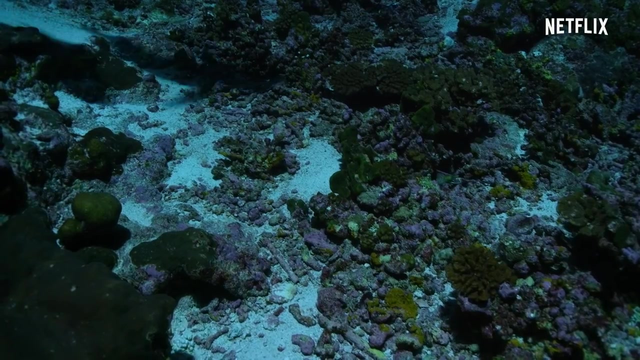 by day. grey reef sharks hang in the current. they let little wrasse pick their teeth clean in readiness for the night's hunt ahead. these sharks prefer to hunt in darkness, when their acute senses give them an advantage over their prey. nightfall time for small fish to take refuge within the nooks and crannies of the reef. 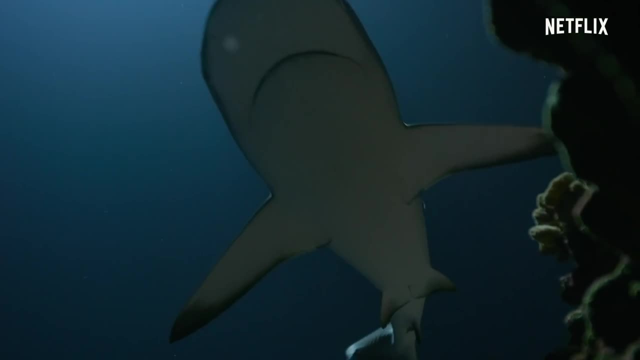 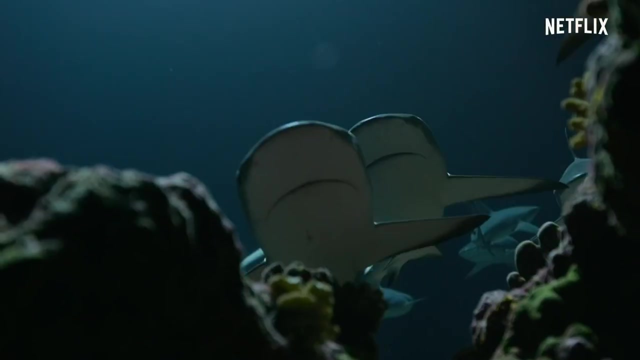 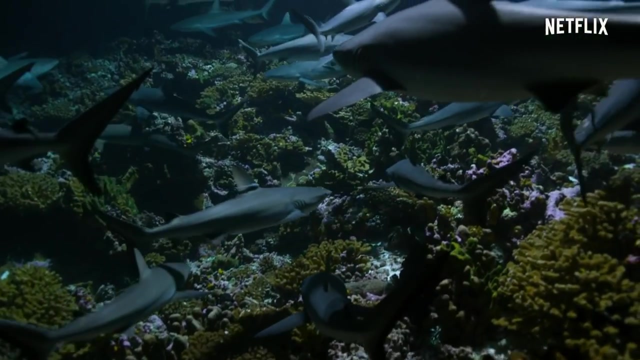 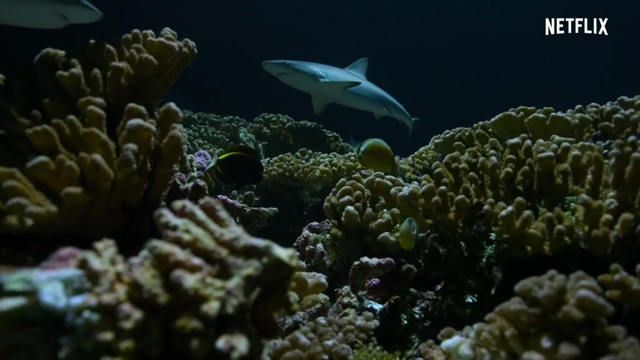 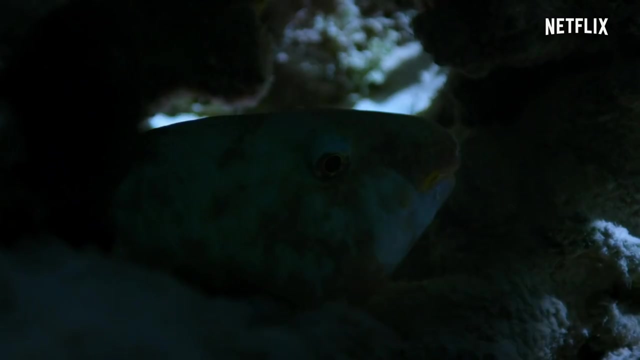 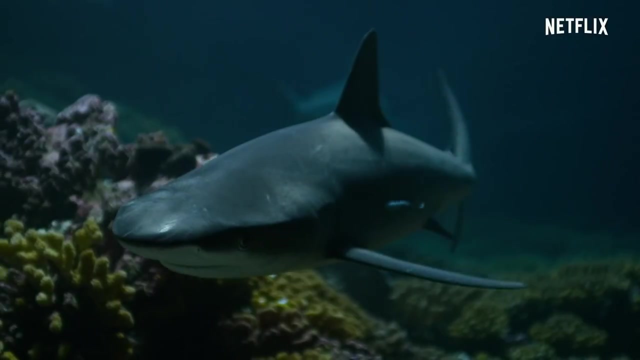 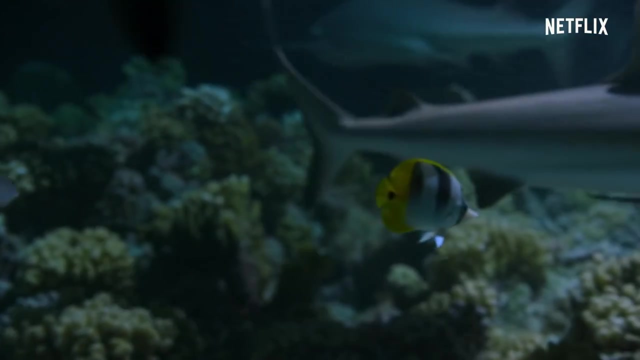 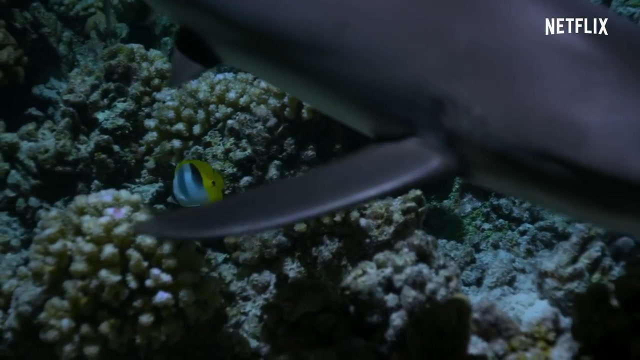 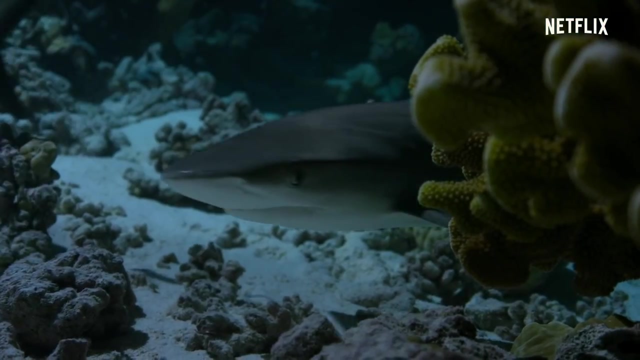 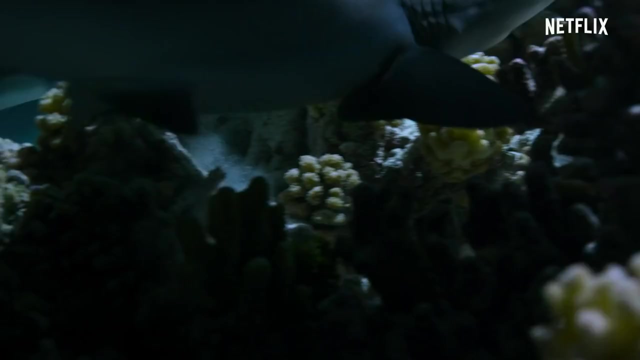 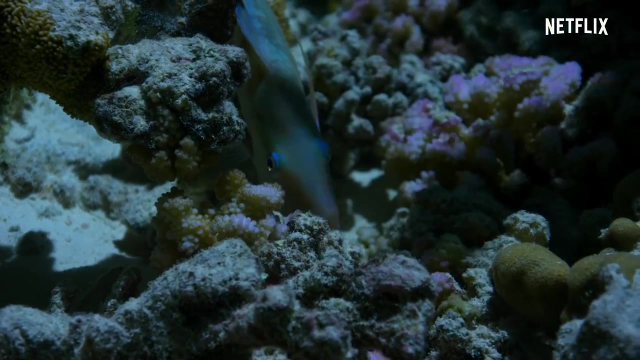 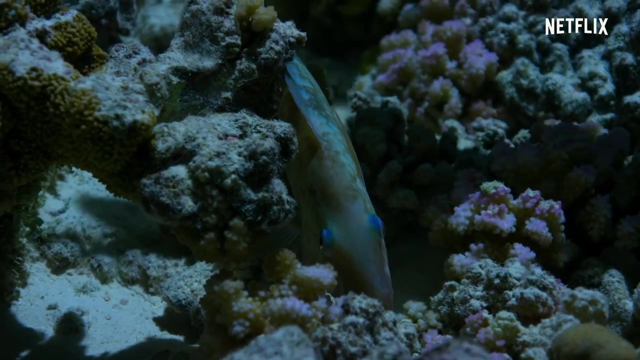 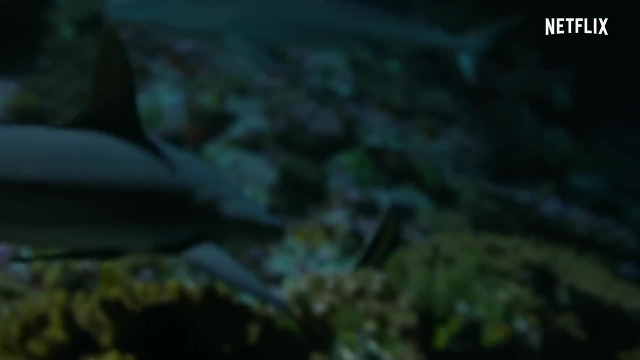 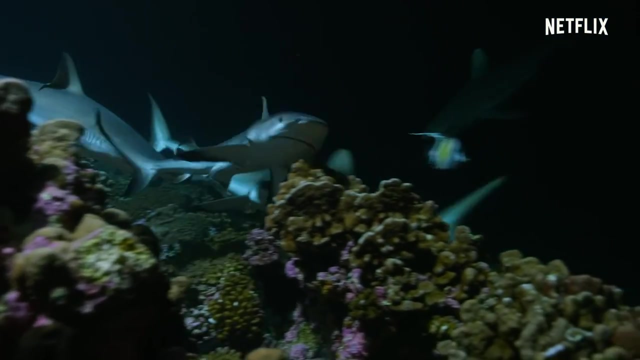 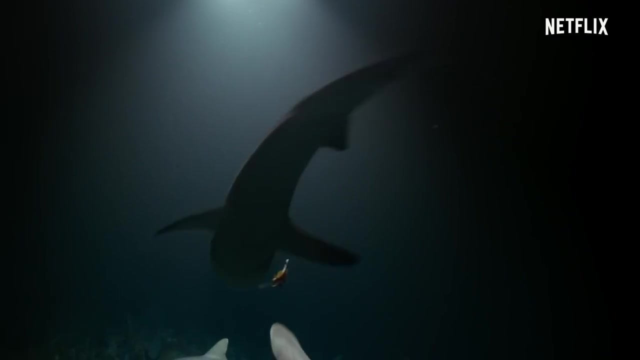 beyond the reach of the grey reef sharks. small fish can trap animals. sharks can detect the slightest movement. small fish can detect the slightest movement. Breaking cover is dangerous. Stay motionless and the sharks may not detect you. A little fish may outmaneuver a single shark. 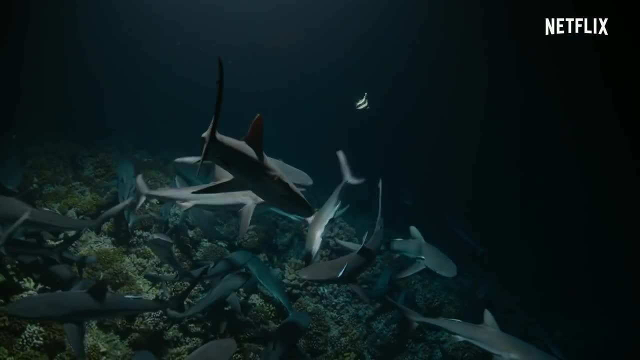 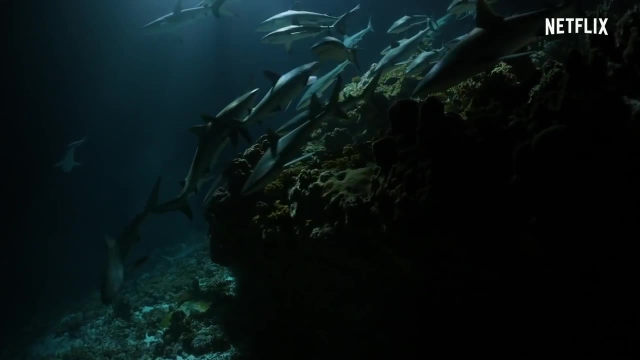 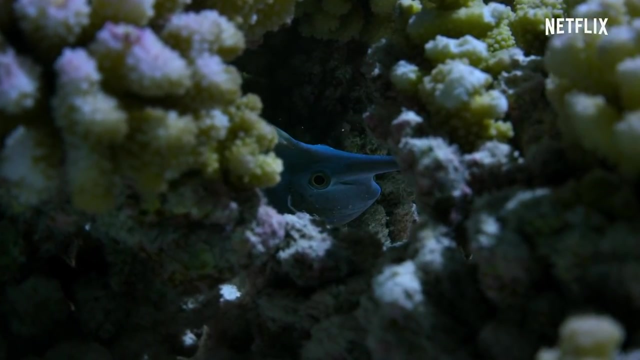 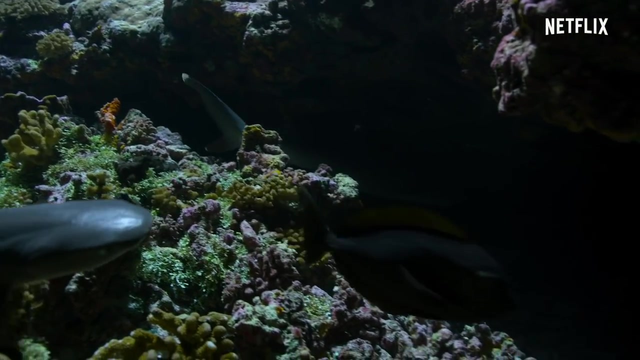 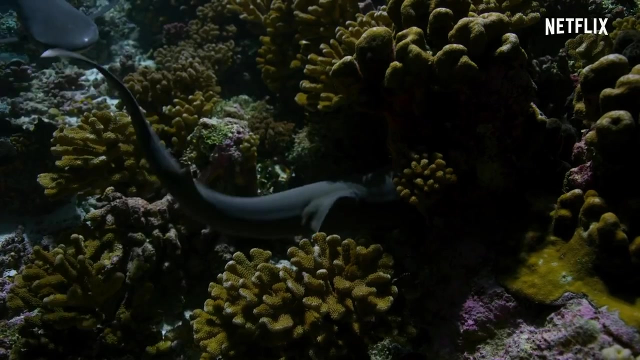 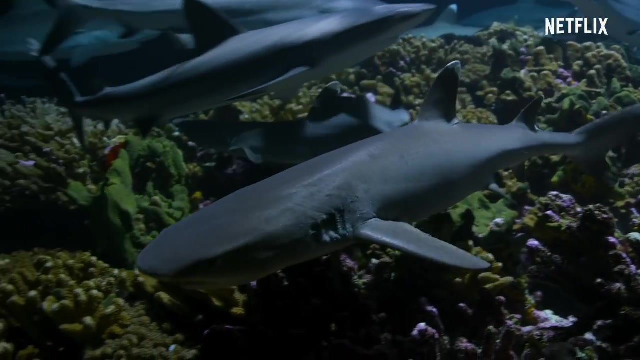 but with so many hunters there is little chance of escape. sheltering within the coral branches is usually the safest option, but the arrival of a second hunter changes everything. white tip reef sharks. slender and more agile. the white tips can get into hiding places other hunters can't reach. 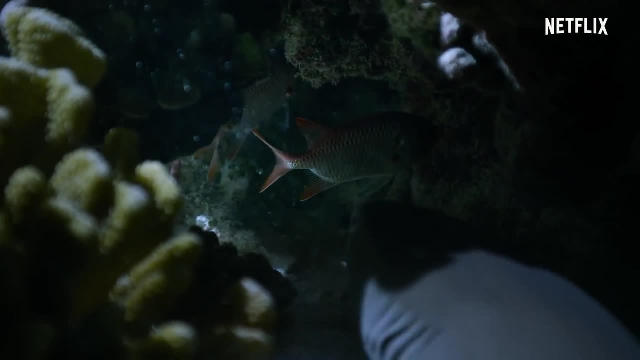 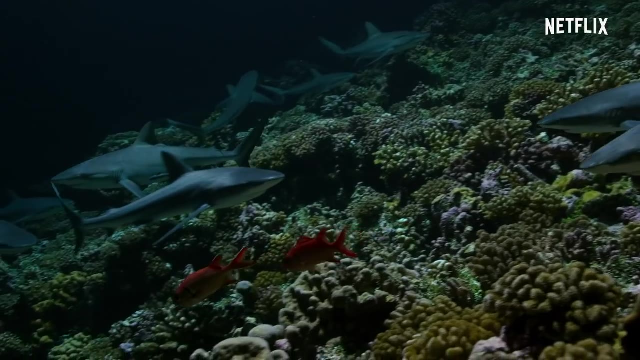 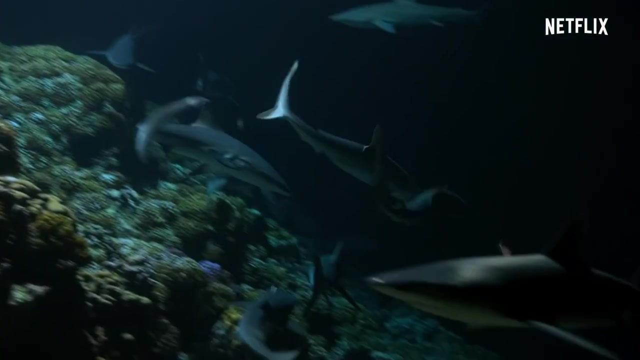 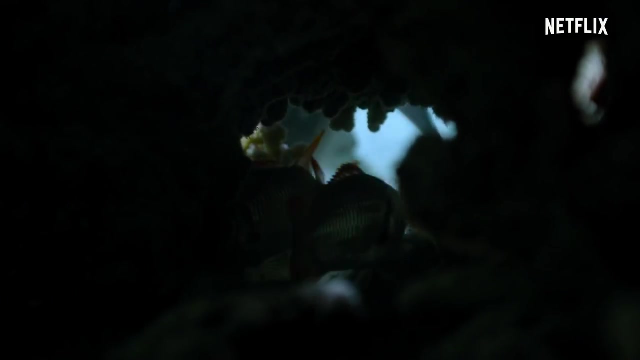 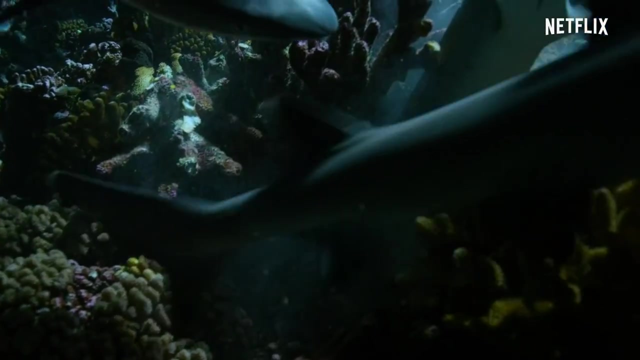 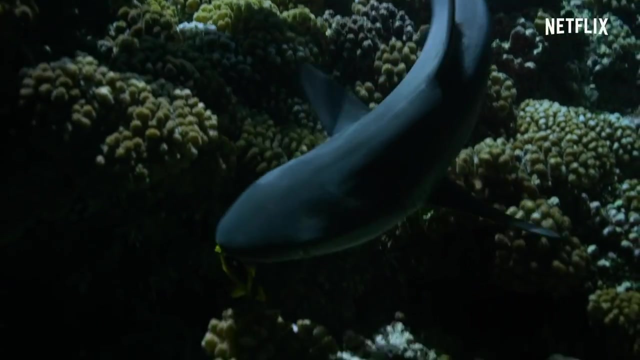 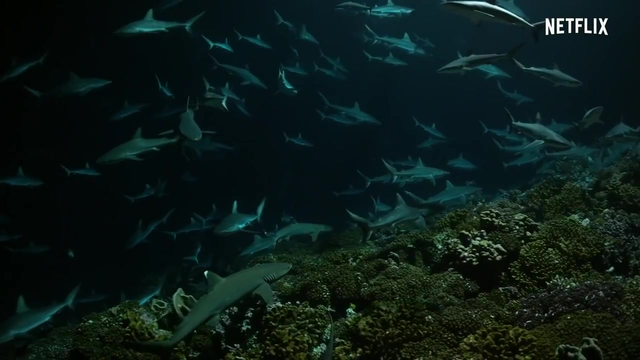 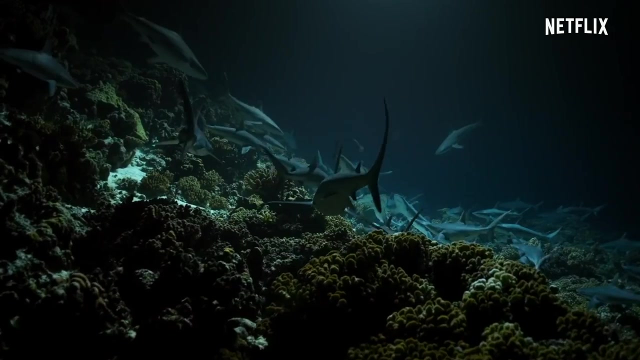 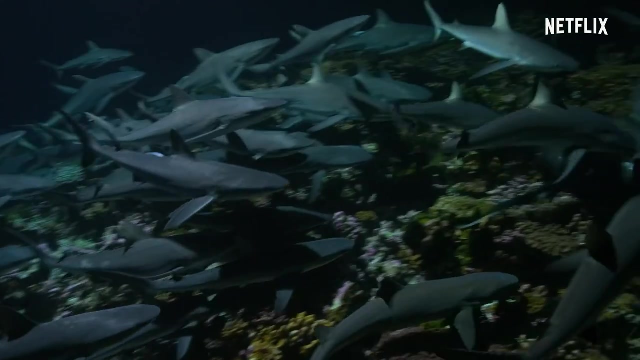 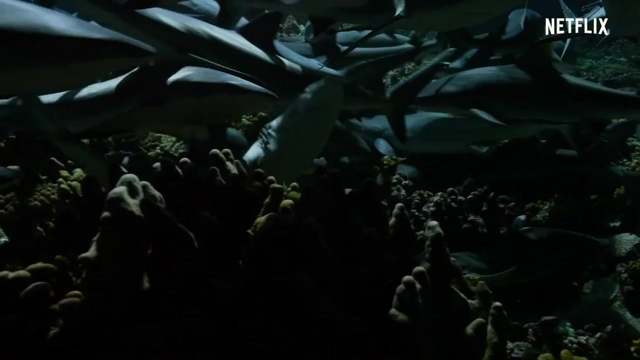 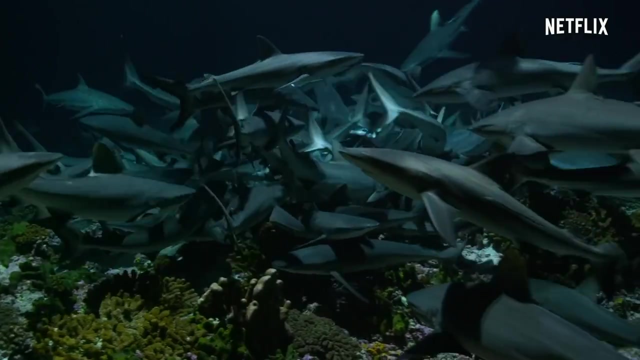 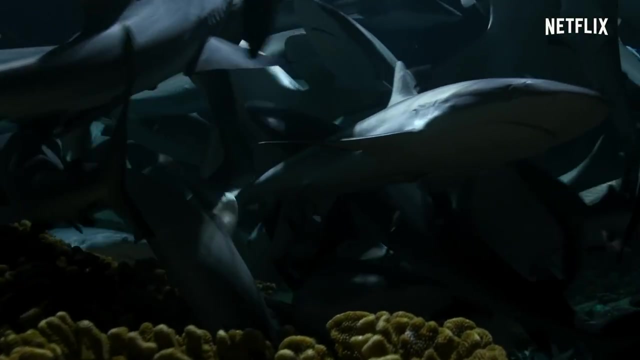 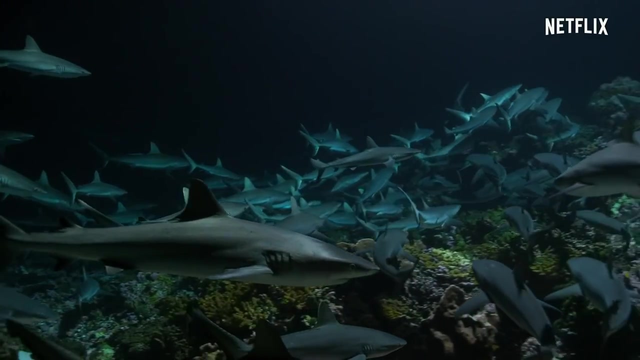 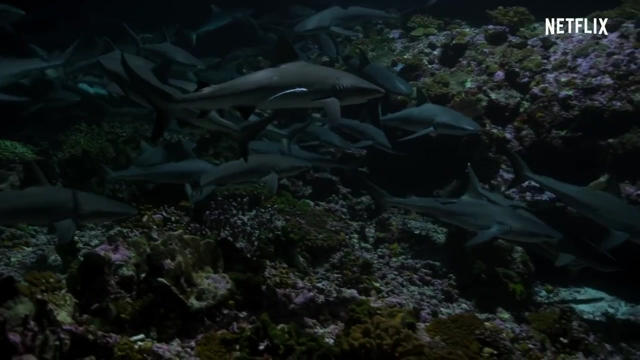 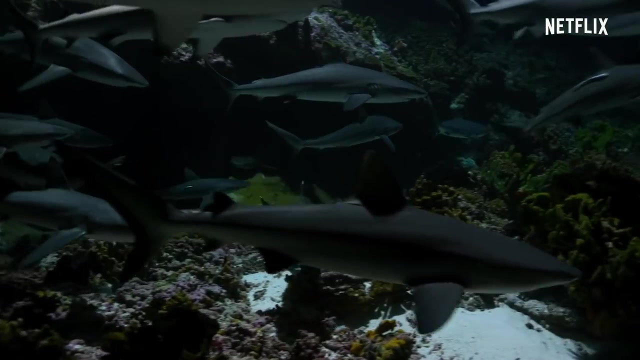 those that are not caught by the white tips are flushed out to the waiting gray reef sharks. with both kinds of sharks hunting in partnership, there is a little respite even within the reef. more and more sharks arrive, attracted by the commotion. such numbers of sharks were once common on reefs around the world, and while so many predators may, 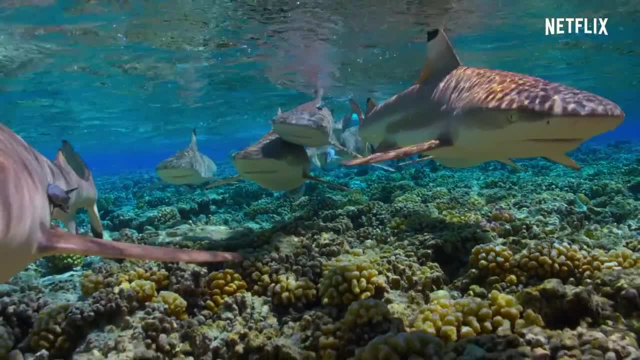 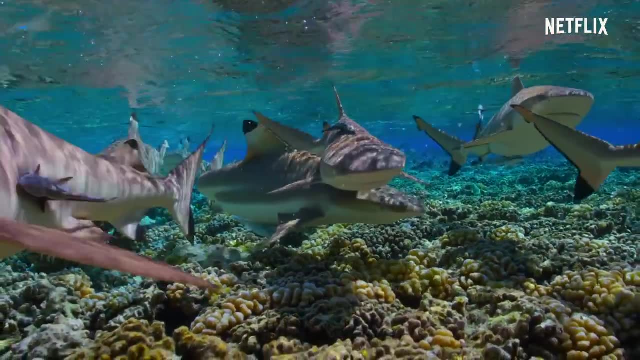 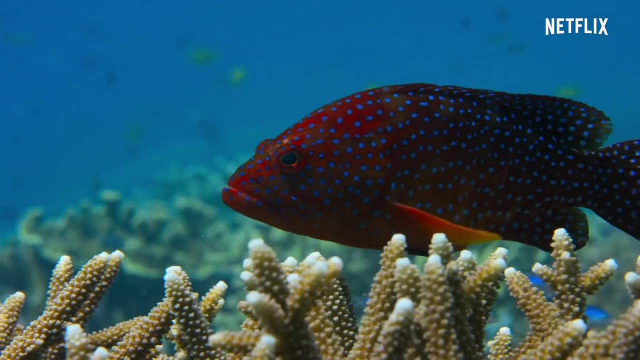 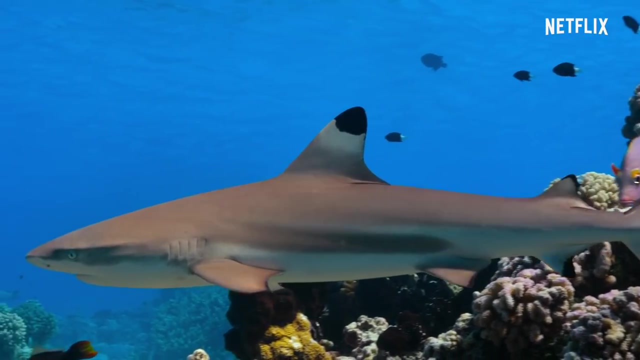 seem damaging. sharks in fact are the most common species of sharks in the world and assist in maintaining the health of the reef. they help to keep a balance in the fish community by hunting the predators that feed on small grazing fish. the grazers in their turn keep the corals free of seaweeds and parasites. 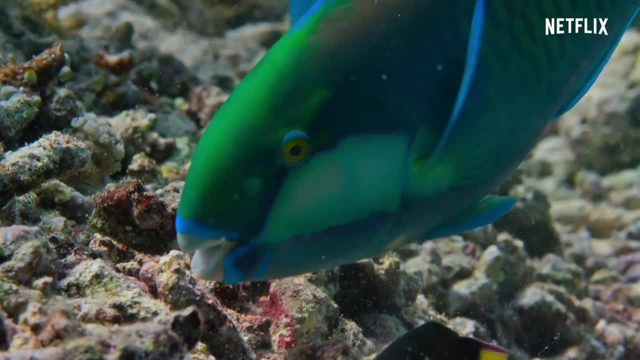 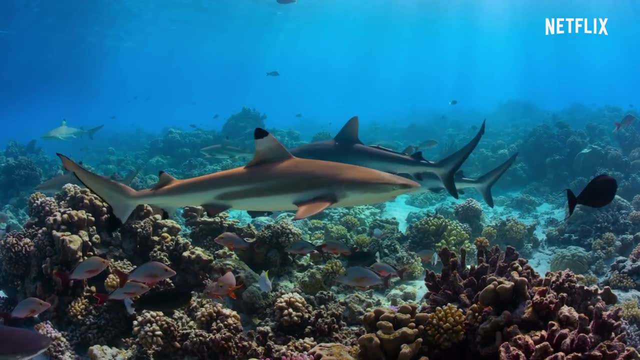 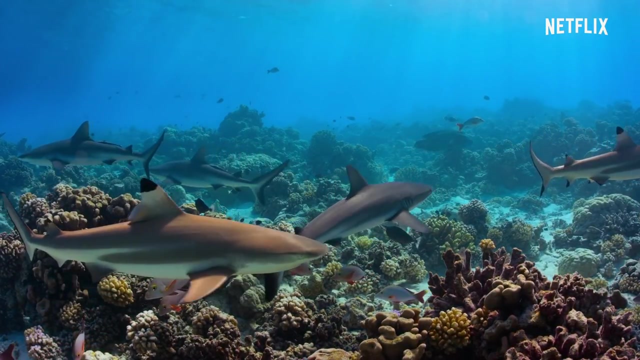 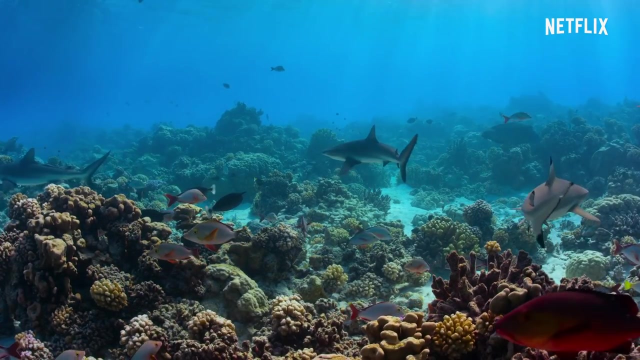 that would otherwise overgrow the reef. a balanced community with sharks as top predators gives a coral reef much greater resilience in the face of damage and disaster. but today even healthy coral reefs are facing a greater threat with climate change: our seas a greater threat with climate change. our seas are�. 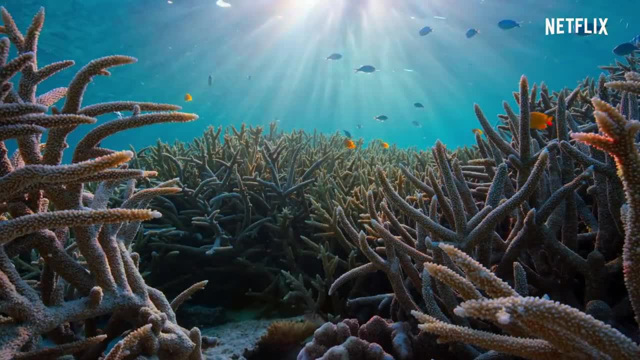 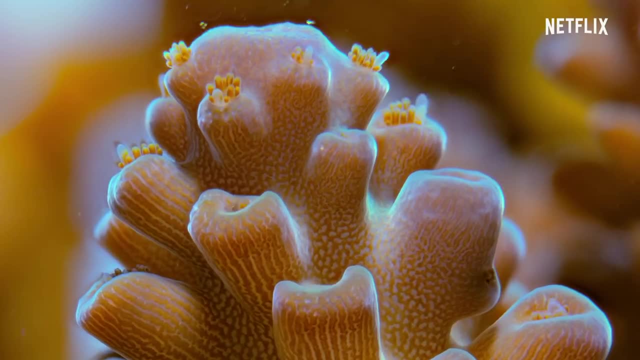 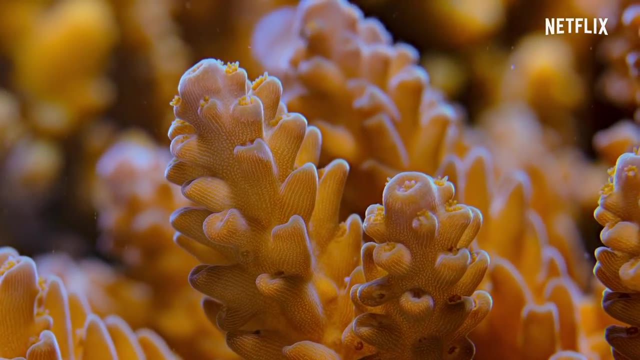 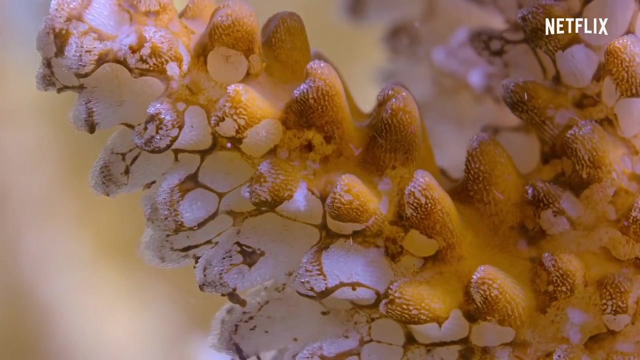 saving our seas are warming. Microscopic plants that live within the tissues of the corals give them both their colour and most of their nourishment. But if sea temperatures rise by just a degree or two, the corals expel their plant partners. 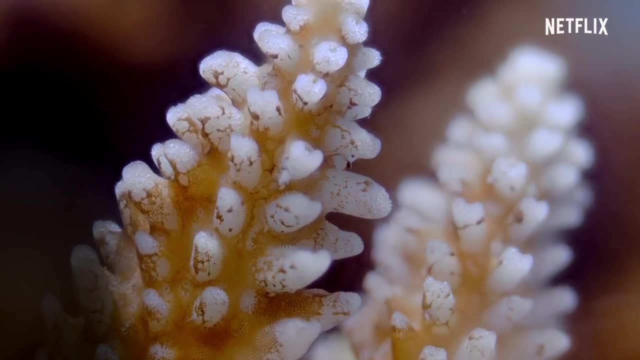 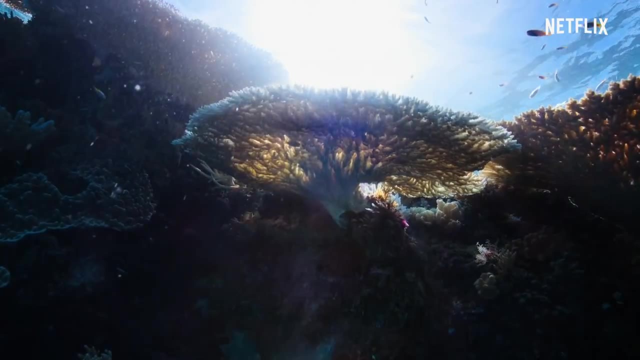 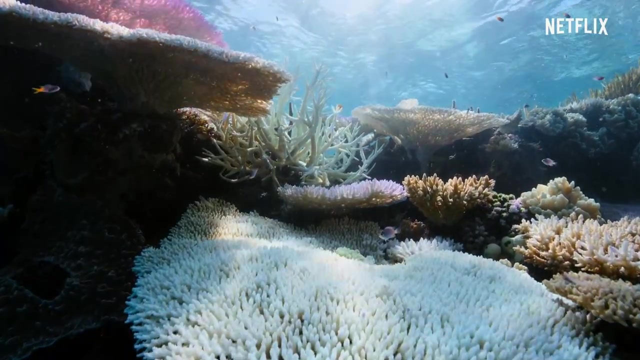 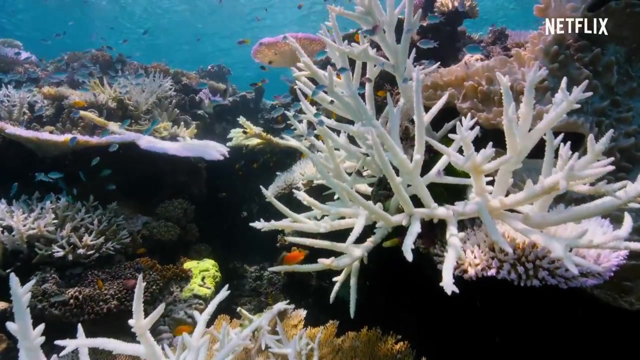 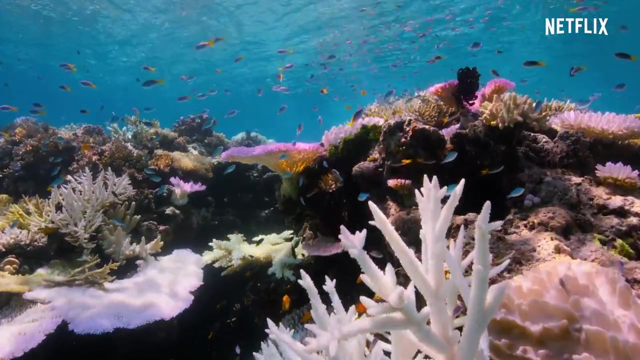 So they lose their main source of food and turn white. Here on Australia's Great Barrier Reef, unusually warm seas have caused many of the reefs to bleach in this way. It may look hauntingly beautiful, but if temperatures remain high for a few weeks, 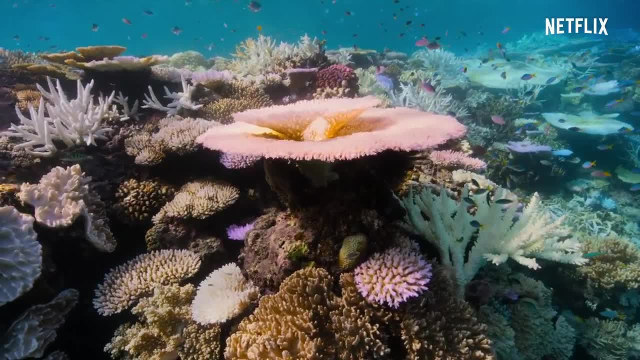 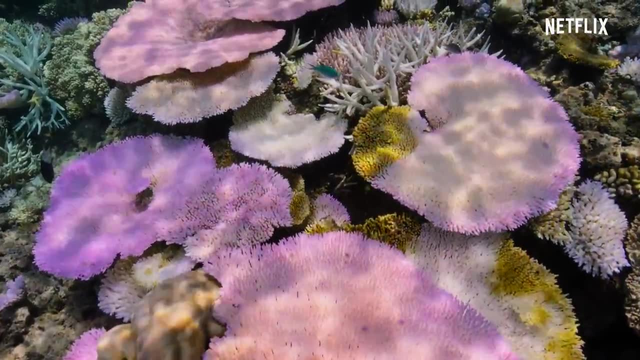 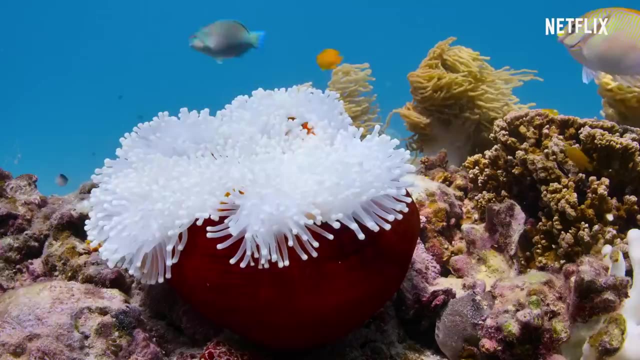 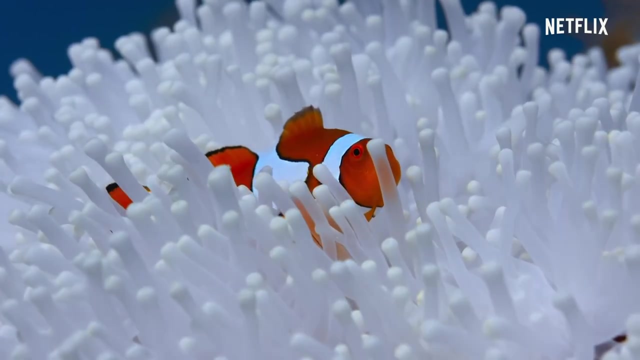 the corals will starve and eventually die. The carbon dioxide that causes global warming is also making the seas more acidic. No reefs can survive both changes And without living corals, many of the reef's residents will also perish During 2016 and 17,. 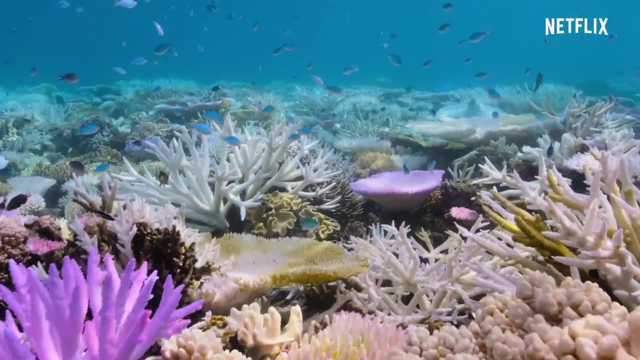 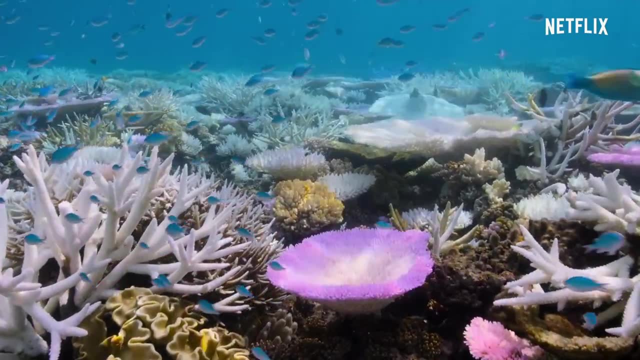 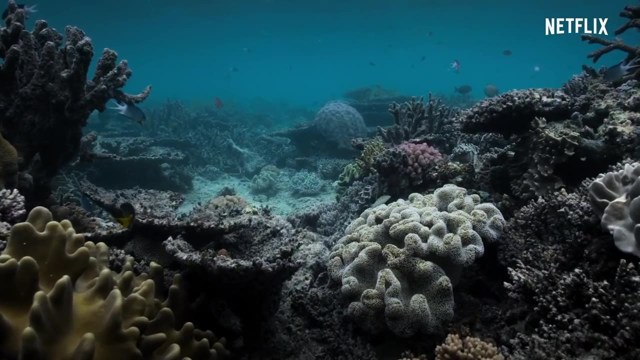 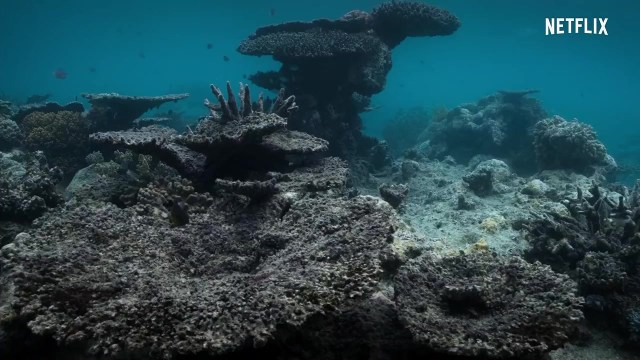 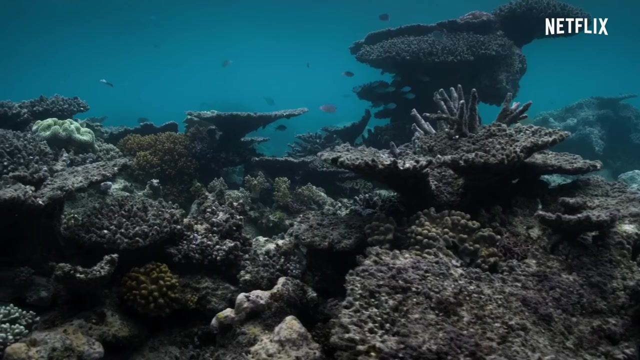 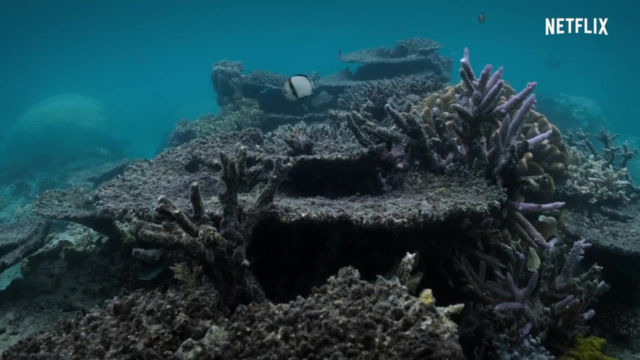 over 1,000 kilometres of the Great Barrier Reef bleached Six months later and many of the corals are dead. The community destroyed. The coral reef was destroyed. The coral reef was destroyed. The coral reef was destroyed Worldwide. half of all shallow coral reefs have already died. 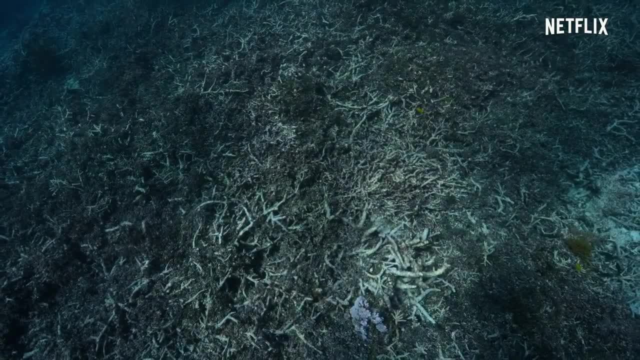 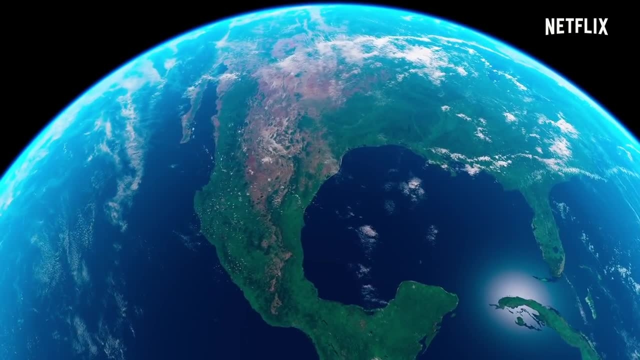 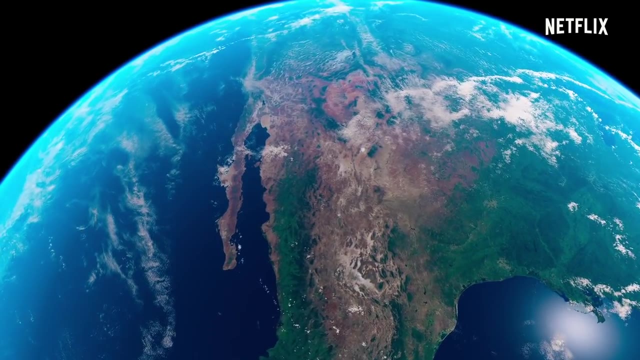 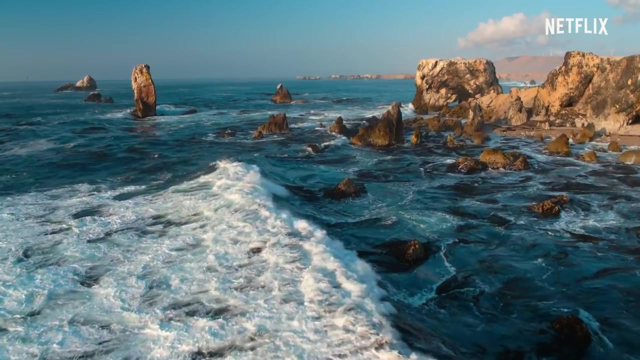 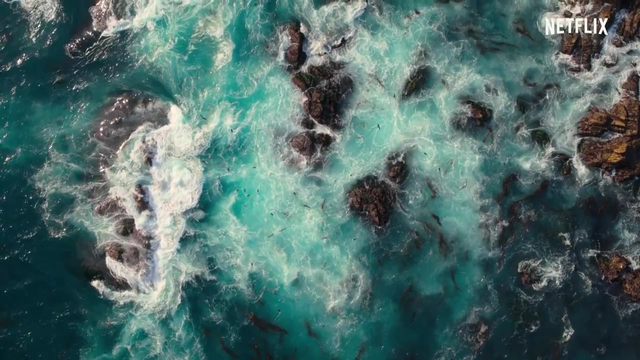 The rest could be gone over the next few decades. away from the tropics, in higher latitudes, the seas are much cooler. storm lashed waters bring essential nutrients to the surface. the enriched water combined with long summer days make these the most productive seas on the planet. 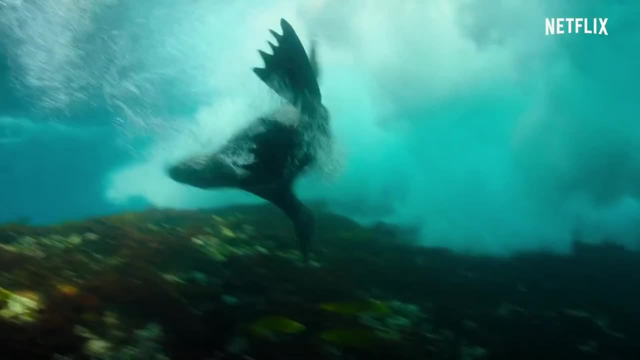 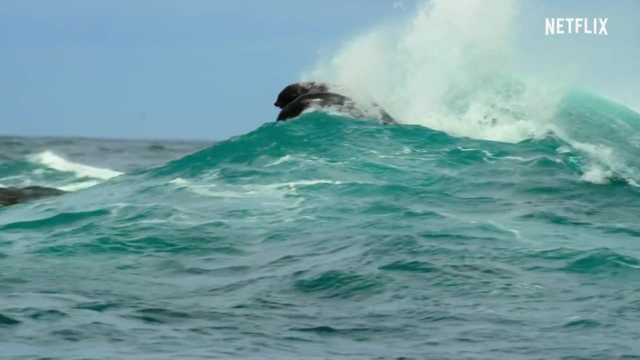 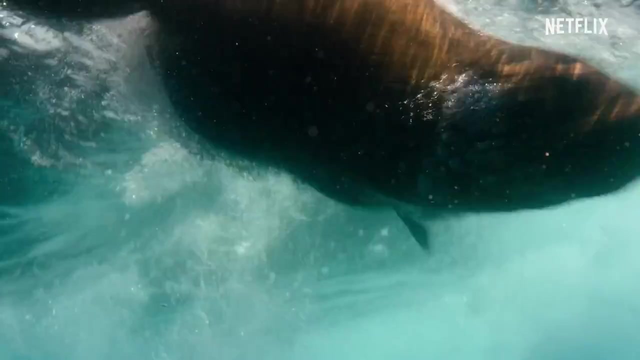 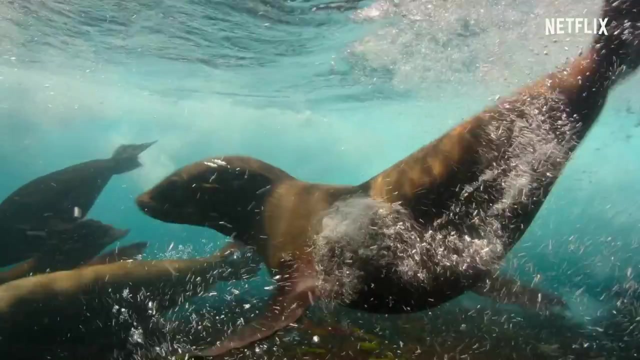 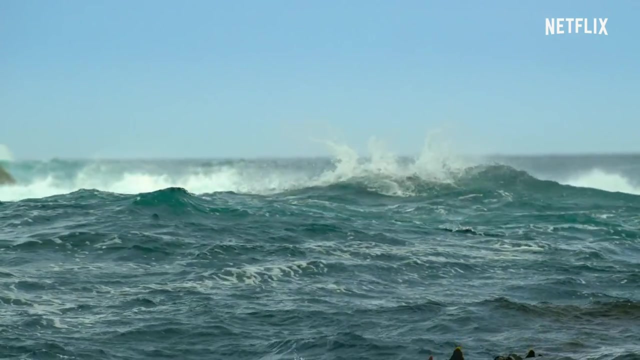 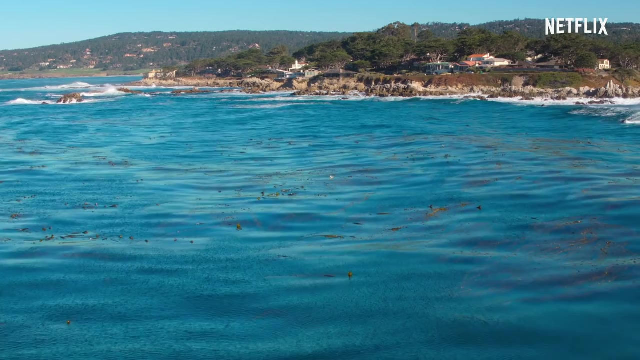 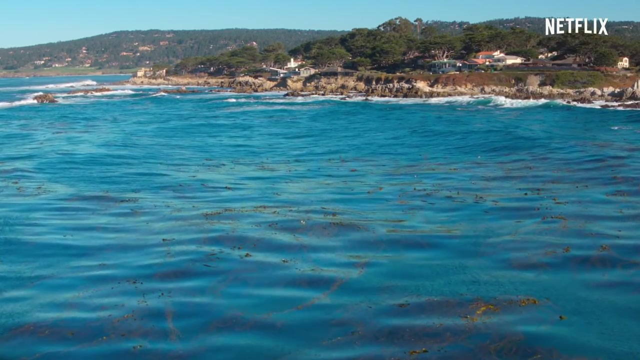 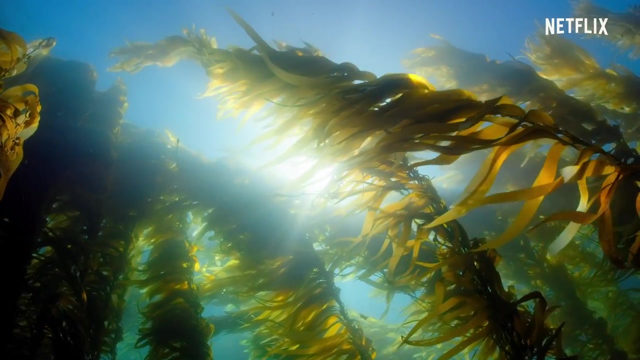 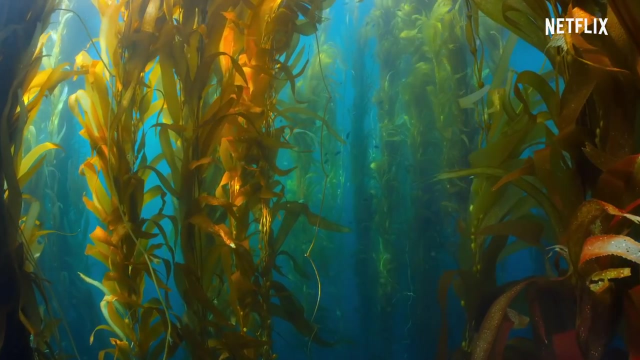 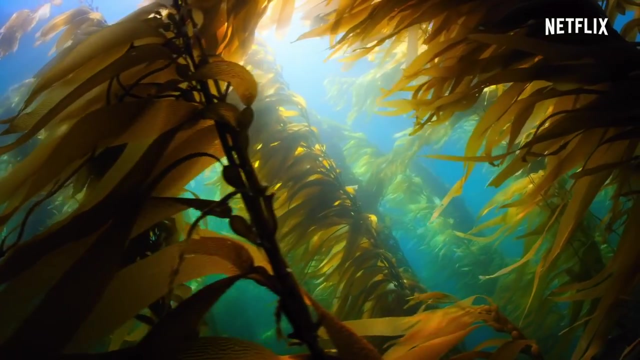 fur seals thrive and even have time to ride. the waves spring off the coast of california and fronds of golden kelp floating on the surface hint at the riches hidden beneath a magnificent submarine forest. these stands of giant kelp are as important to the oceans as trees are to. 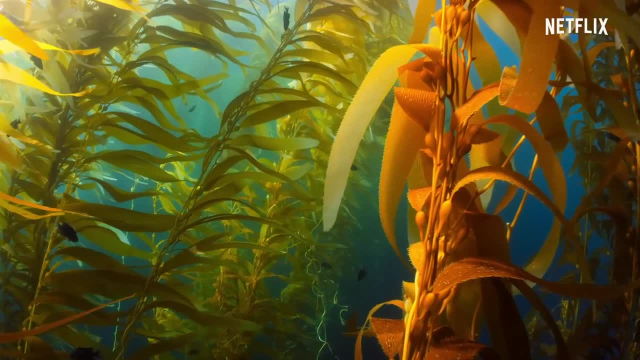 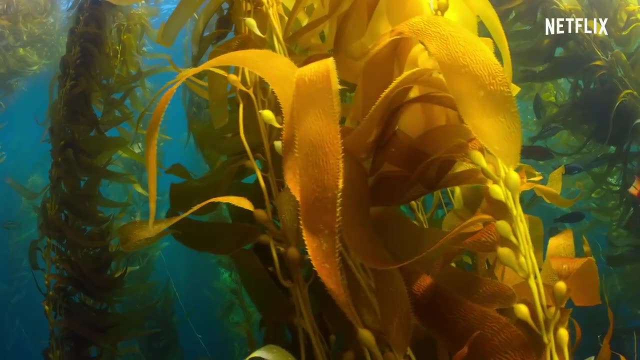 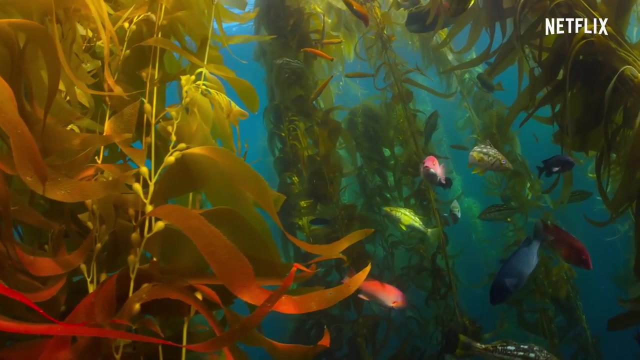 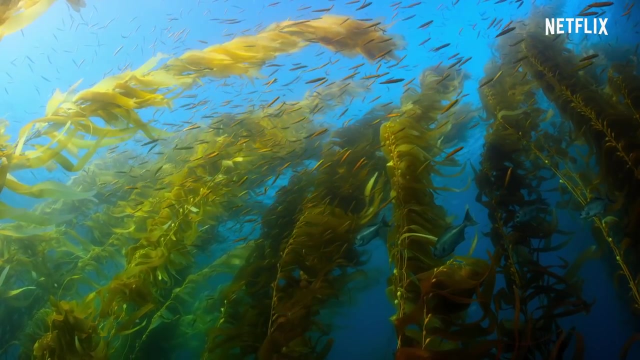 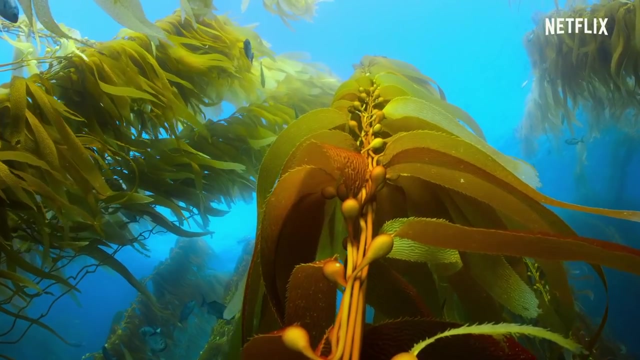 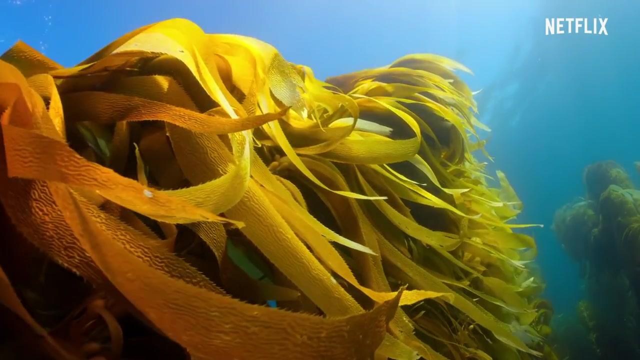 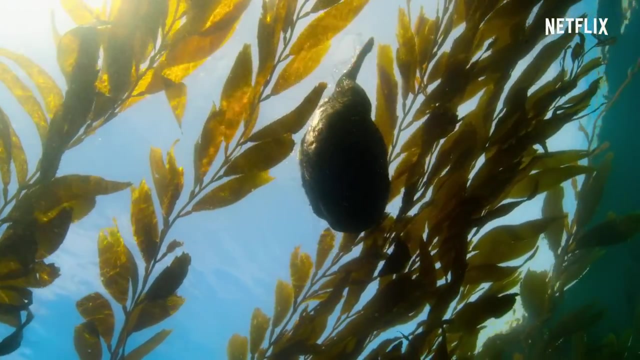 the land like a rainforest. the dense canopy provides food and shelter for an abundant community. in the cool, rich seas, giant kelp can grow 50 meters high. airfield floats lift the from towards the Sun. that surface, nestling in this canopy, A sea otter. 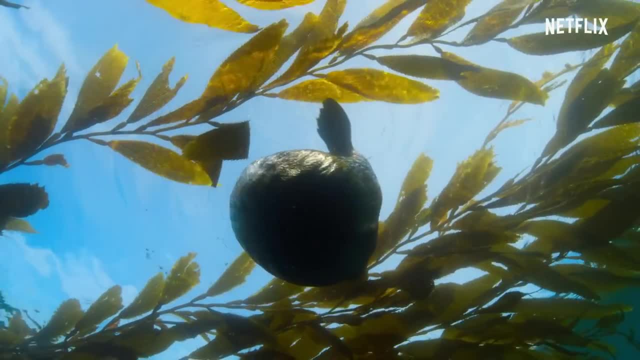 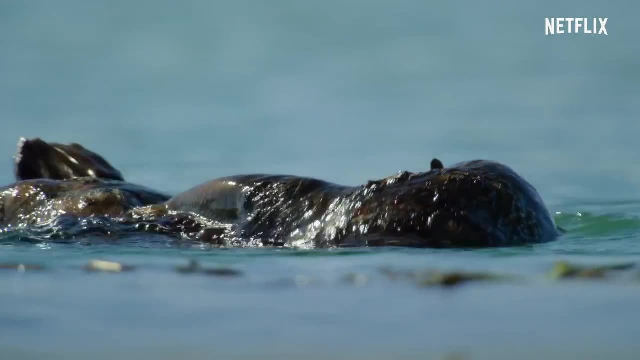 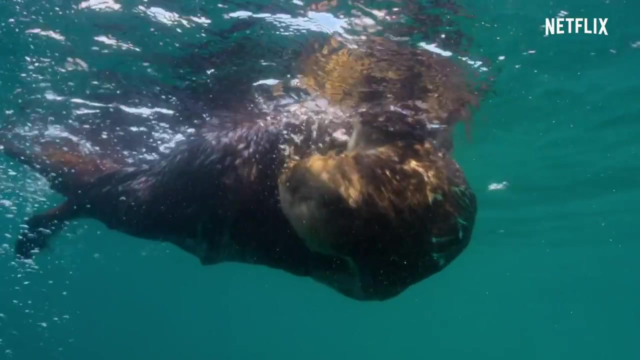 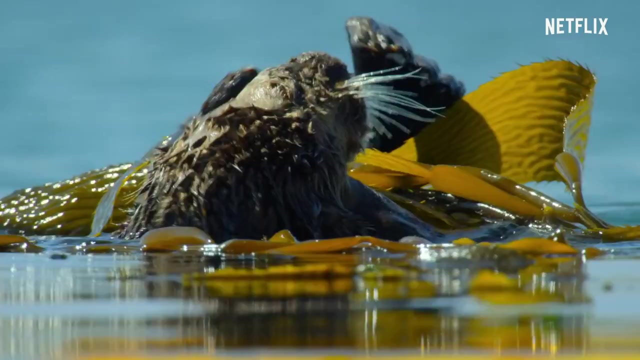 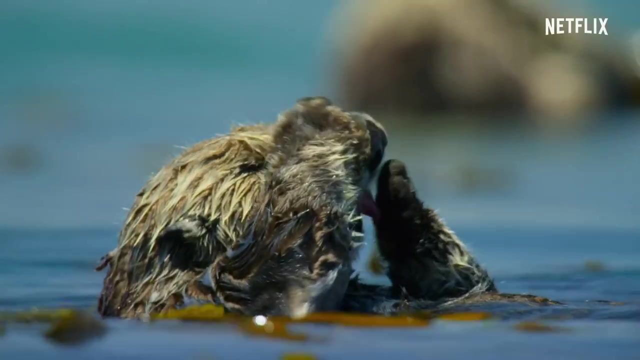 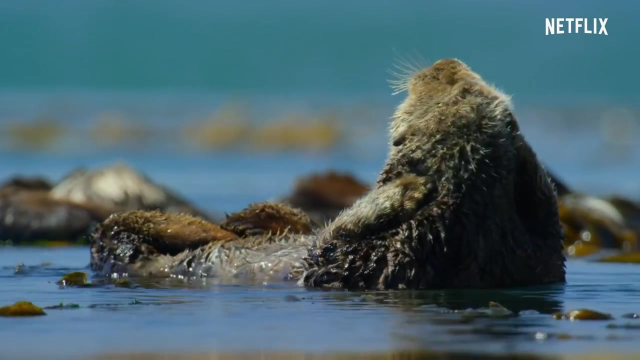 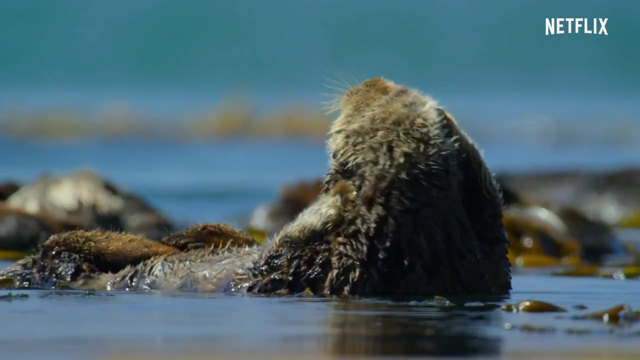 His thick fur keeps him warm in the chilly water. Blowing air into it gives him extra insulation. Sea otters have the densest fur of any animal And such a luxuriant coat requires a great deal of attention. They need to eat a lot to keep warm. 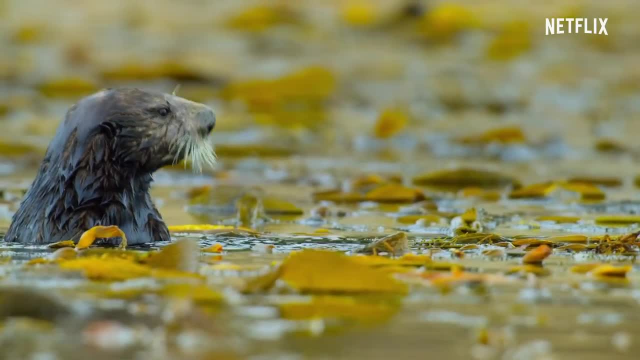 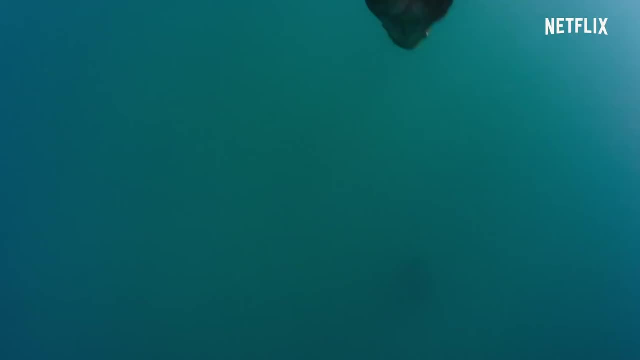 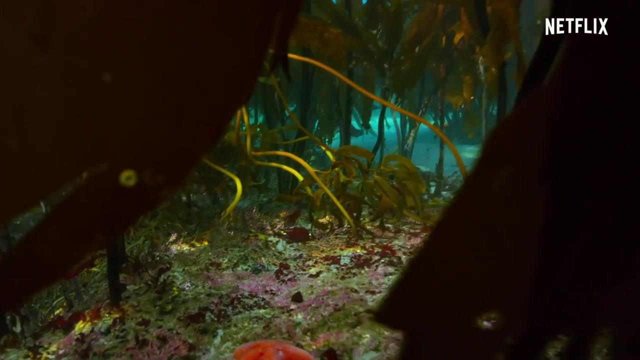 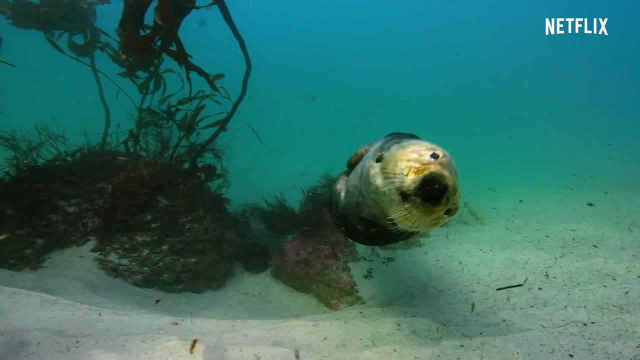 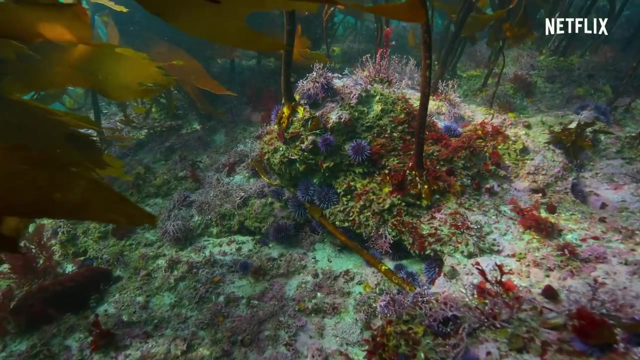 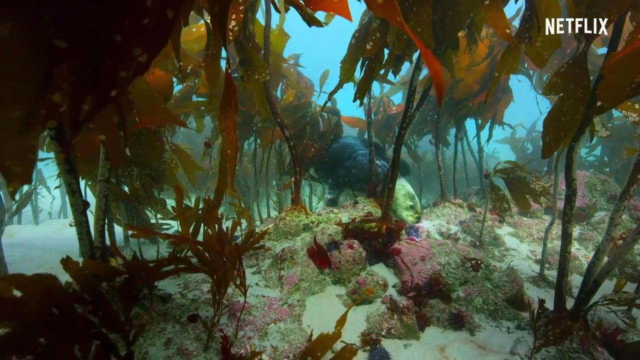 and consume up to a quarter of their body weight every day. They need to eat a lot to keep warm and consume up to a quarter of their body weight every day. Sea urchins are a favourite food. There's one And a second. 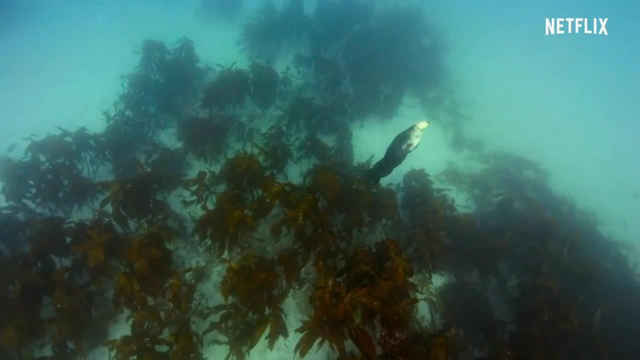 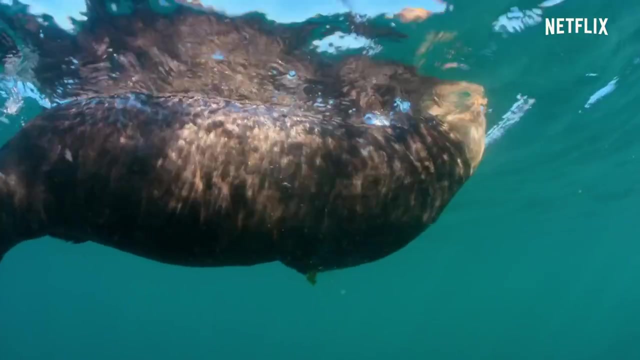 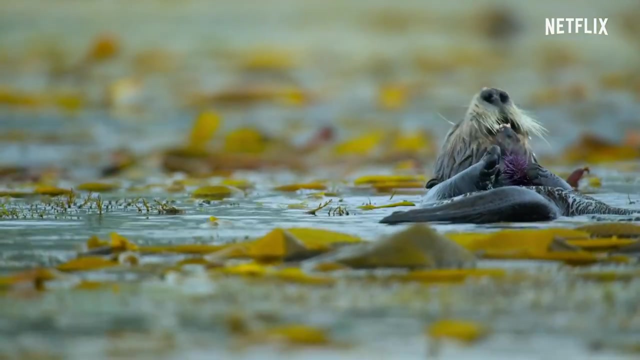 And then the otter is out of breath and must return to the surface. And then the otter is out of breath and must return to the surface. An urchin looks like a rather prickly meal, but if you can break the shell, there's a feast inside. 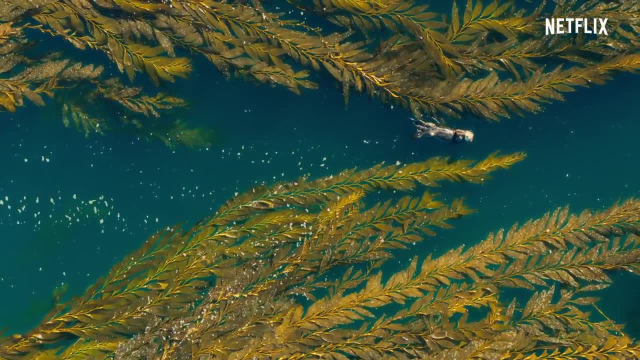 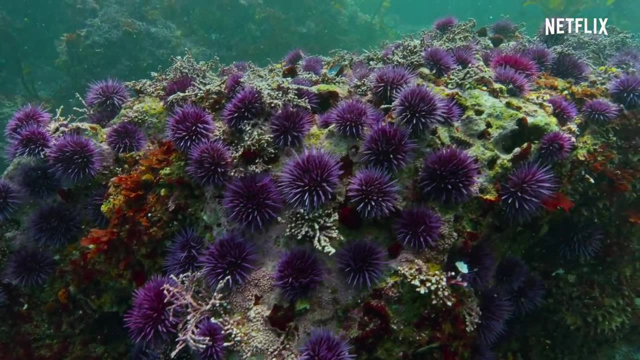 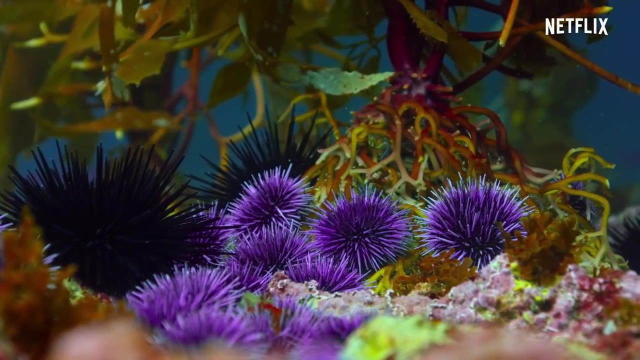 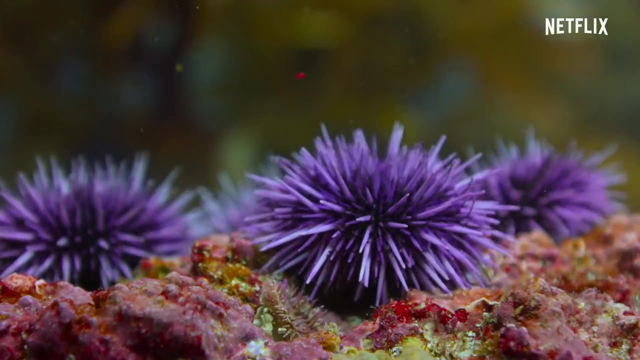 Sea otters are crucial to the health of the kelp forest because they keep down the number of sea urchins. Sea otters are crucial to the health of the kelp forest because they keep down the number of sea urchins. The urchins graze on kelp. 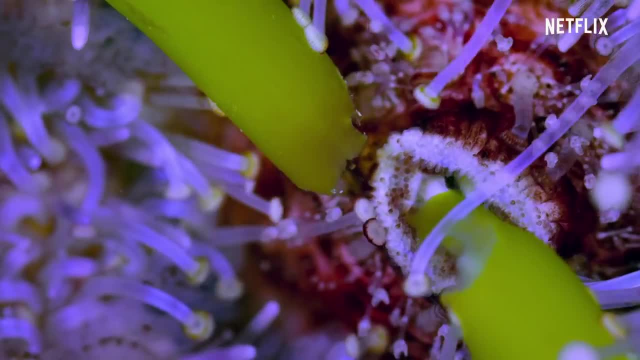 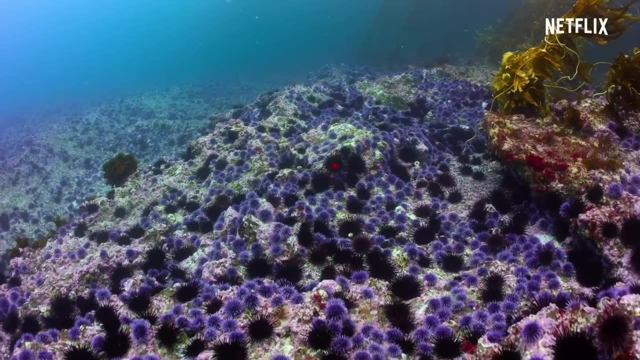 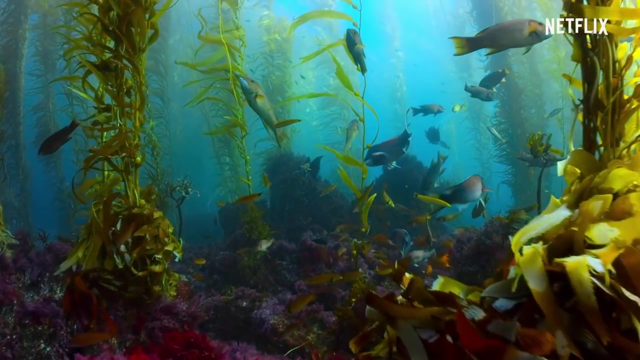 munching through their tough stems. Left unchecked, they spread across the seafloor like a plague. Left unchecked, they spread across the seafloor like a plague. Fortunately, the otters have a helper in the fight against these spiny grazers. 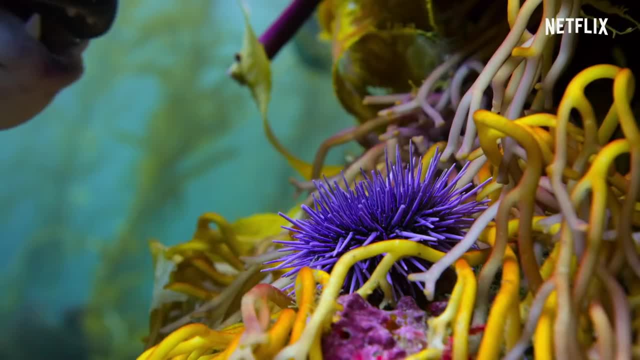 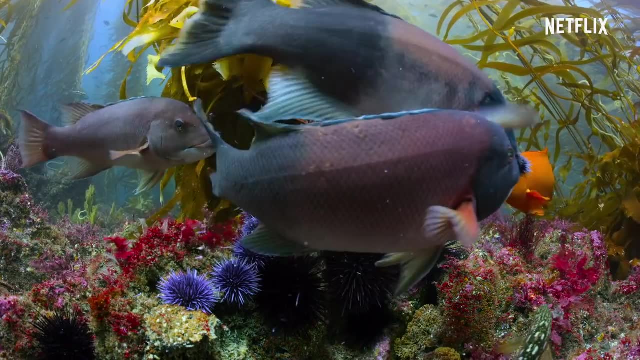 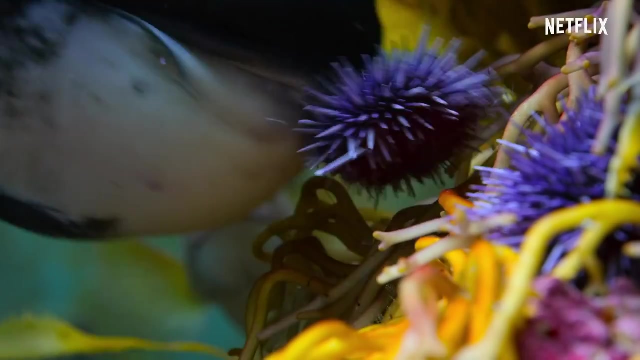 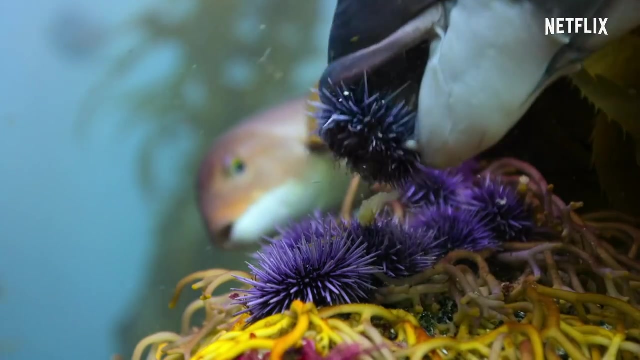 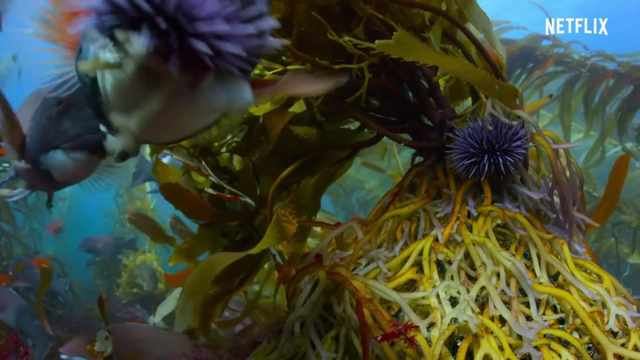 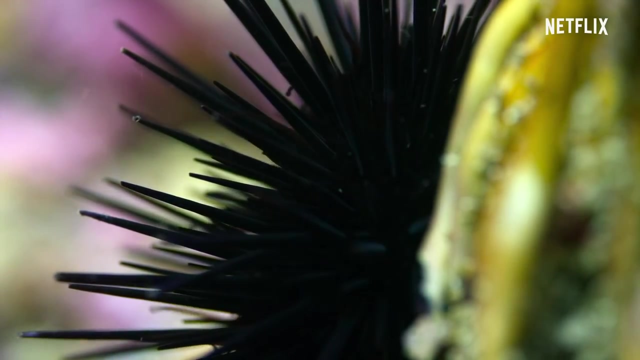 Sheephead wrasse. They have powerful teeth and can make short work of the smaller purple urchins and can make short work of the smaller purple urchins. The larger black urchins, The larger black urchins- a challenge especially for smaller wrasse. 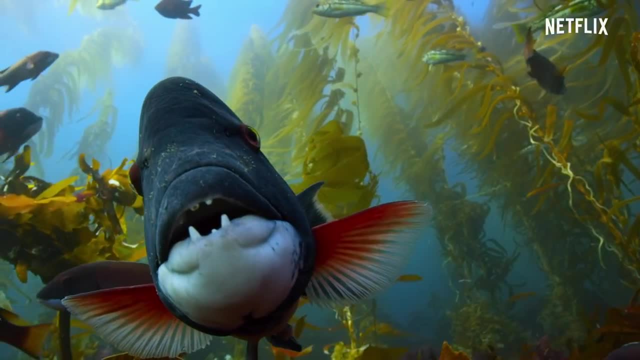 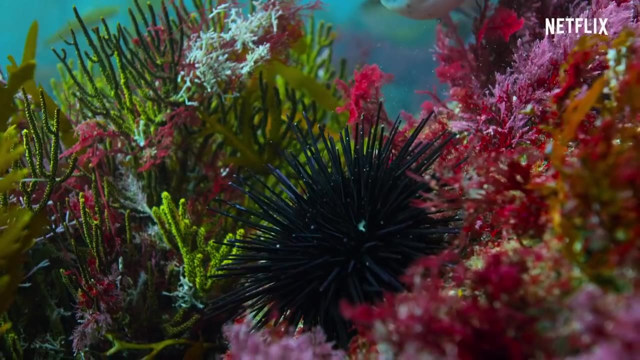 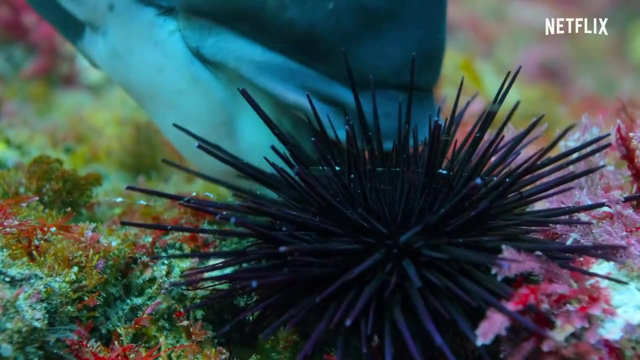 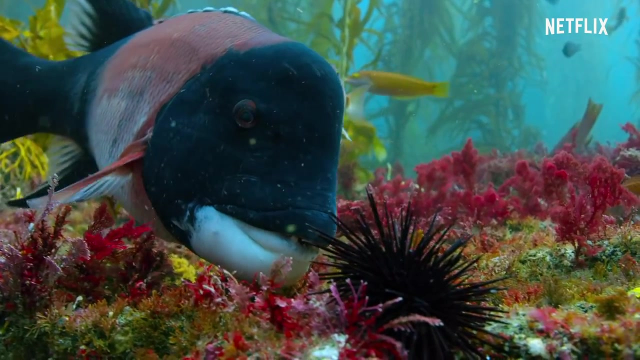 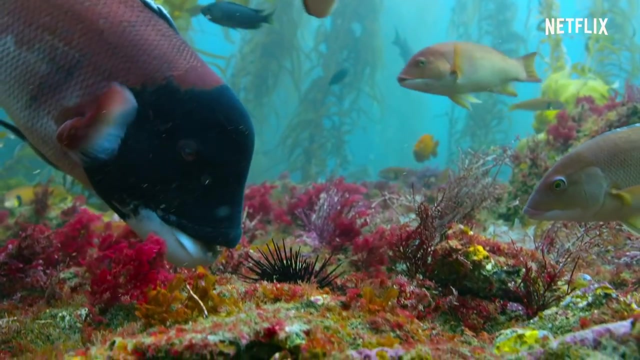 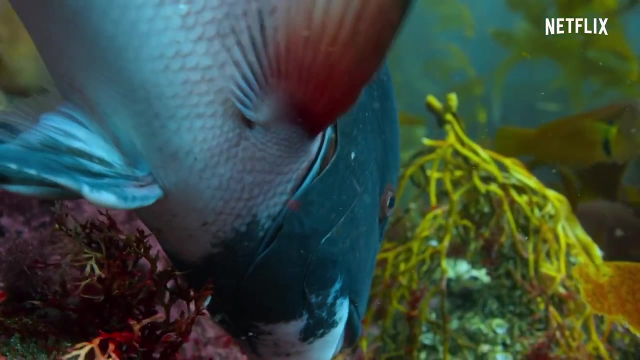 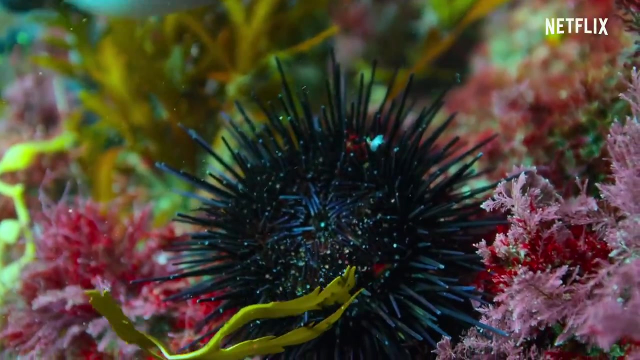 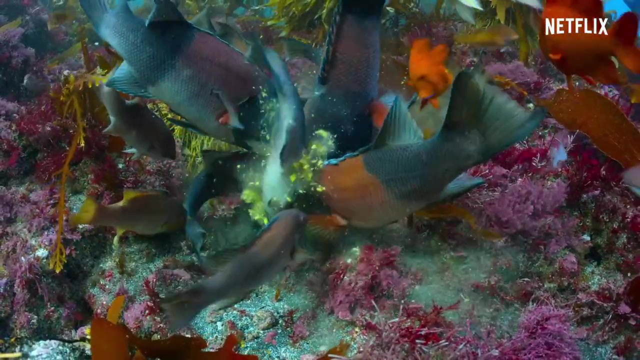 Only the very largest sheephead can tackle them. But it still has to get past those long spines. The urchin has to be flipped over to expose its vulnerable underside. Not easy when you have no hands. Success at last, And everybody benefits. 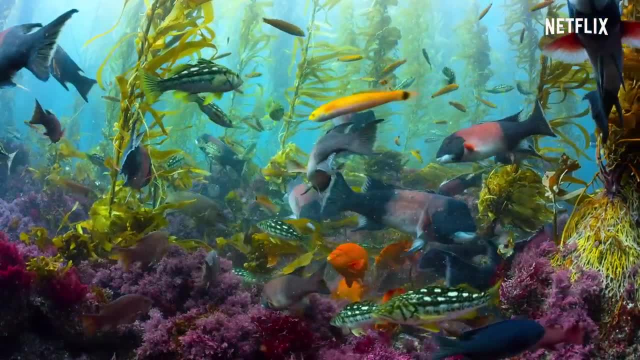 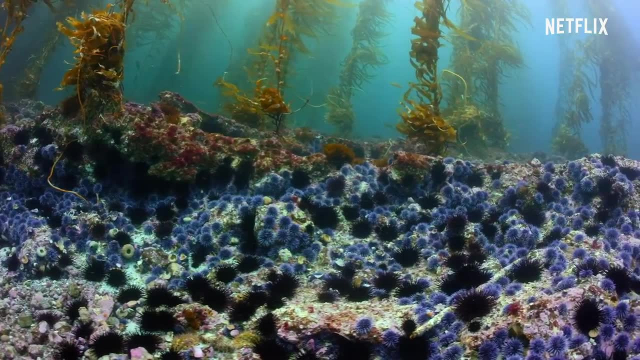 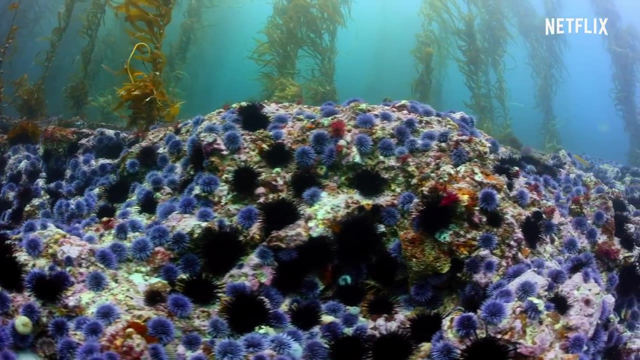 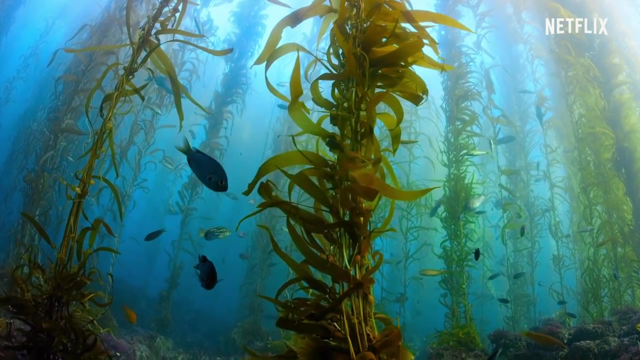 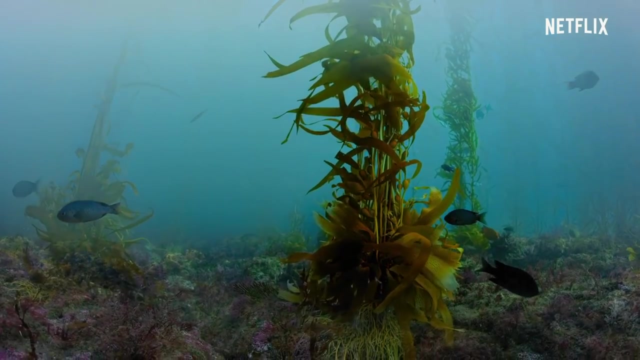 These fish and otters living within marine protected areas keep the kelp grazers under control, But giant otters just outside these sanctuaries, the urchins graze unchecked and fell the kelp forest, All those that depend on the kelp. 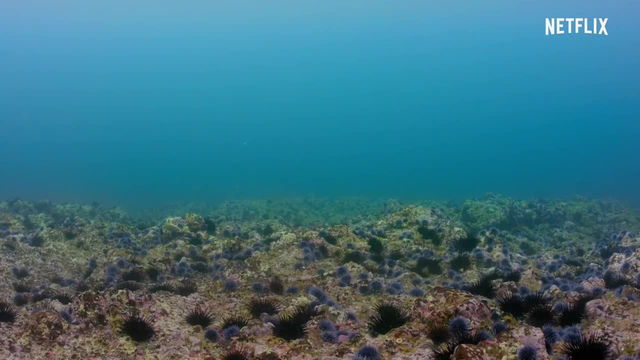 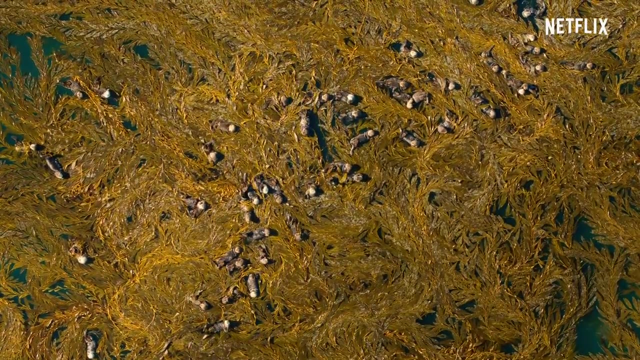 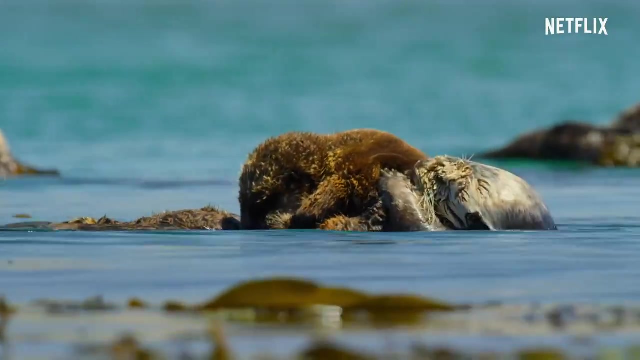 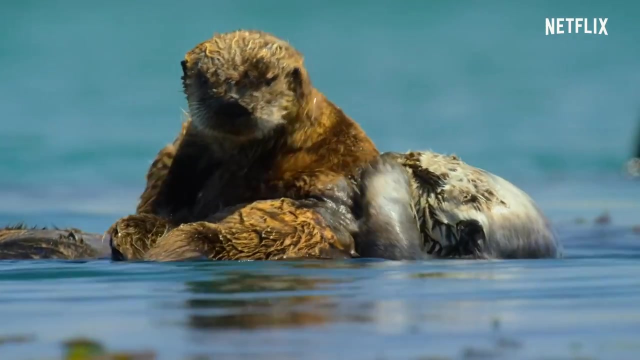 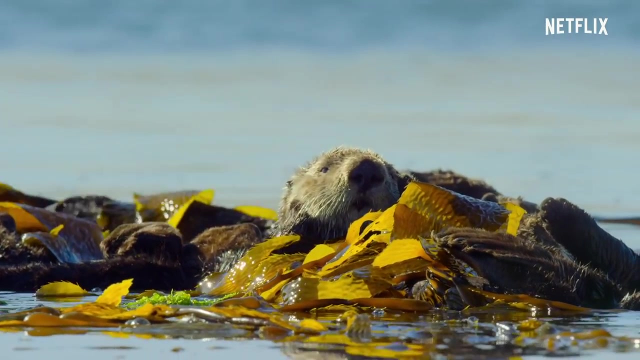 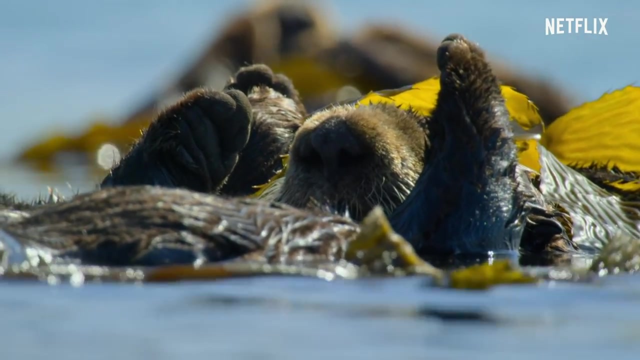 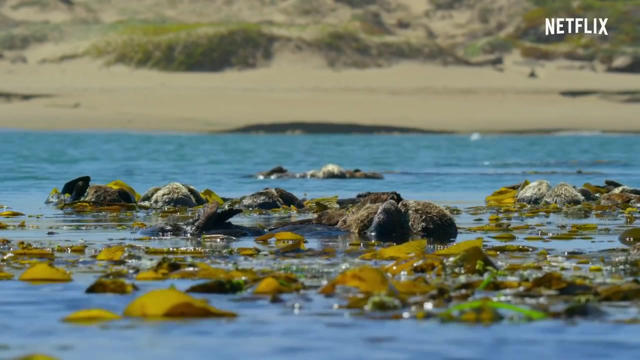 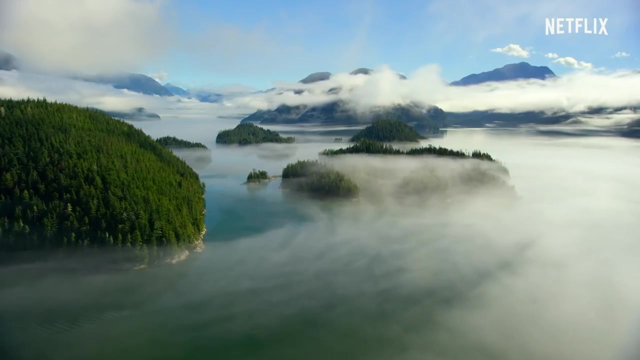 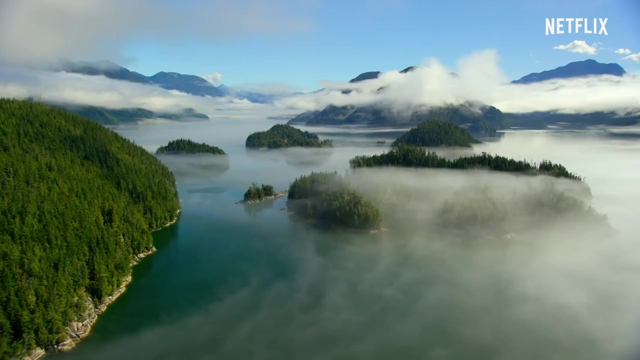 have disappeared. In California, kelp forests grow abundantly in protected areas where the whole marine community can live without pressure from people. Here at least sea otters can chill out- Californian style- The 3,000 kilometers further north in Alaska. 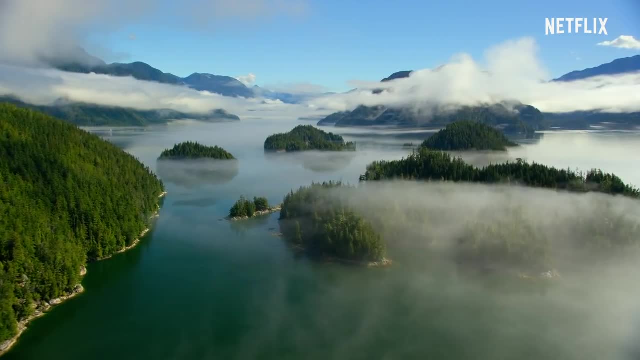 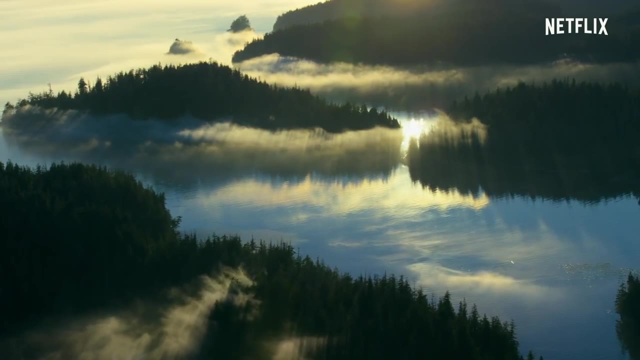 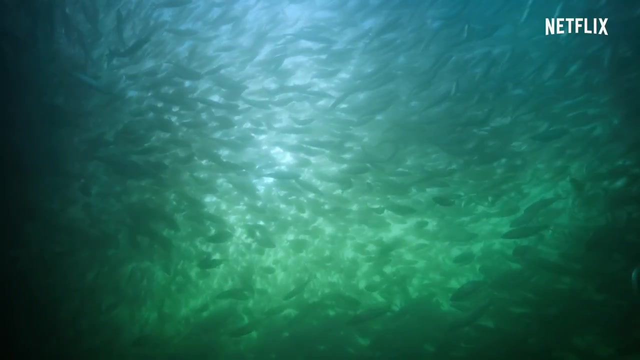 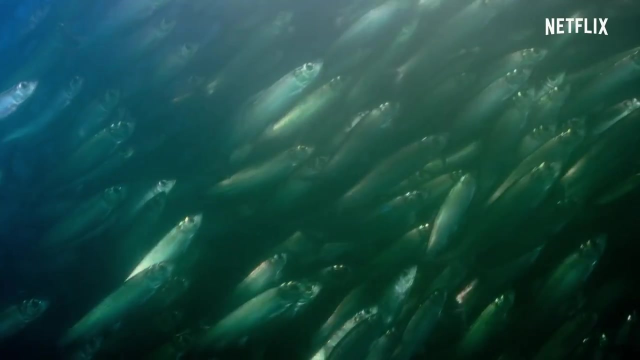 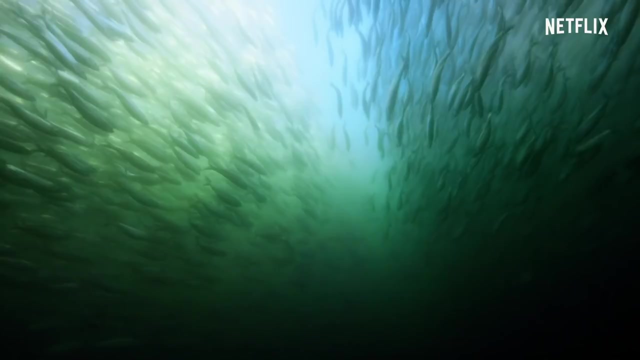 spring arrives much later in the year, After a cold, hard winter. the first rays of the sun trigger a great annual event: Immense shoals of herring rise up from the depths and move into shallower waters. They're gathering to breed. 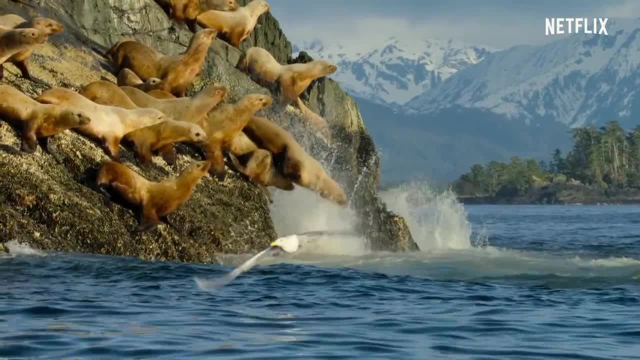 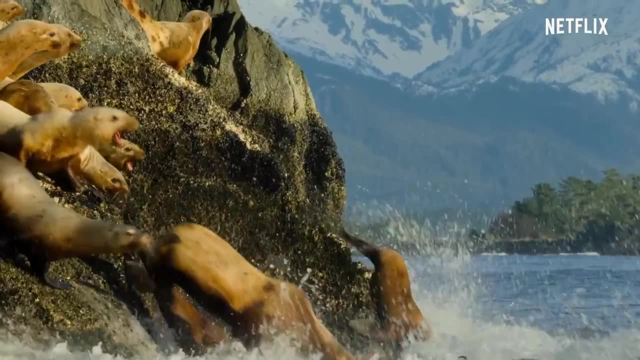 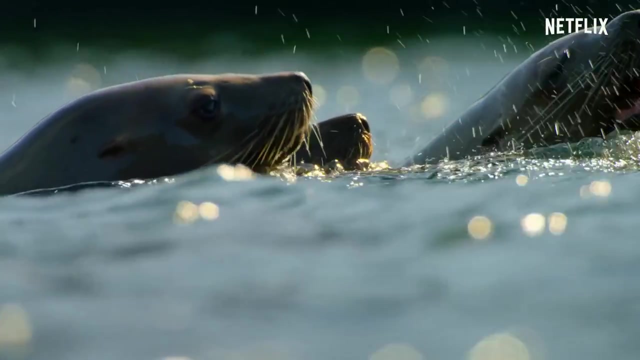 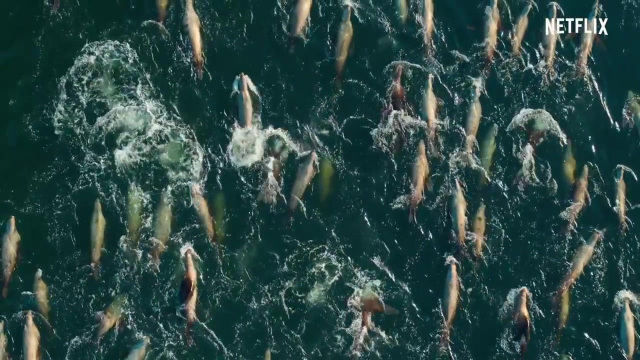 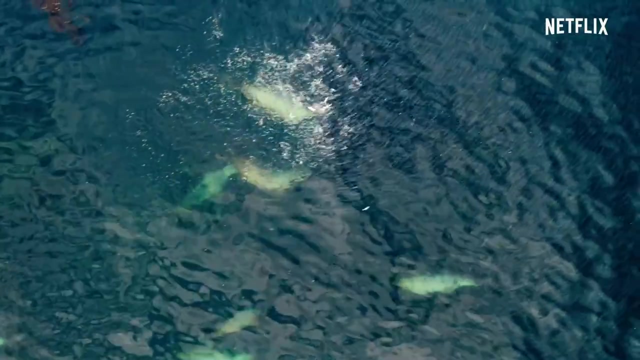 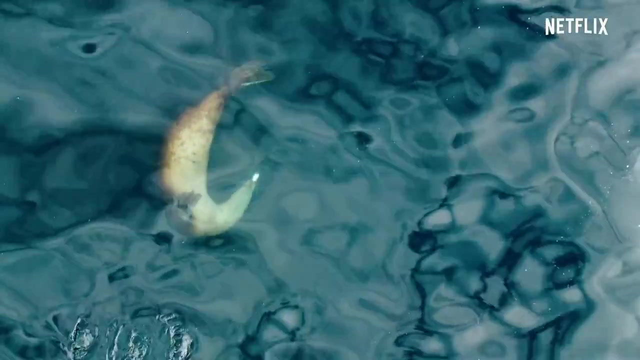 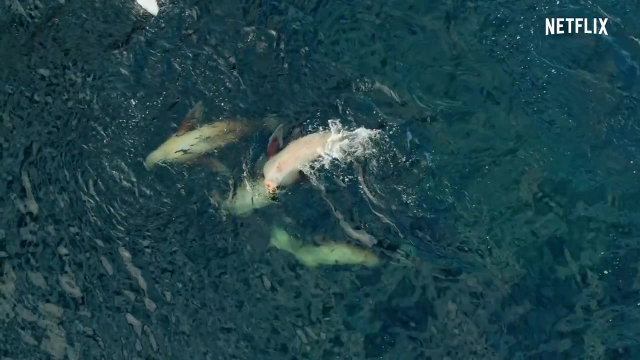 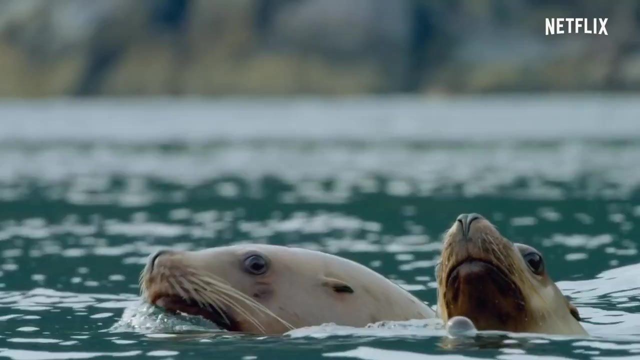 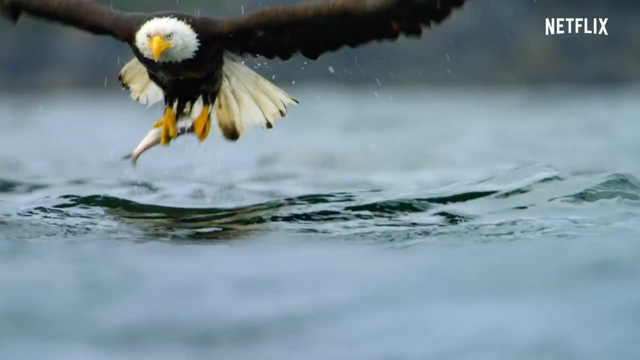 But predators are waiting for them. Stellar's sea lions, So intent on their mission, the herring make easy prey. Sea lions drive the fish to the surface within range of aerial hunters. Bald eagles: normally solitary birds. 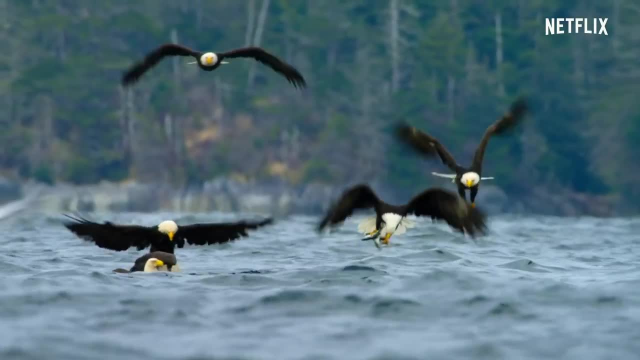 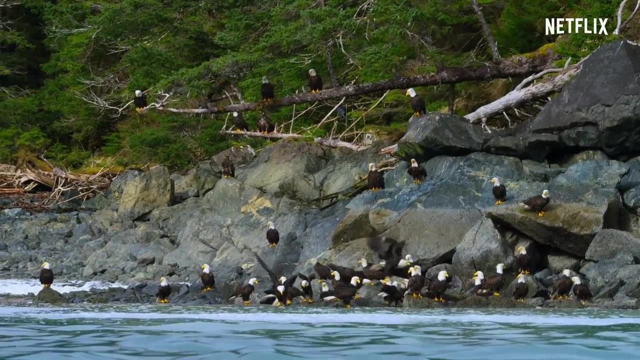 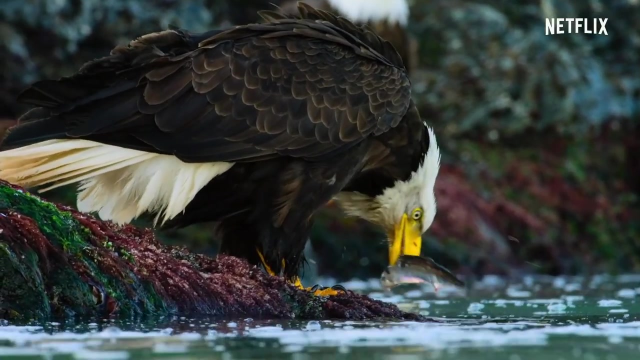 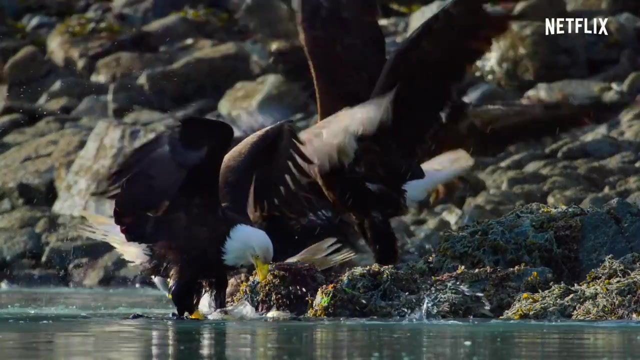 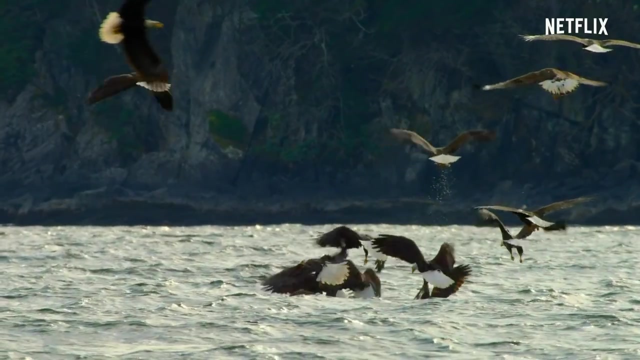 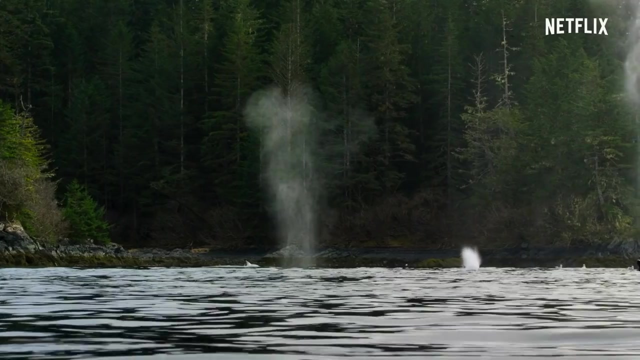 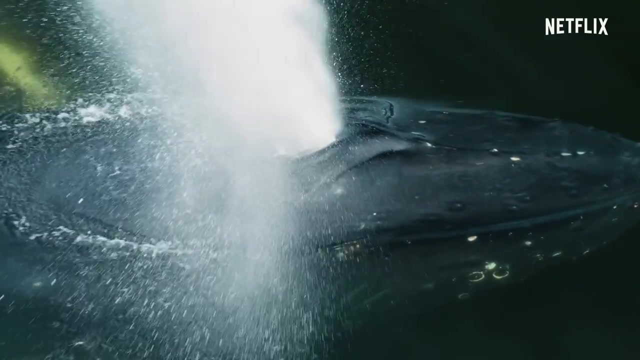 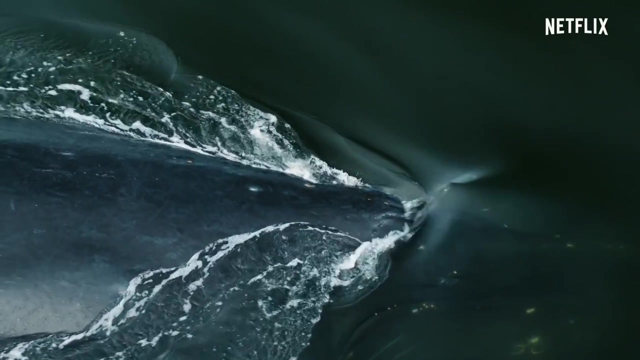 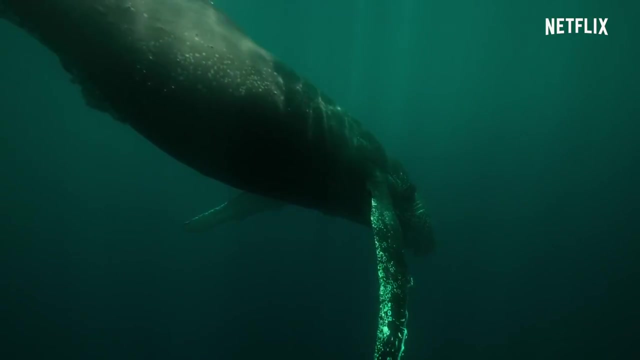 have assembled in numbers for the feast. In places, the herrings reach shore and there the eagles don't even need to take to the air Humpback whales. They have come all the way from the tropics hoping to get their first meal in months. 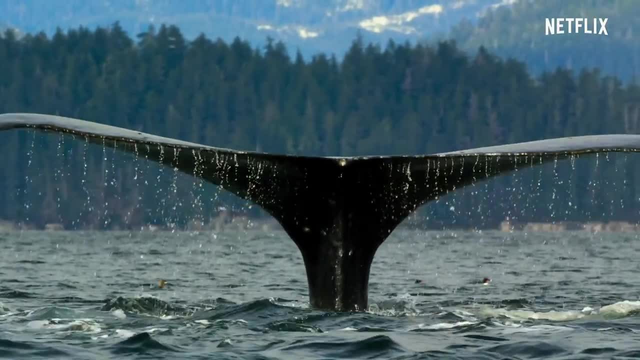 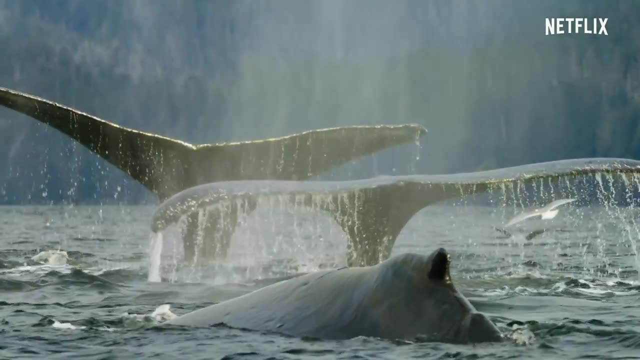 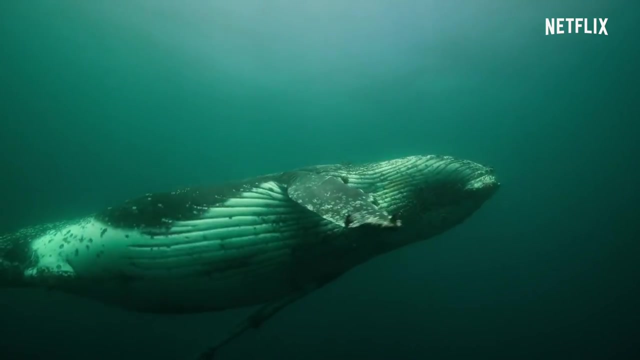 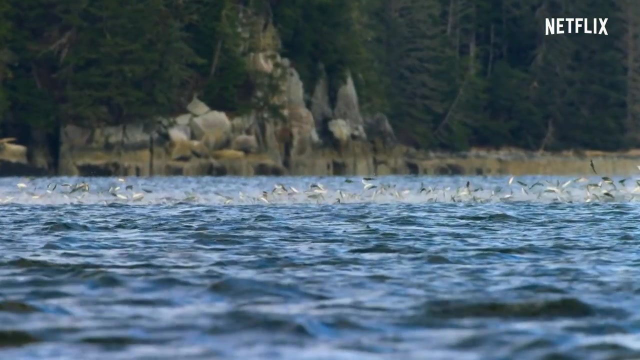 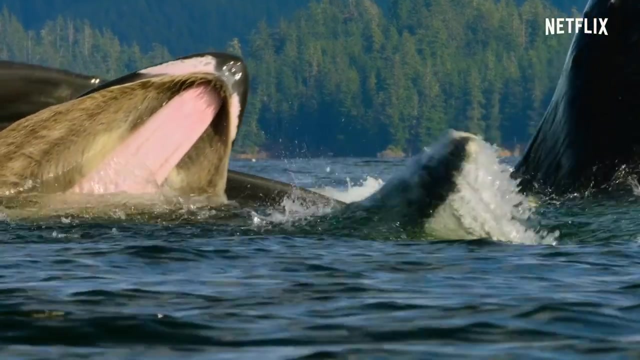 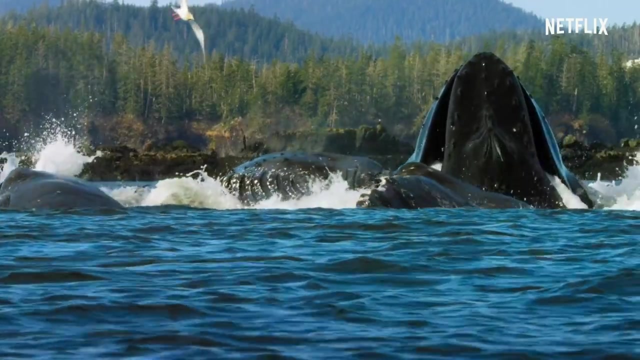 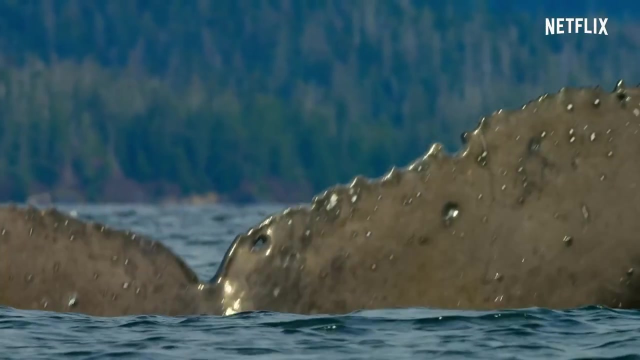 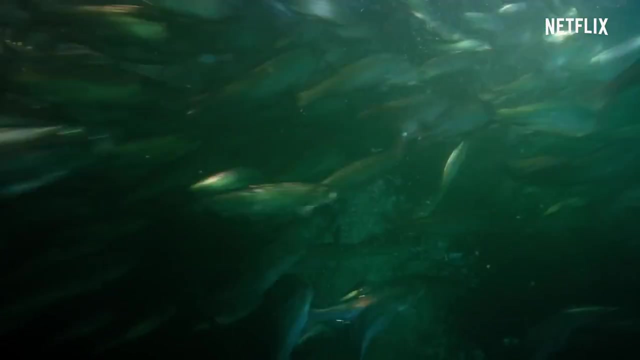 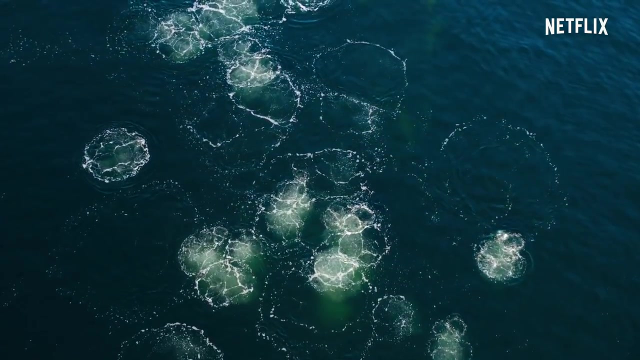 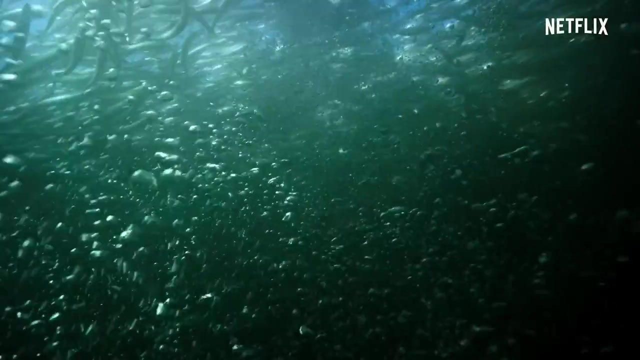 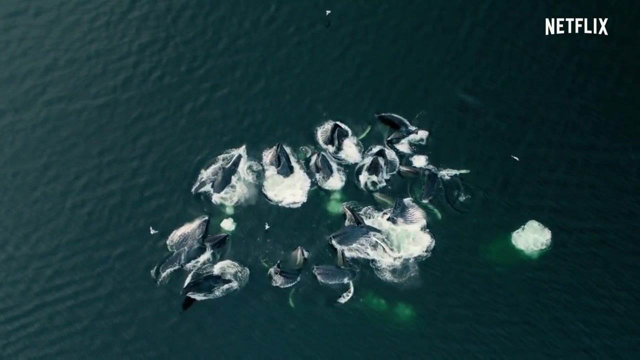 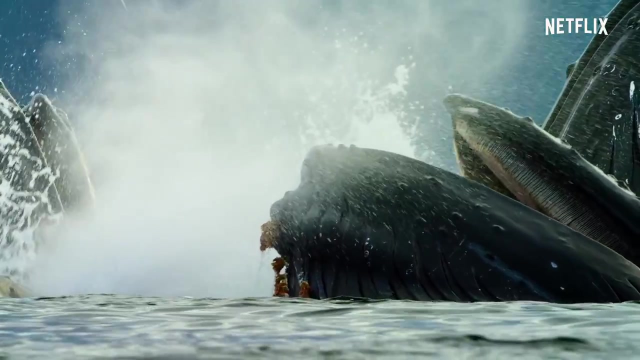 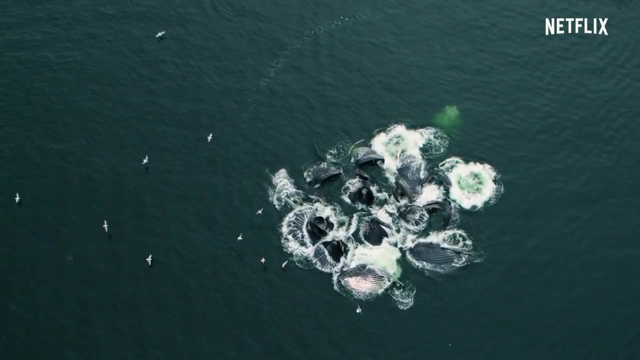 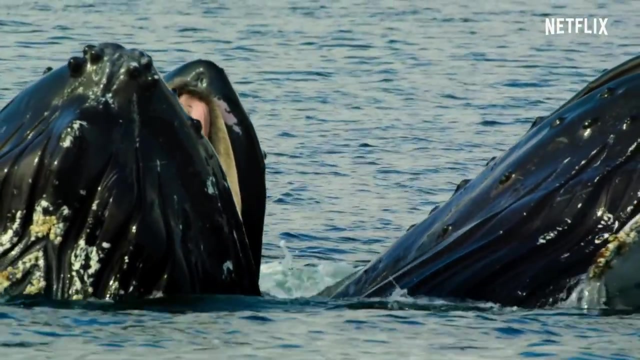 These whales have a remarkable way of collecting this seasonal bounty. They work as a team. The lead whale dives first and blows a curtain of bubbles to concentrate the fish. A call synchronizes the attack. Humpback whales are also superhuman. 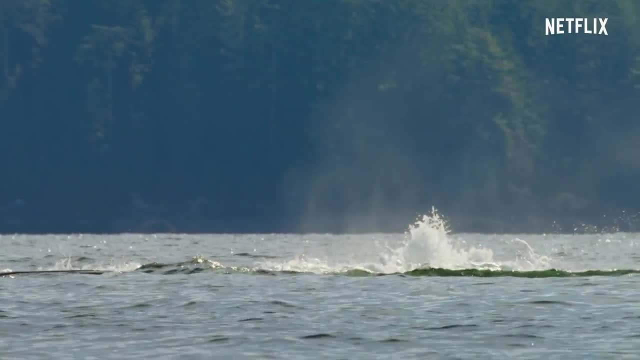 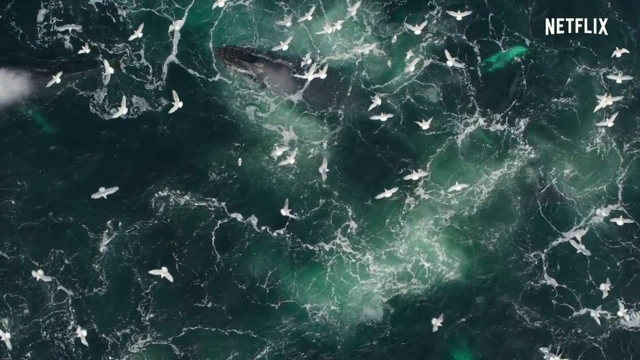 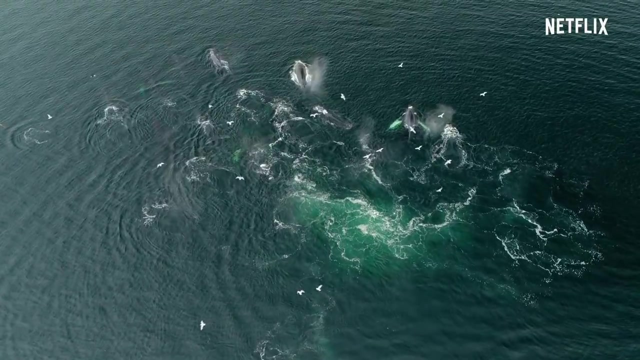 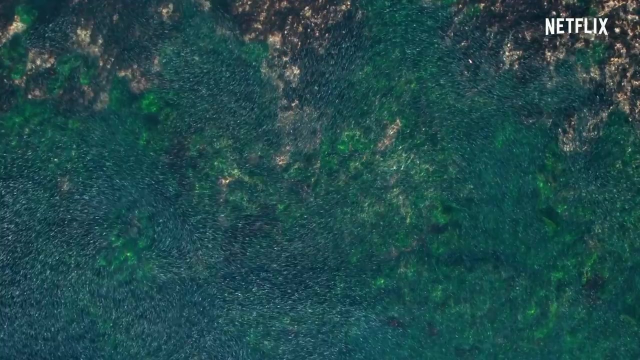 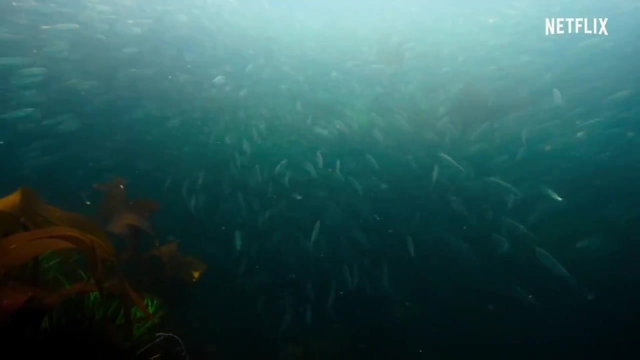 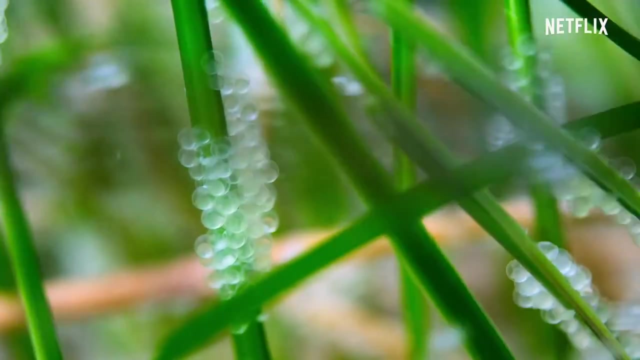 Their. By cooperating in this way, each whale can eat a ton of fish a day, Yet the herring are so abundant that, in spite of the whales most manage to reach the shallows And here they spawn, The females lay their eggs on the sea grass. 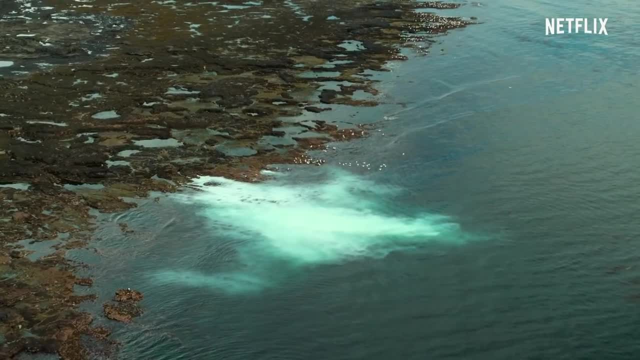 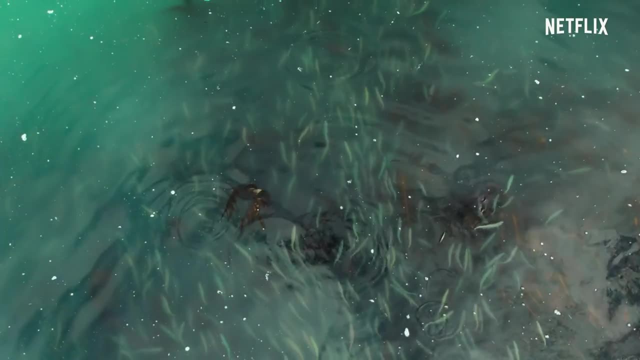 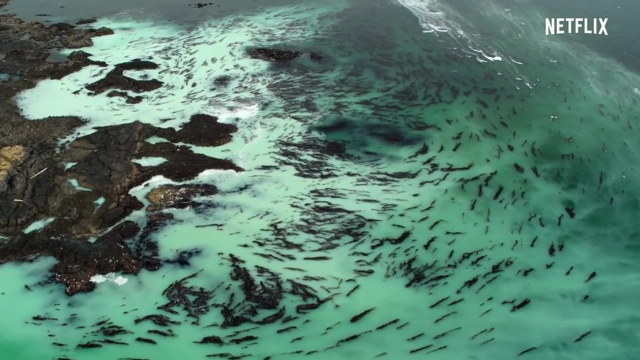 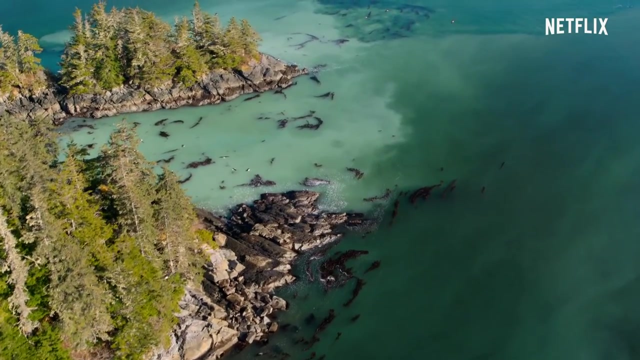 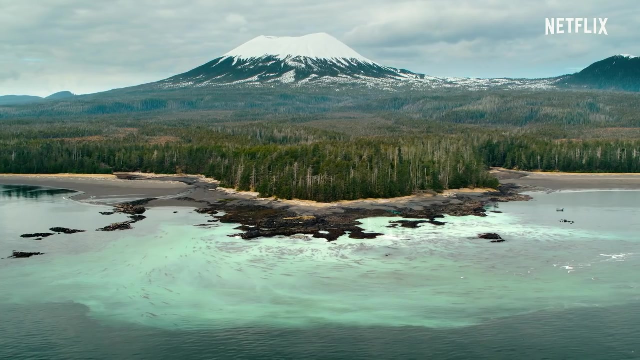 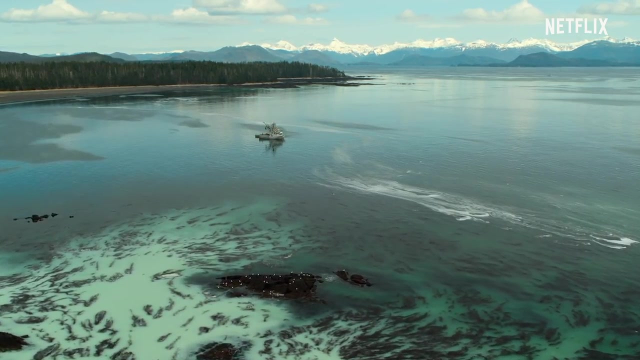 The males follow, fertilizing the eggs with clouds of sperm. Once, herring thrived here in an abundance we can barely imagine today. They used to turn shorelines white, with spawn right across the North Pacific, from Japan to California, With industrialized fishing techniques. 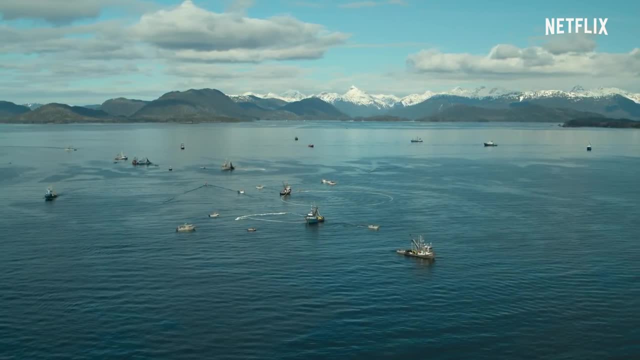 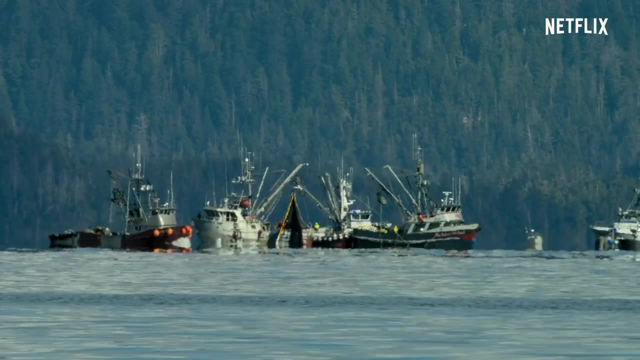 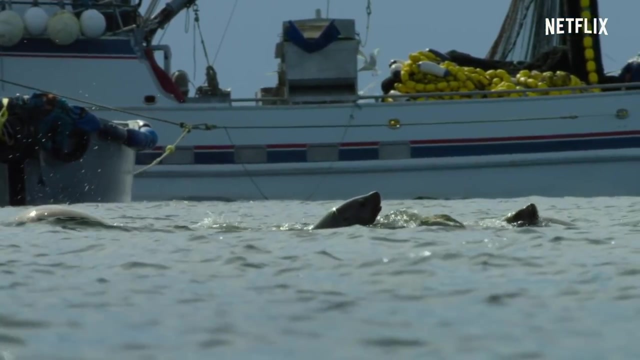 it's all too easy to over-exploit these breeding stocks. This is one of the few places where a fishery still survives. It's the only place in the world where herring can be found in the Pacific Ocean. And it's the only place in the world where herring can be found in the Pacific Ocean. 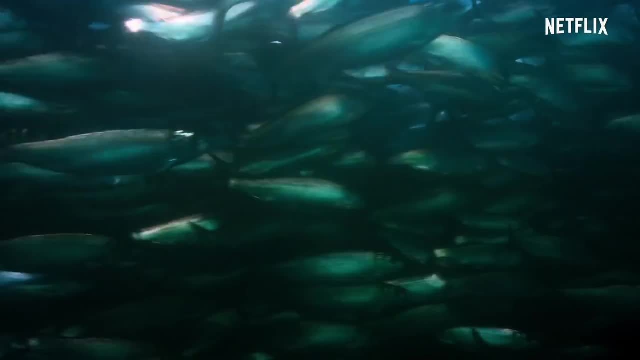 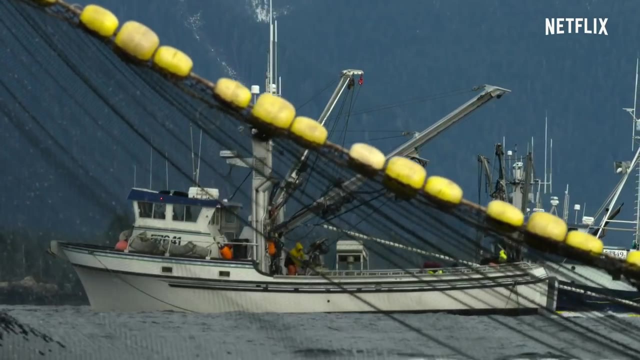 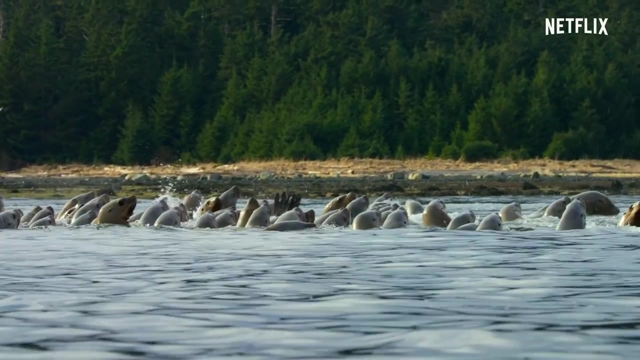 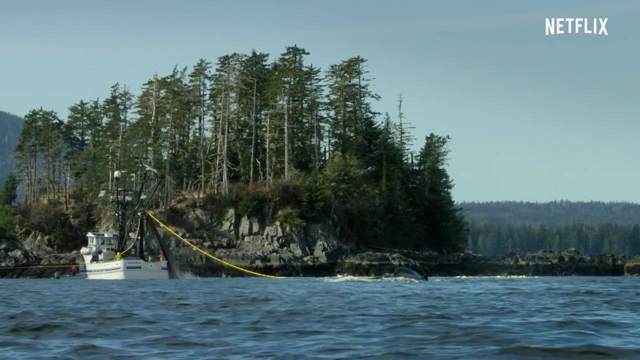 It's the only place in the world where herring can be found in the Pacific Ocean. Pacific herring populations are greatly reduced- a mere fraction of what they once were. This sorry tale of unsustainable fishing has been repeated time and again around the world. 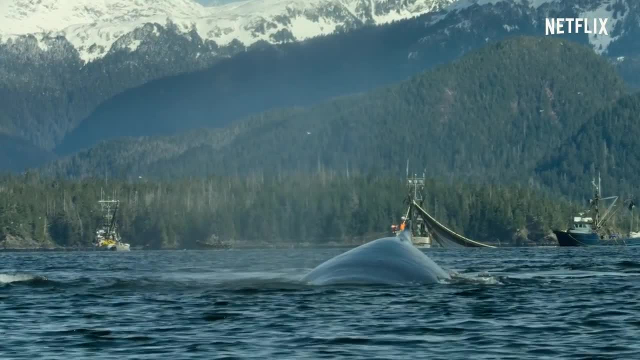 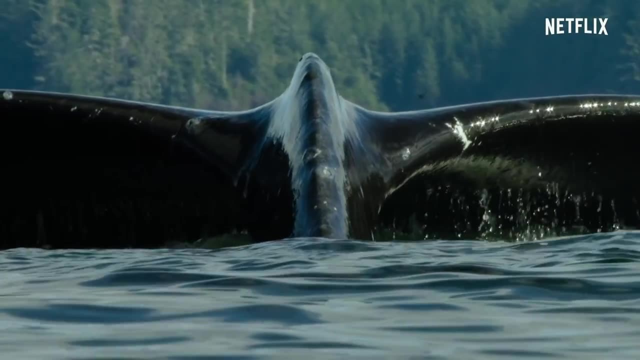 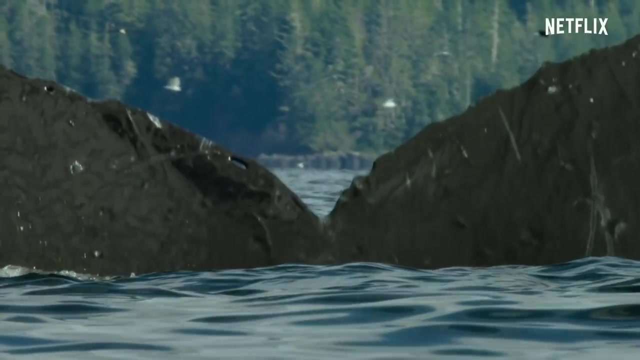 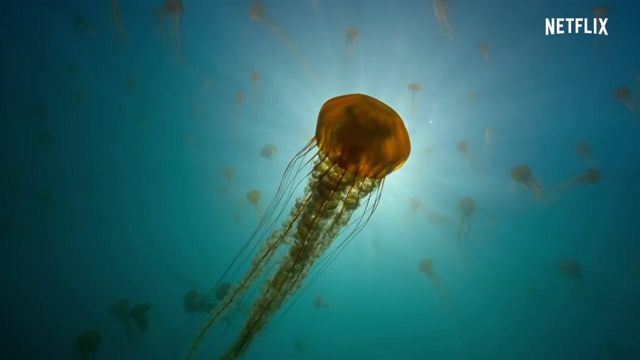 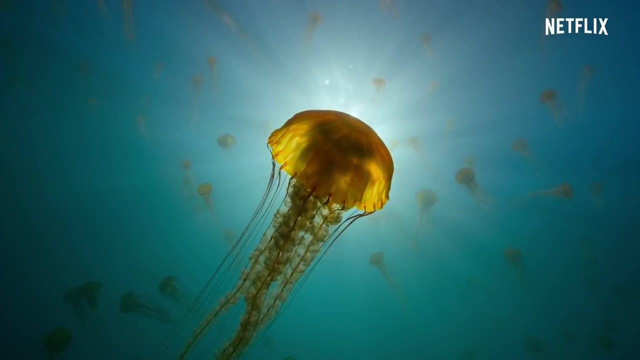 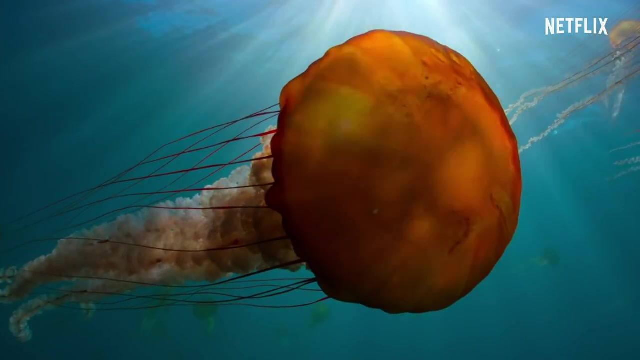 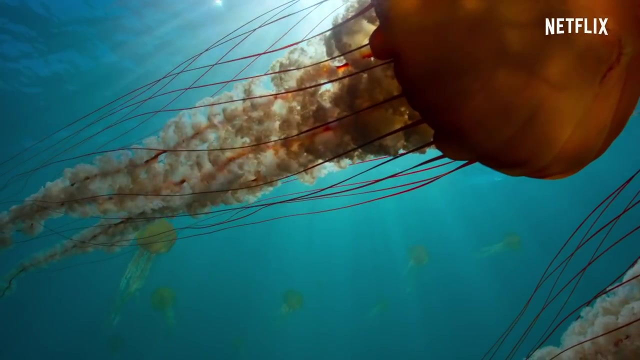 Many of the world's fish stocks are now in serious decline. A third of them have collapsed. In coastal seas, jellyfish are taking over waters that were once dominated by fish Compass. jellyfish have an ethereal beauty, but they provide very little sustenance for other wildlife or us. 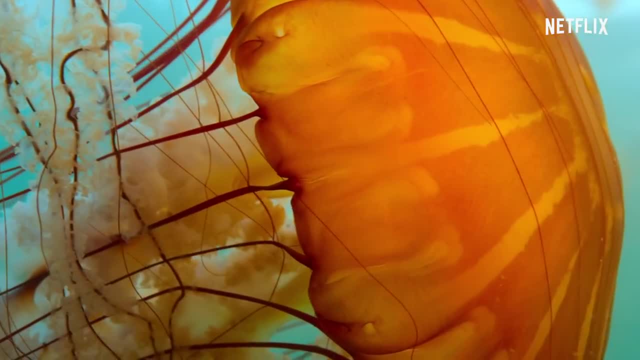 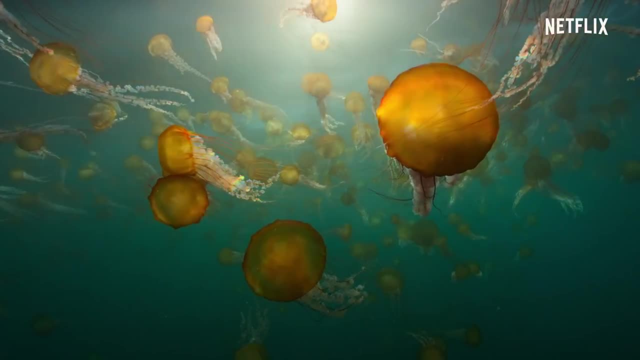 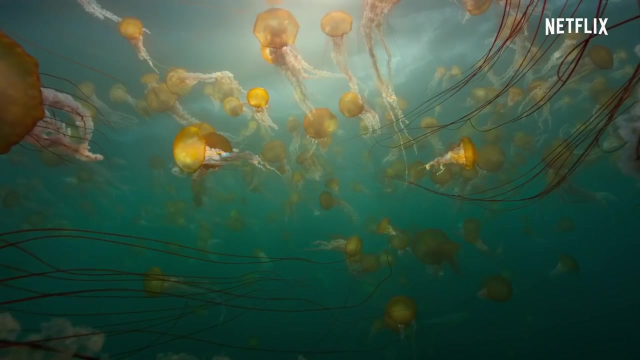 These fish are no longer a source of food for the earth. They're a source of food for the sea, But they're more like a source of food for the seas. In the South they produce a huge amount of fish which are a sort of food for the sea. 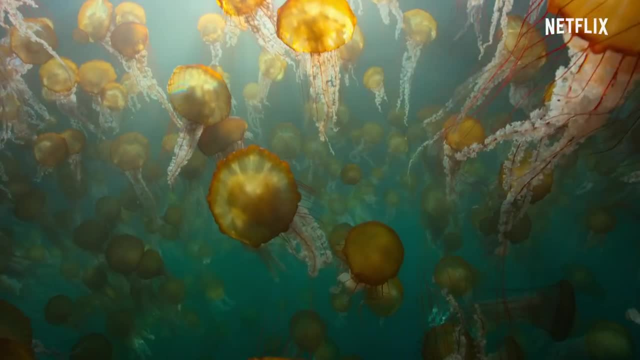 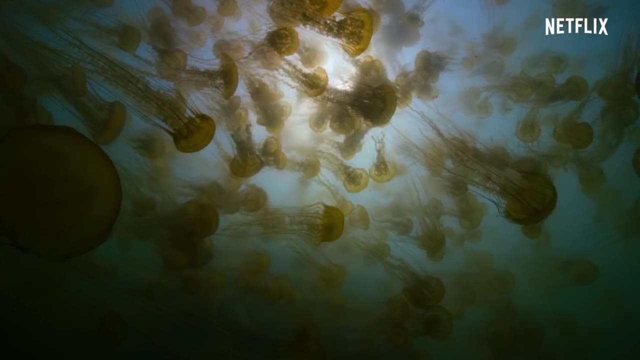 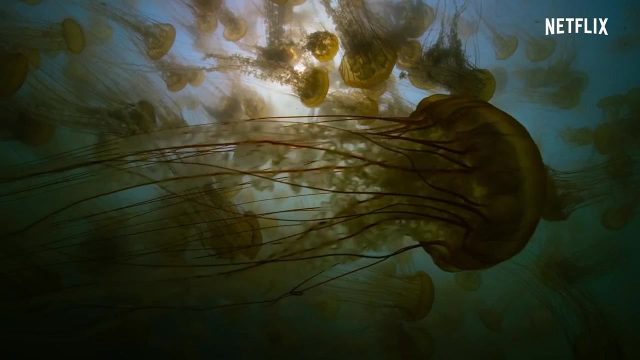 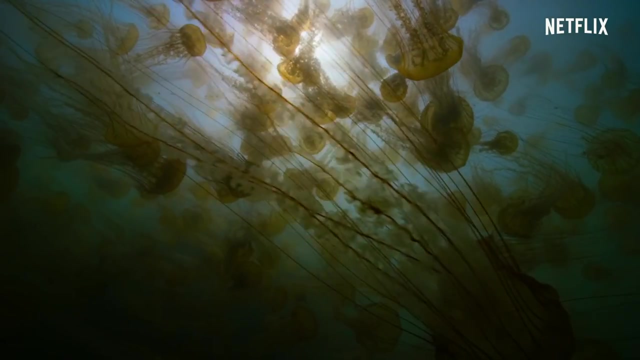 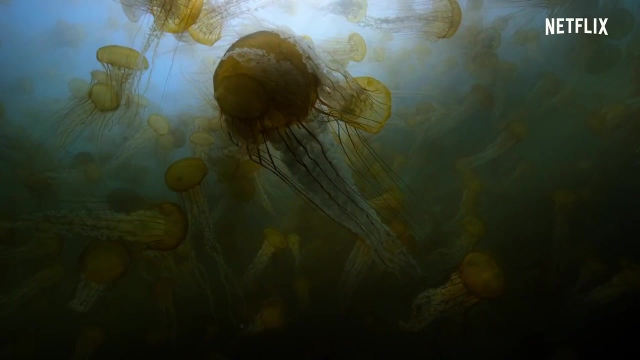 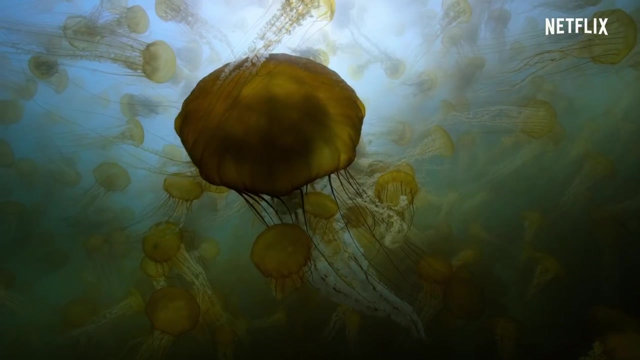 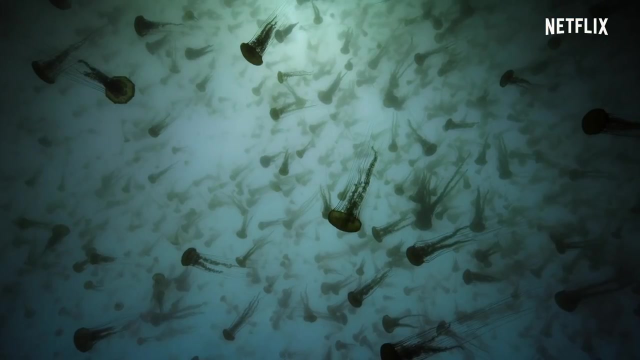 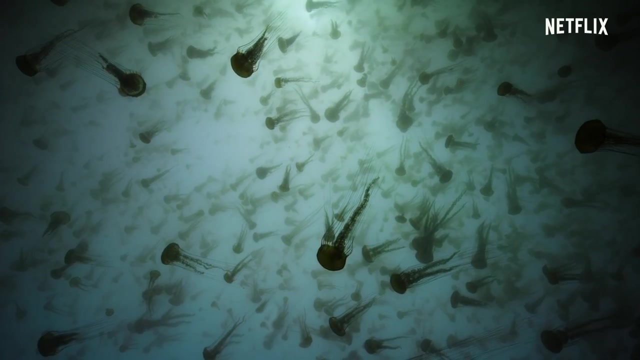 These immense swarms are becoming increasingly common, a worrying sign of a serious imbalance. Unless we start to fish sustainably, our seas, once so bountiful, will be filled with little more than vast swarms of jellyfish. But the future does not have to be like this. 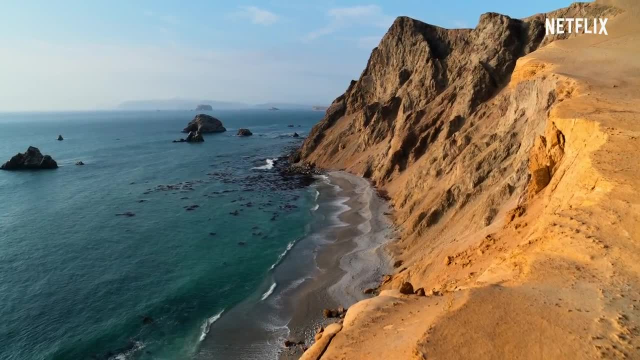 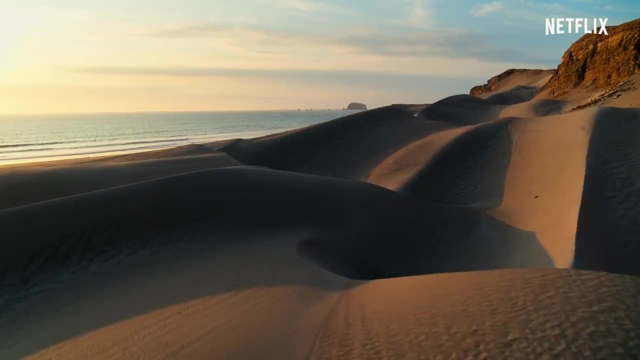 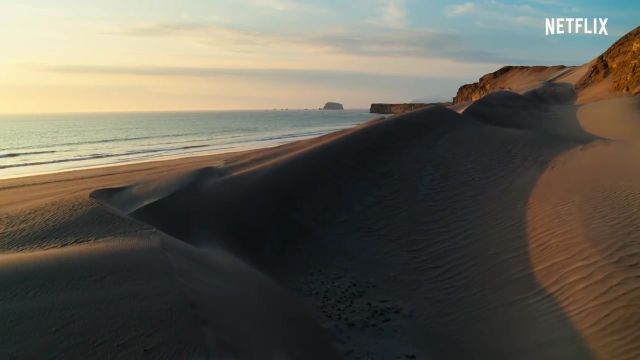 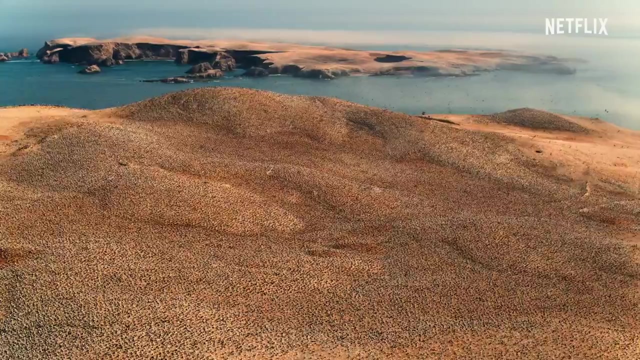 On the Pacific coast of South America, we can see how the oceans can recover The Atacama, the world's driest desert Inland. it's barely able to sustain life of any kind, And yet the coast could not be more different. 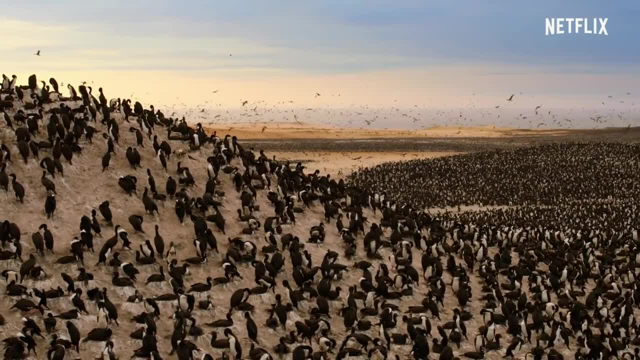 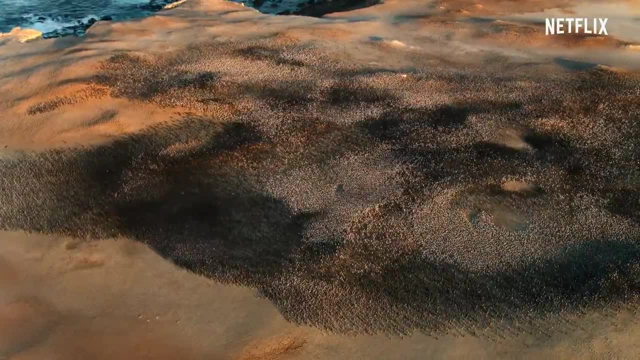 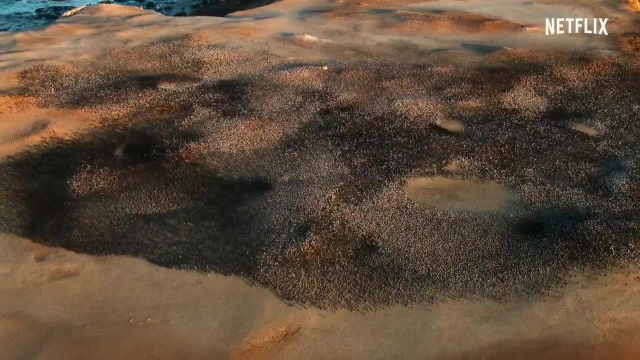 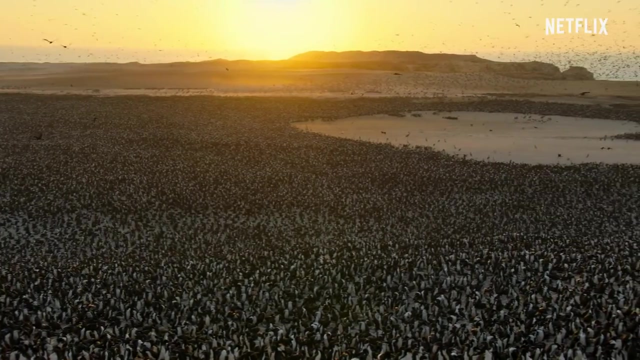 For centuries, seabirds have been a part of the ocean. Seabirds have gathered in millions on these desert shores, But 50 years ago the great colonies disappeared because we overfished the local waters. Controls were introduced and now the fish stocks are recovering. 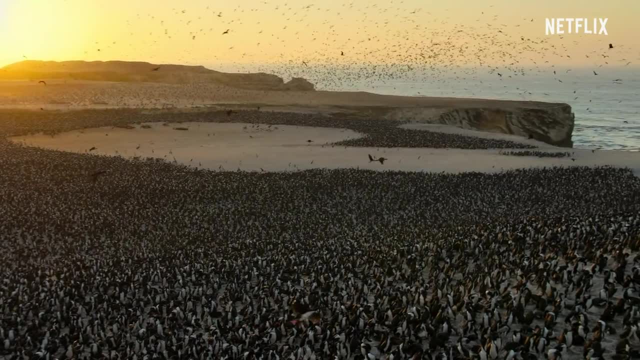 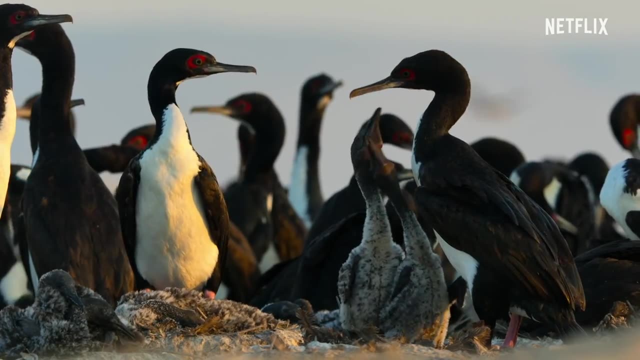 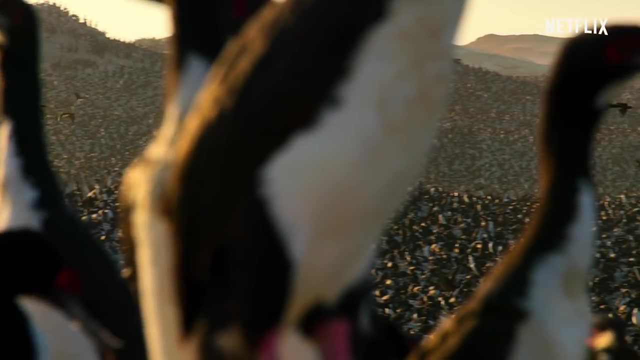 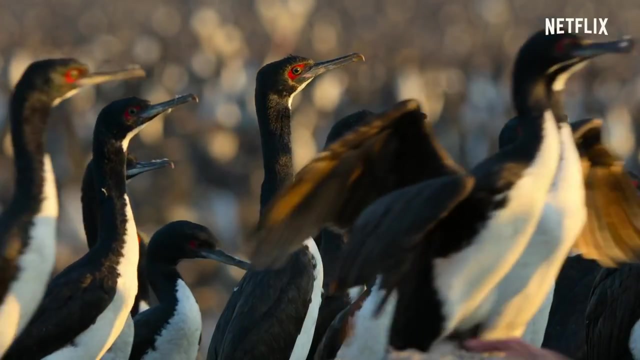 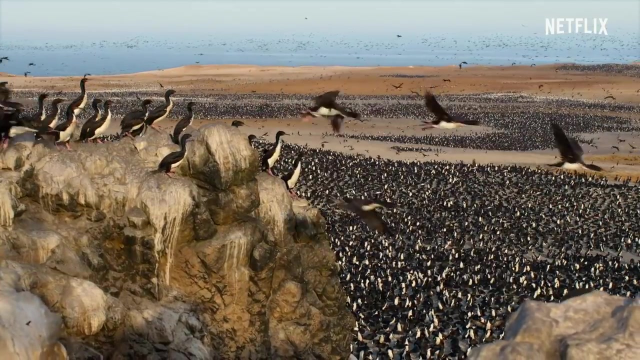 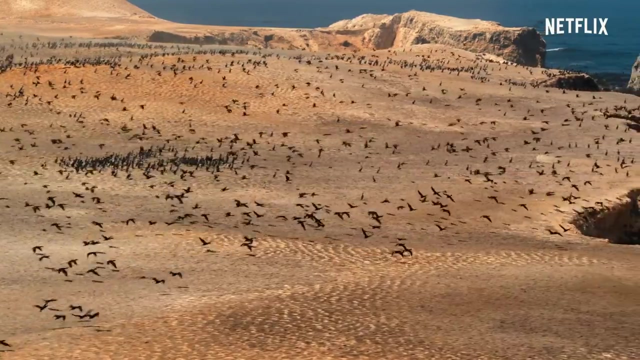 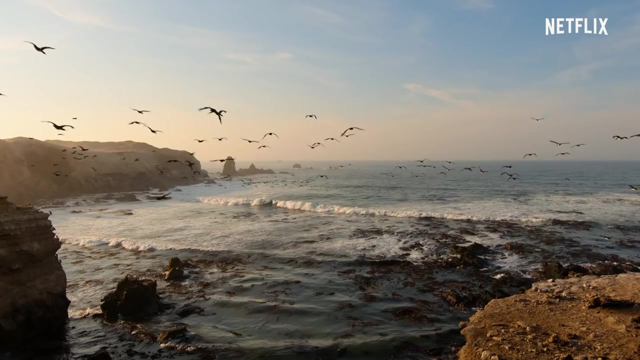 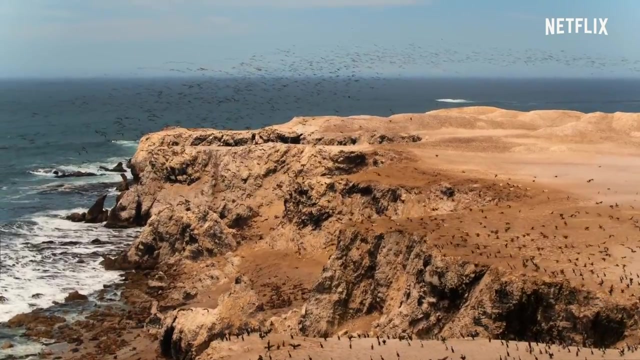 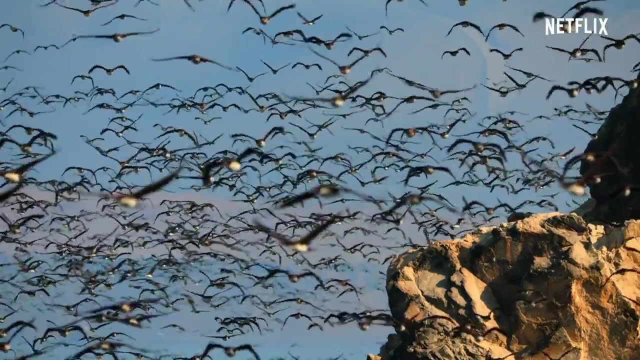 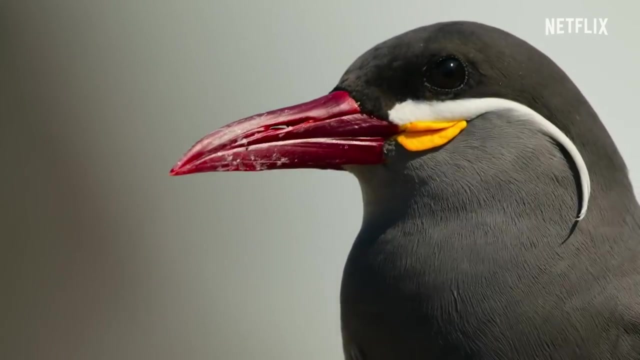 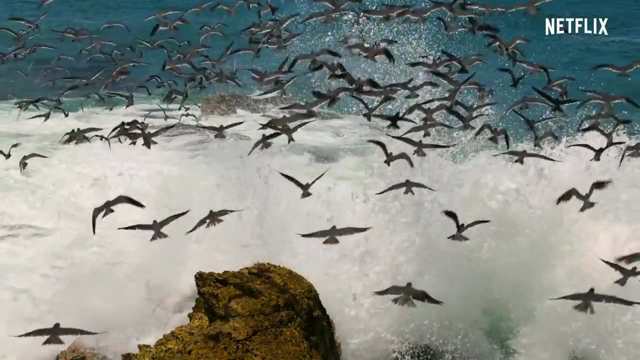 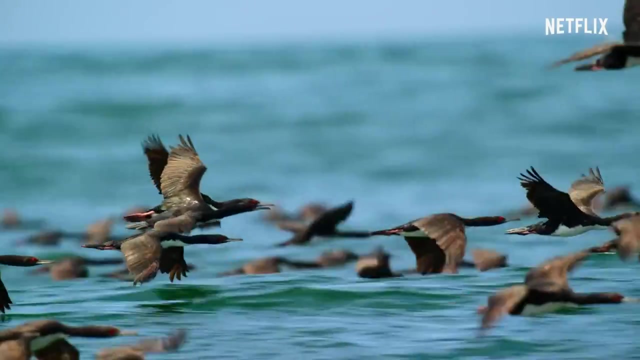 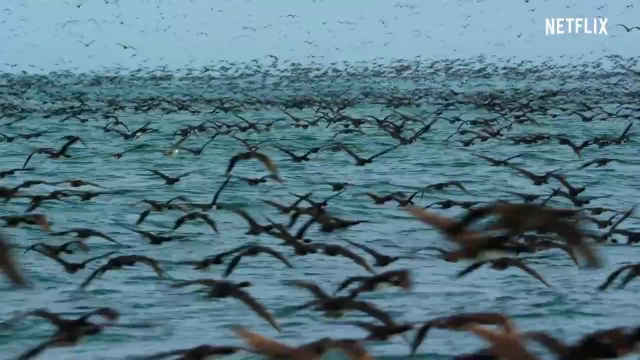 So today, 3 million guane corals assemble each year to recover The, The, The And So the, We, The And The, The, The, We, The, We, The. The colonies are so vast they take over an hour to empty. Beginning the procession, Inca, terns, Peruvian boobies, a great caravan of hunters all searching. 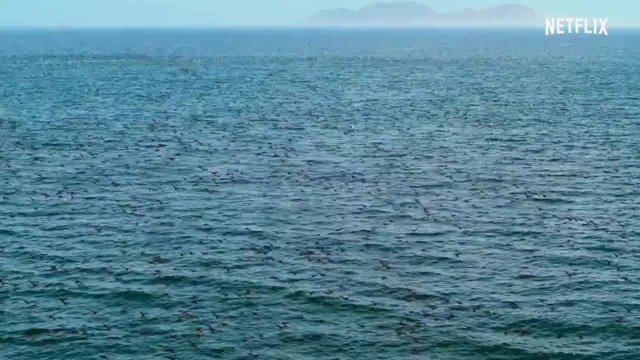 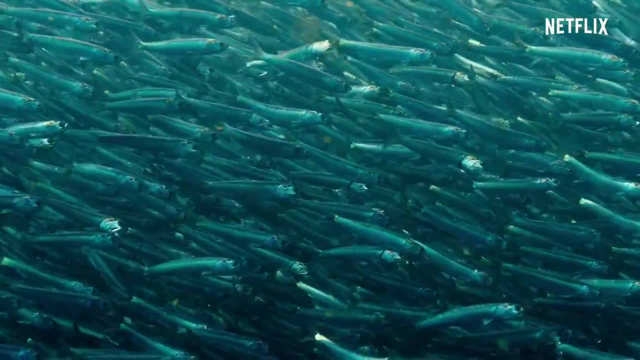 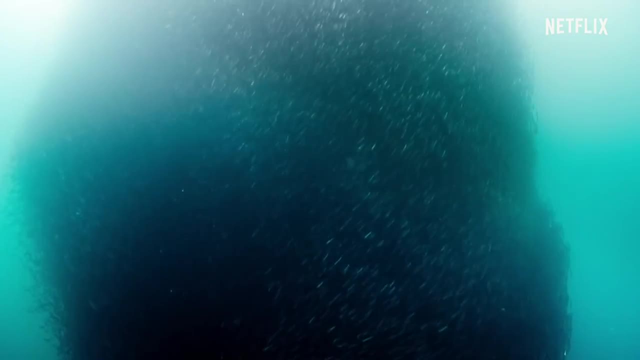 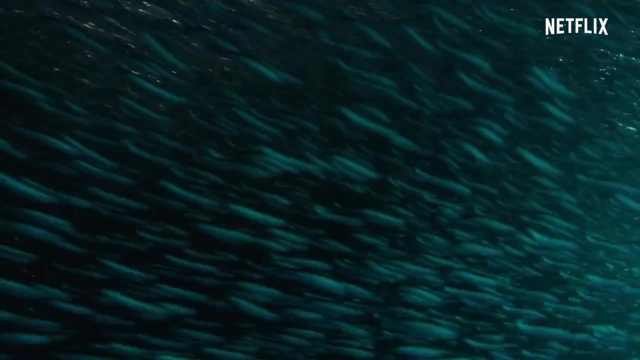 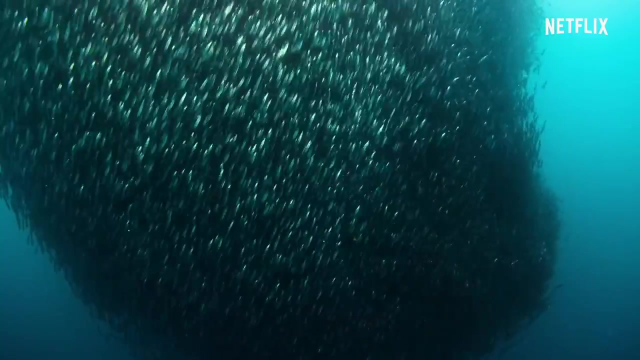 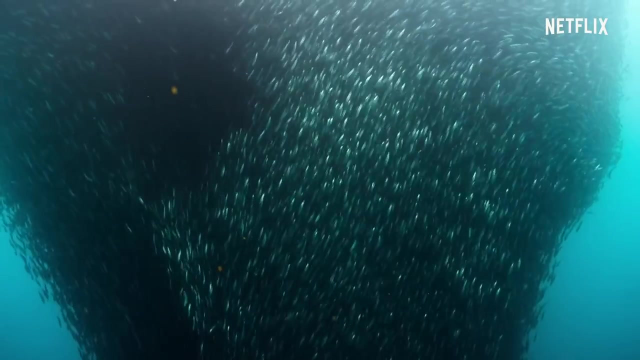 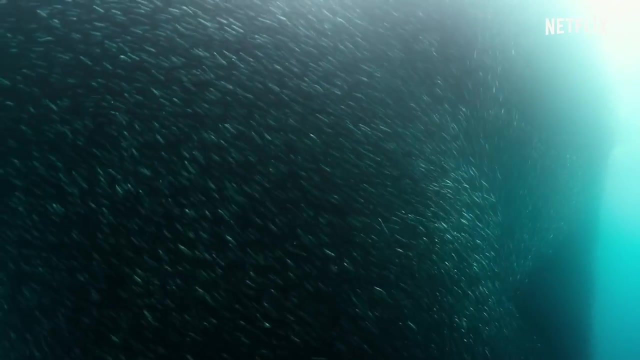 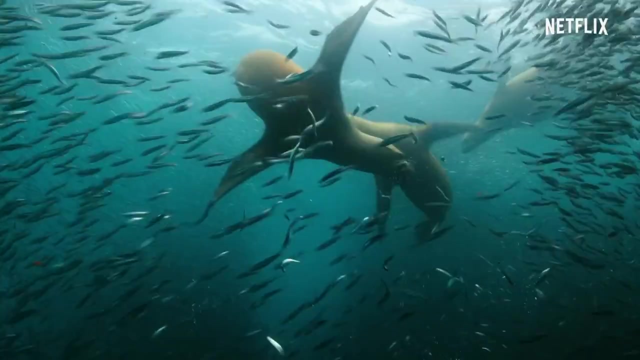 for the same thing. These little fish are so abundant that they support the greatest fishery on our planet. Astonishingly, they can account for a tenth of all the fish we harvest from our oceans every year. Sea lions are first to find the shoals. 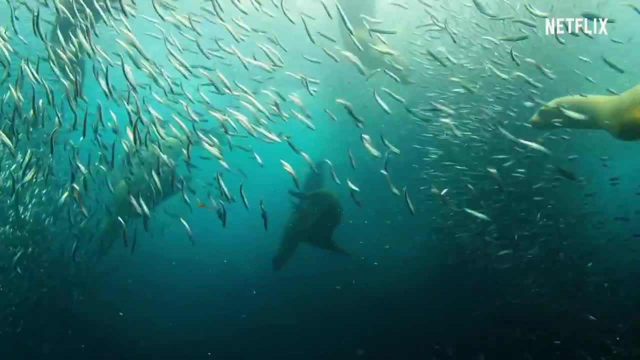 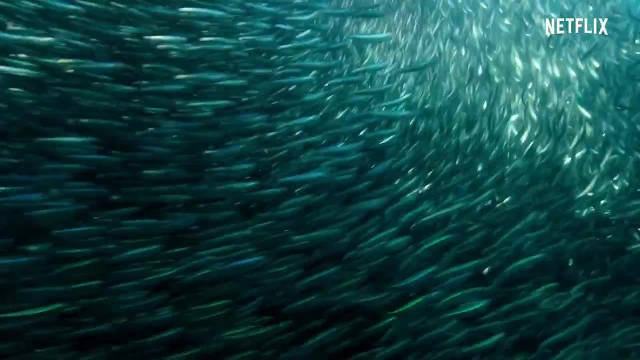 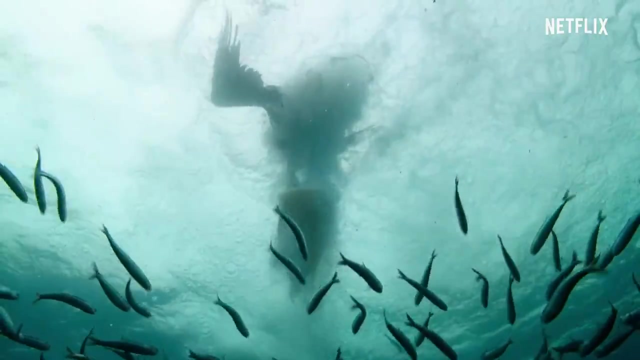 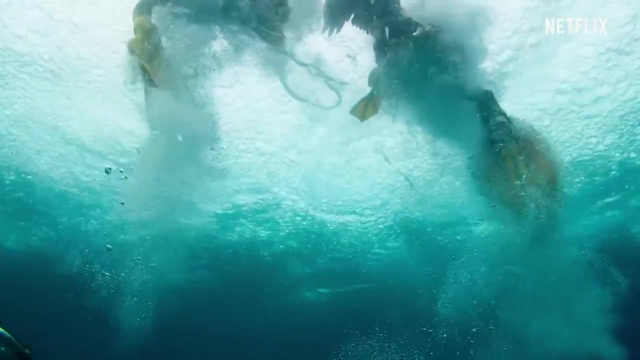 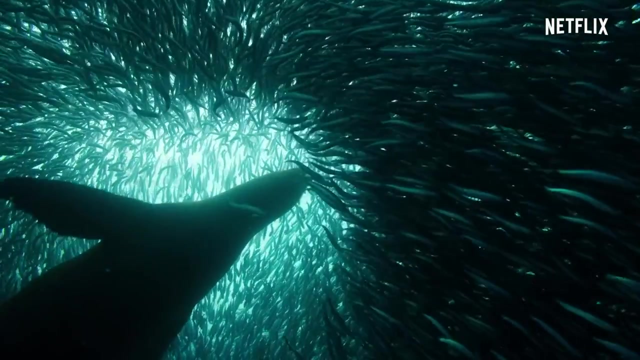 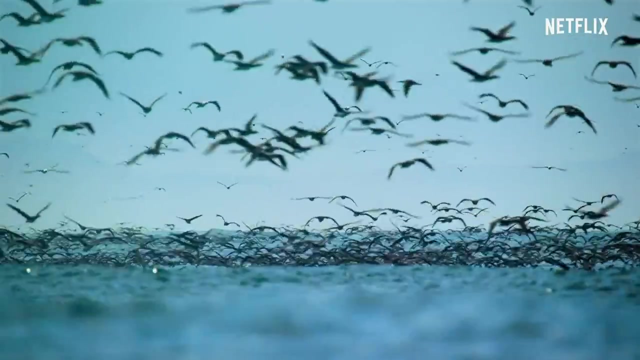 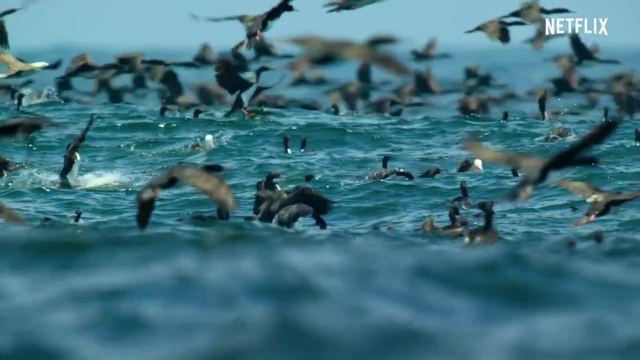 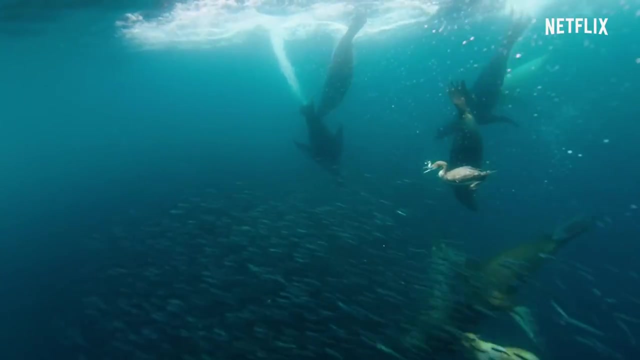 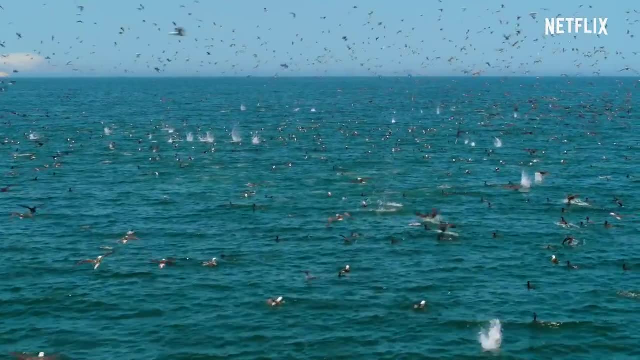 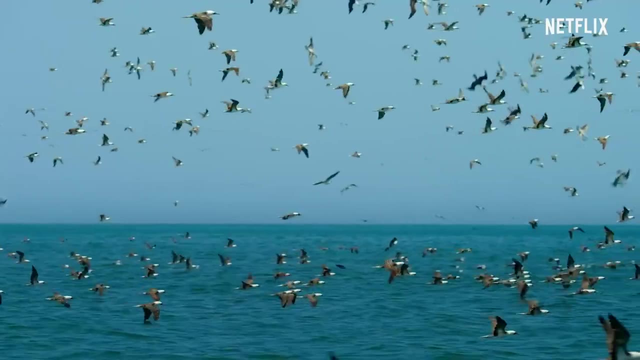 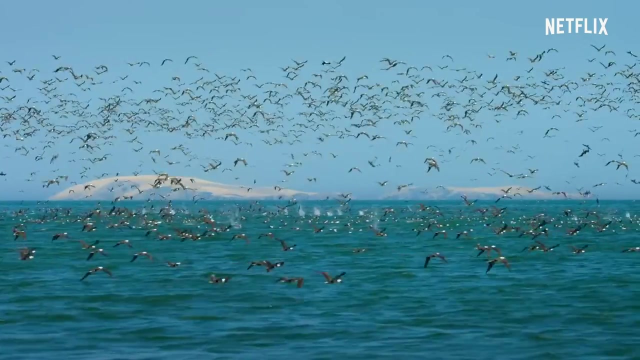 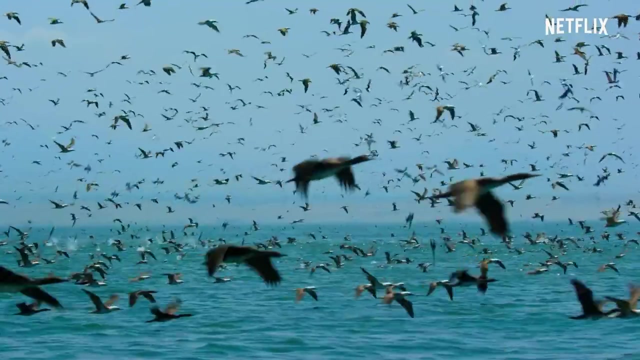 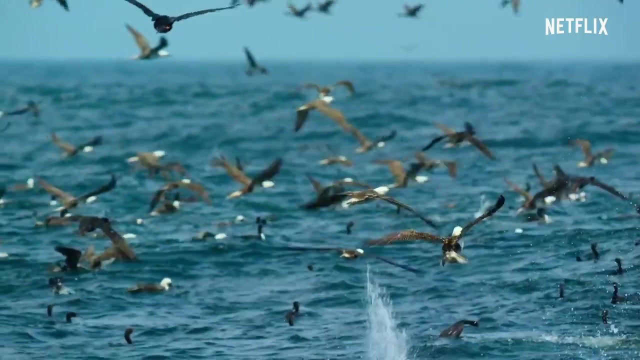 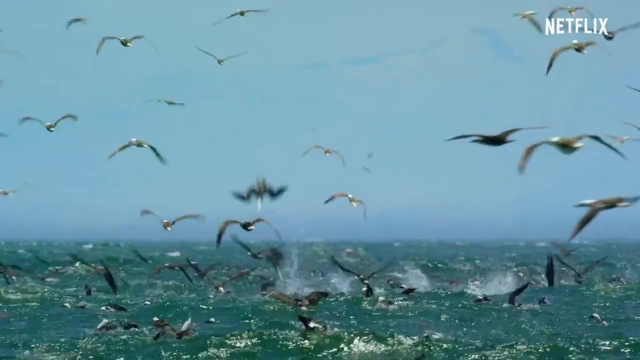 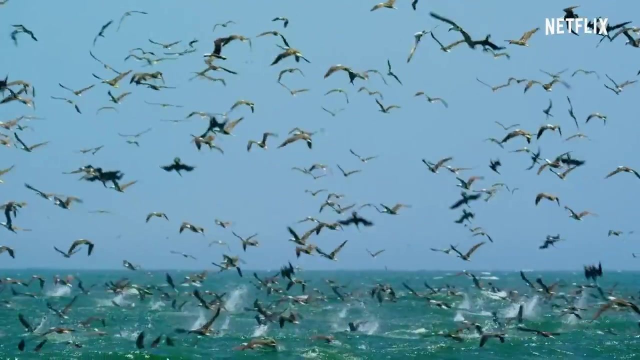 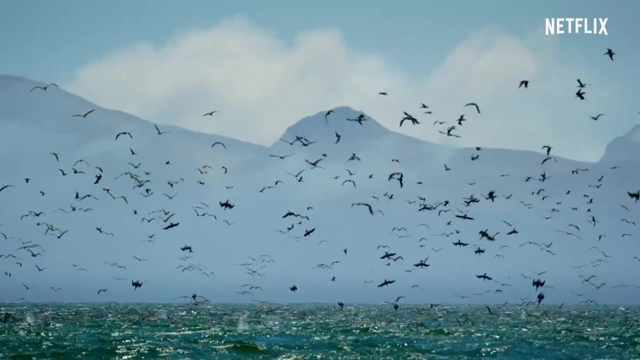 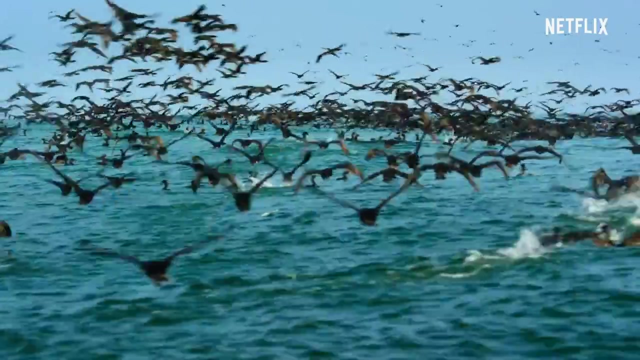 Corvins dive to grab their share. The rubies strike from heights of 20 meters. They hit the water at 100 kilometers an hour. They hit the water at 100 kilometers an hour. They hit the water at 100 kilometers an hour. 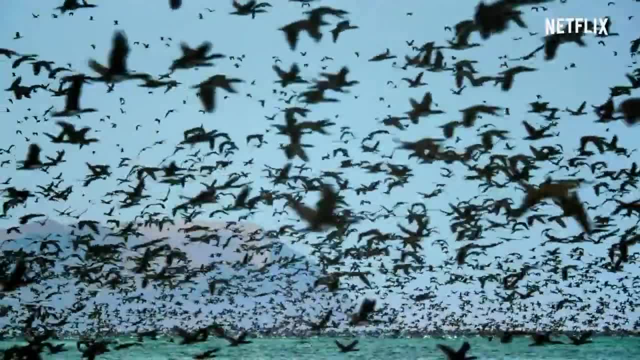 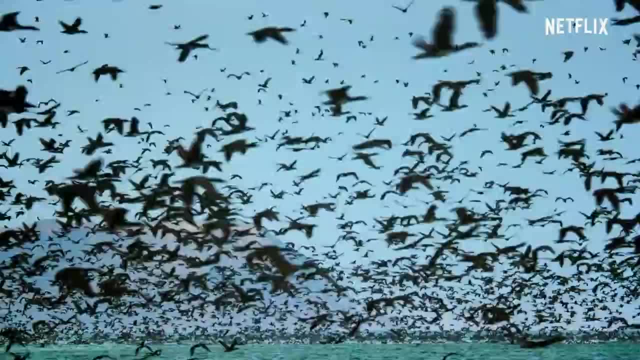 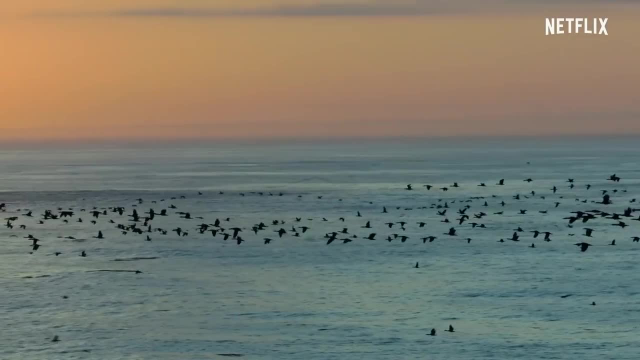 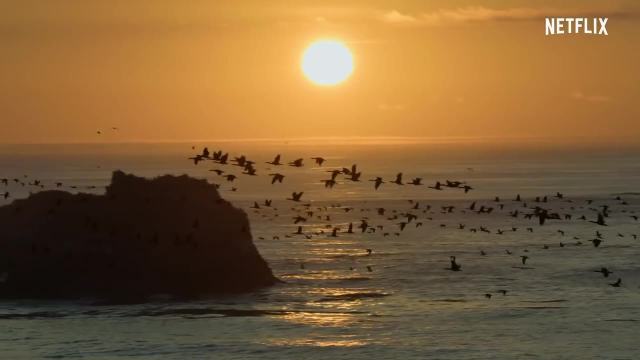 The lives of five million cormorants and boobies depend on the great shoals. Yet if we allow the anchovies to fully recover, they could sustain the 25 million seabirds they once did. It is a vivid reminder of the astonishing riches. 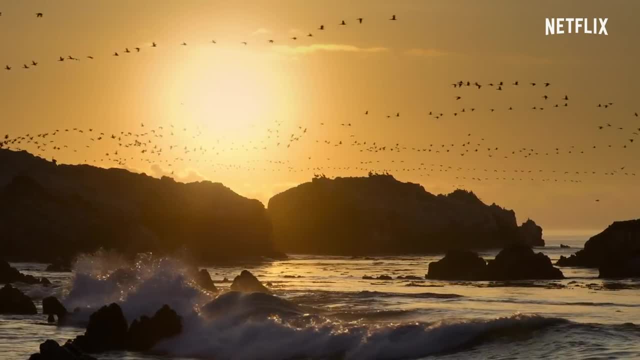 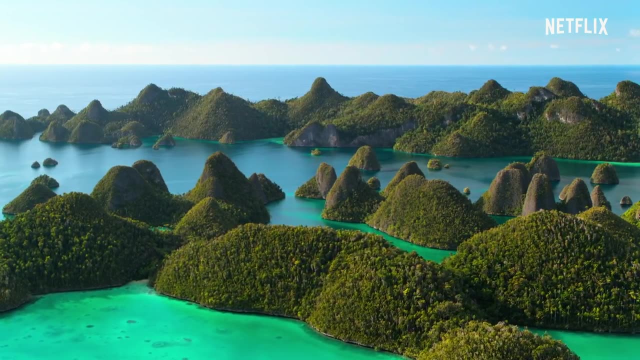 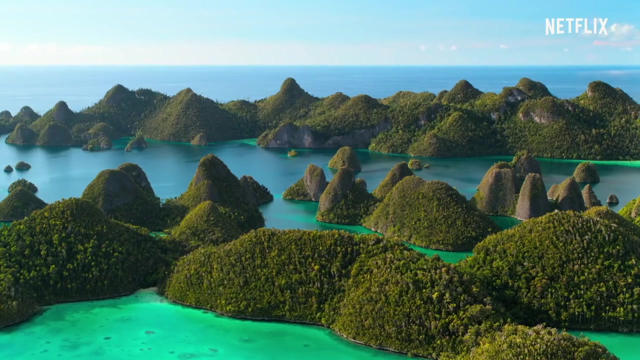 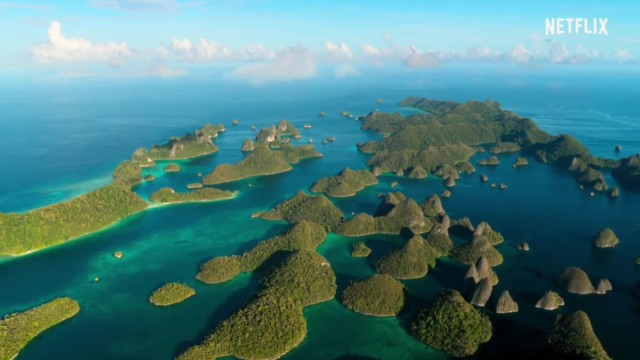 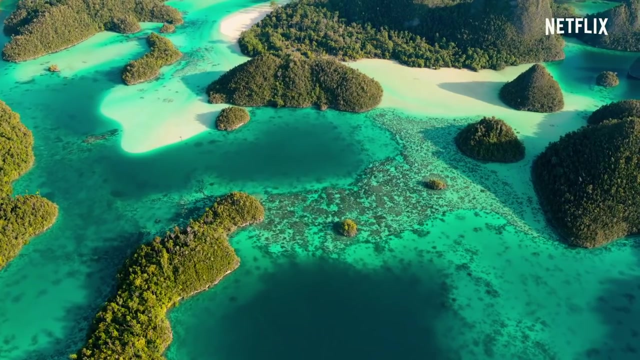 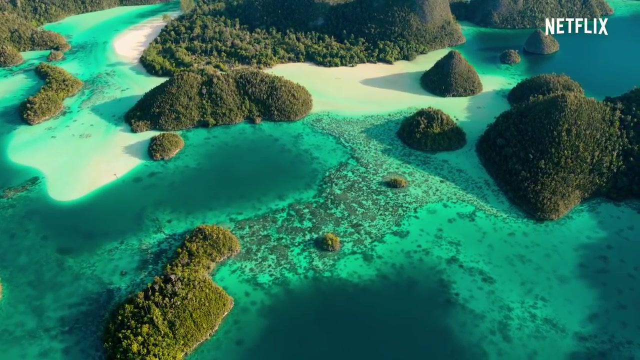 our coastal seas can support And when given the chance, they can recover surprisingly quickly. The islands of Raja Ampat in Southeast Asia. These seas were largely strewn and stripped of sharks and other large fish by years of unregulated fishing. This lagoon was once occupied by a shark fishing camp. 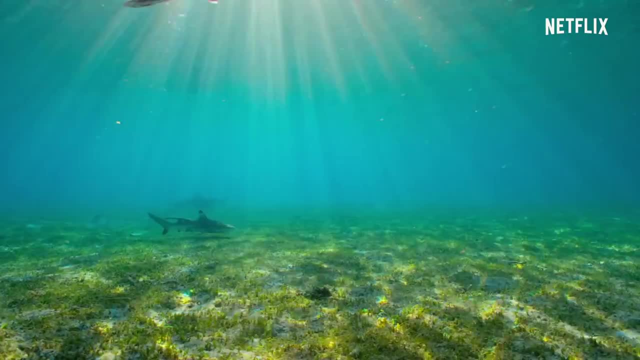 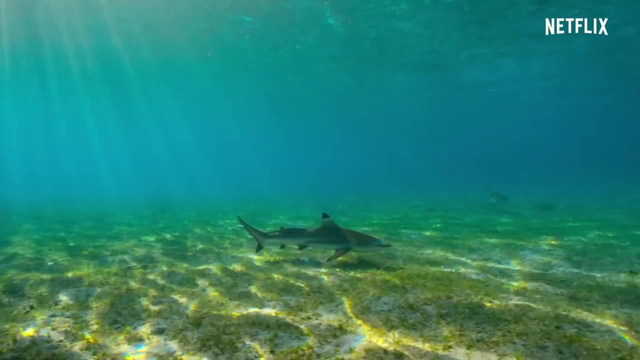 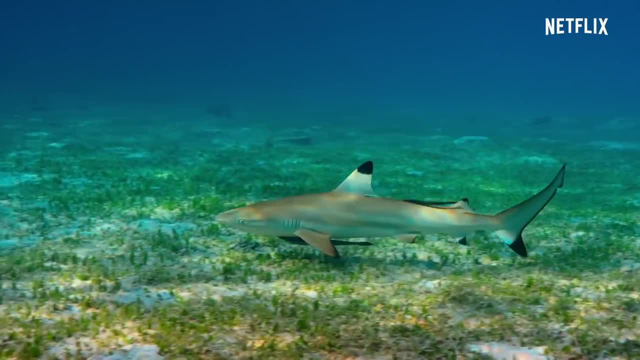 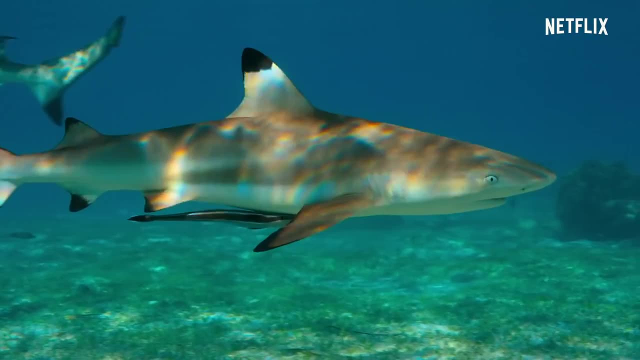 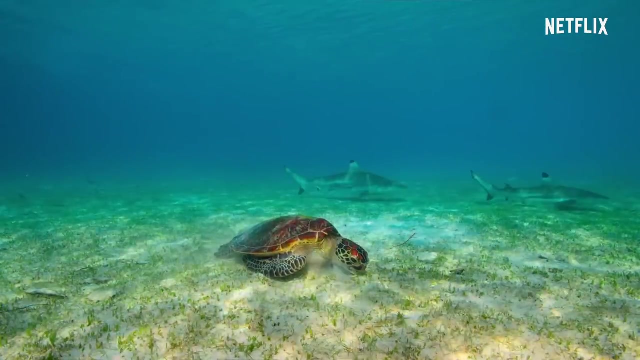 and the recovery has been miraculous. Today there are 25 times more sharks than a decade ago. Turtles that used to be hunted now peacefully graze on the sea grass. Turtles that used to be hunted now peacefully graze on the sea grass. 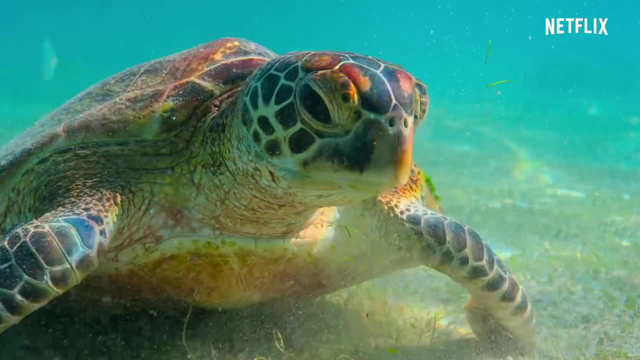 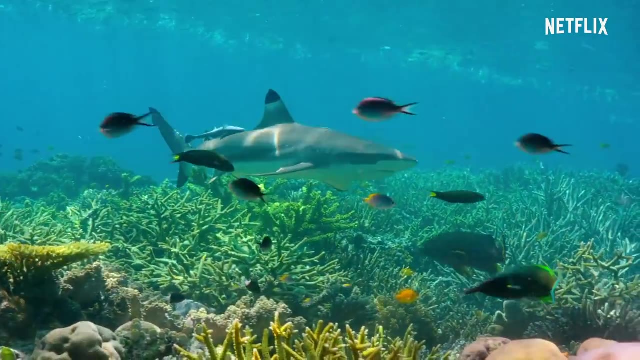 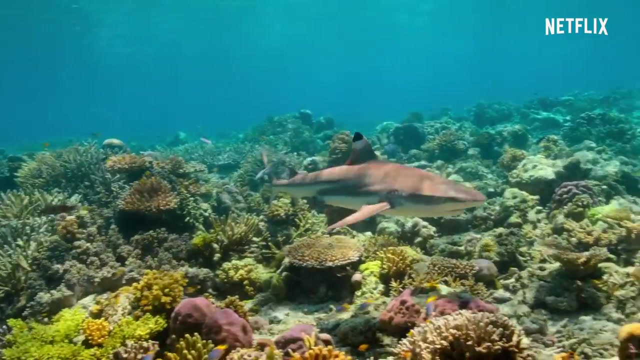 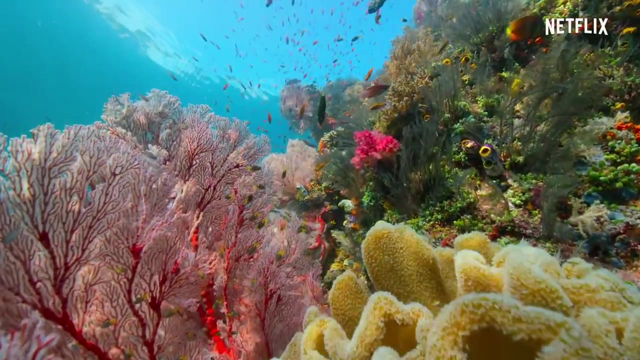 Now they are active and active again. Sharks are returning to local reefs, helping to restore the balance community, giving them a greater resilience against the effects of coral bleaching. against the effects of coral bleaching. The local reef owners have agreed to show their support. 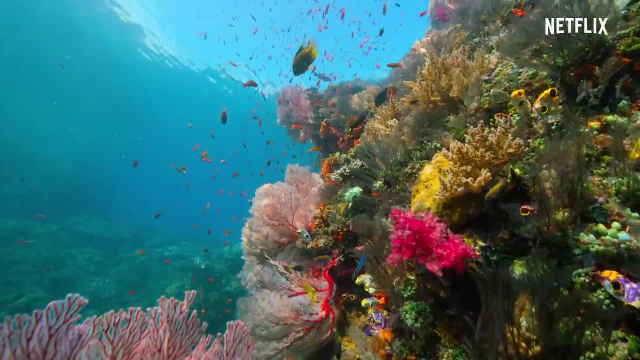 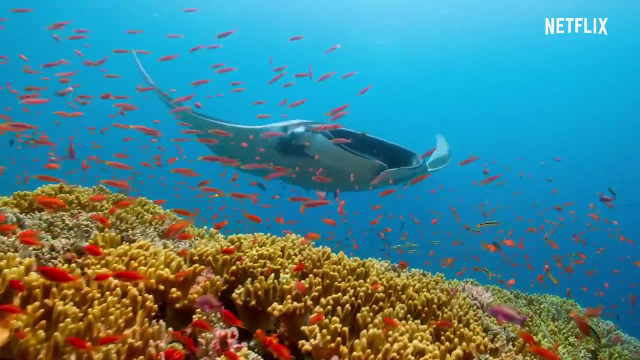 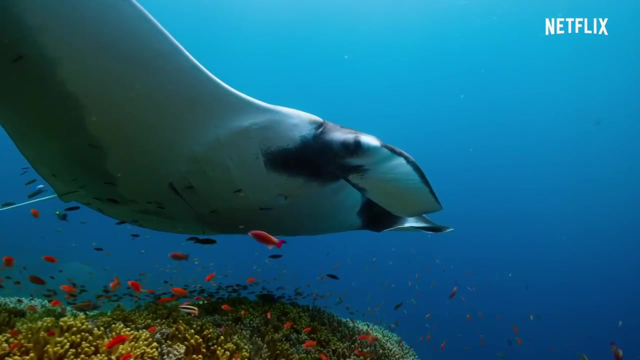 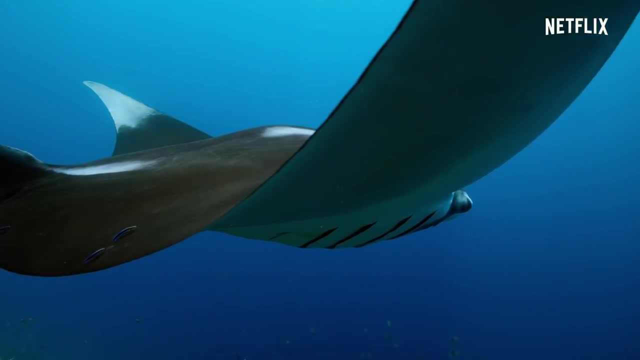 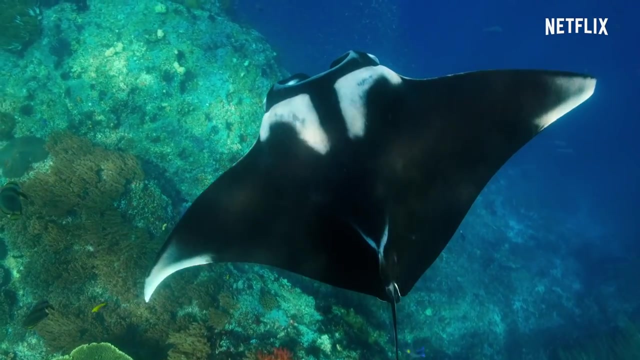 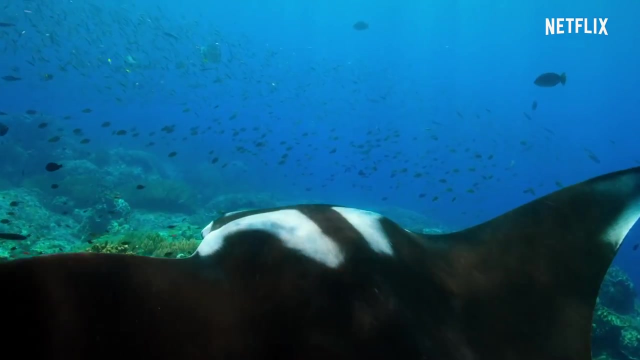 throughout the year, which gives them an opportunity to make progress in their lives. the local reef owners have agreed to show their support. Ocean-going manta rays Seven meters from wingtip to wingtip. These endangered giants spend most of their lives roaming the high seas. 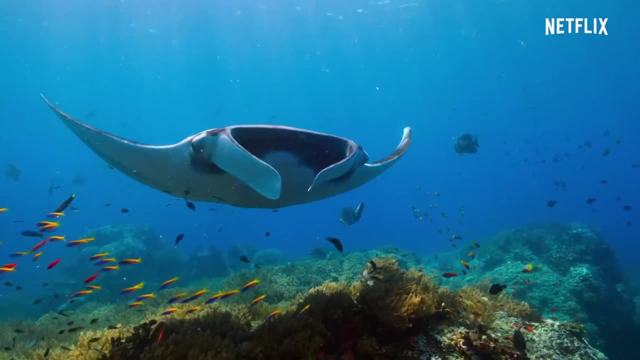 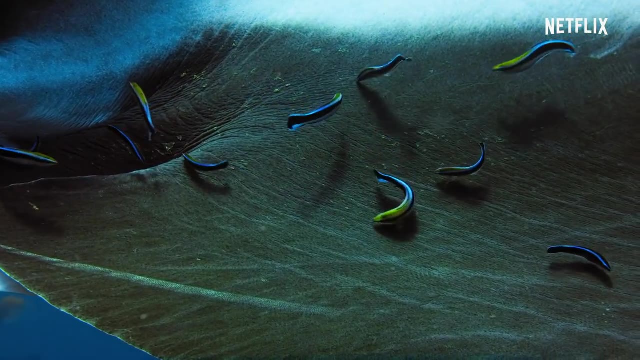 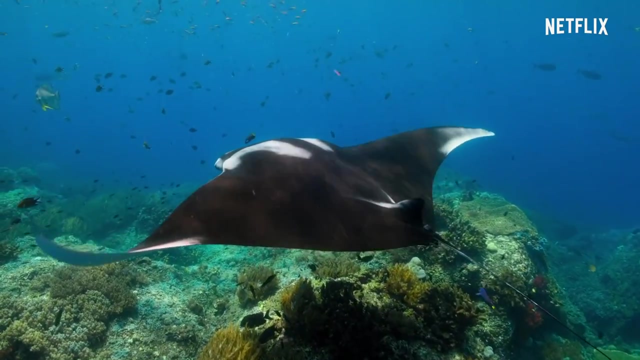 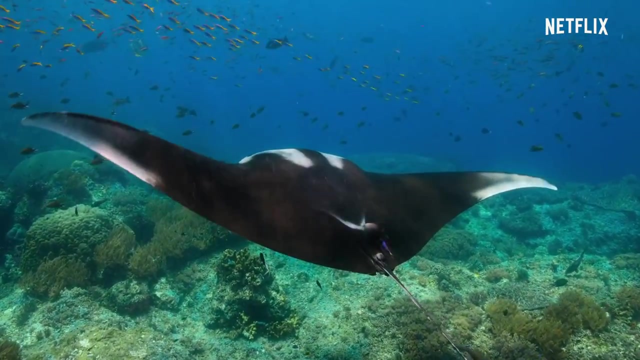 But now they are returning to this sanctuary to seek the attention of cleaner wrasse. Missoul is one of the few places on Earth where manta rays can be found, A place where biodiversity is actually increasing. Since protection, there are three times more fish. 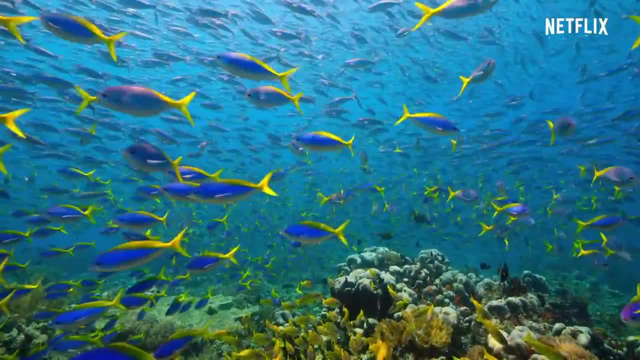 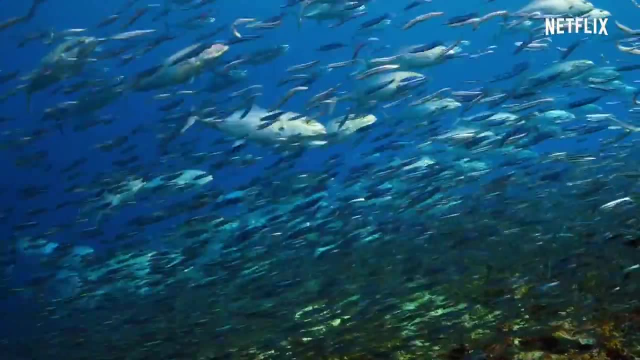 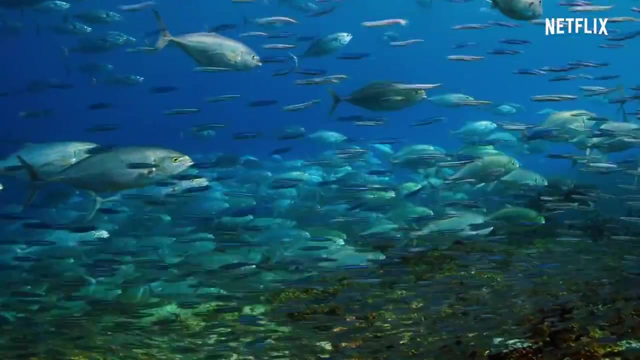 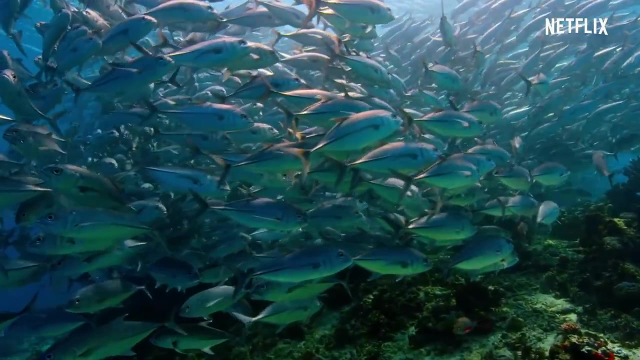 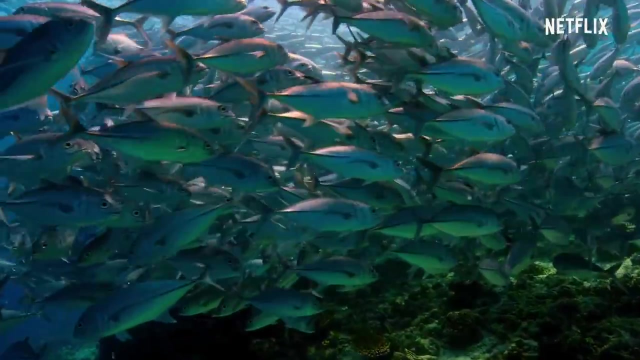 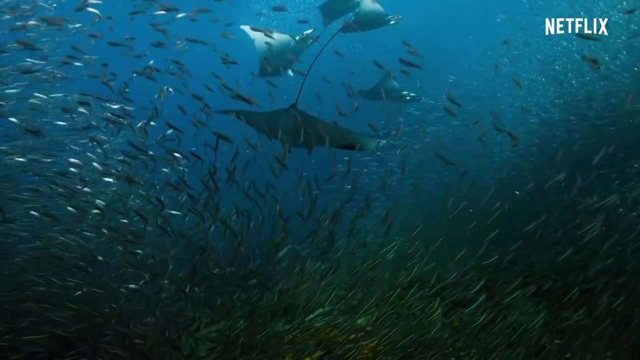 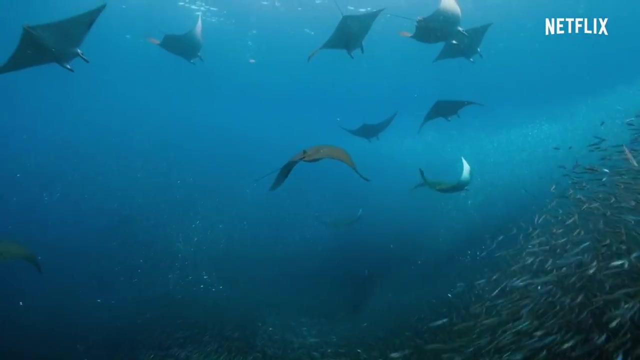 than just ten years ago. Fishermen working nearby waters profit from the overspill. They now catch more fish for less effort. We have far too few marine sanctuaries And in many commercial fishing is still allowed. We now have to clear the reef from manta rays. 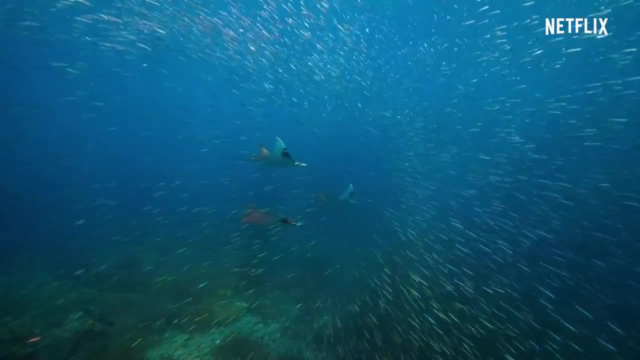 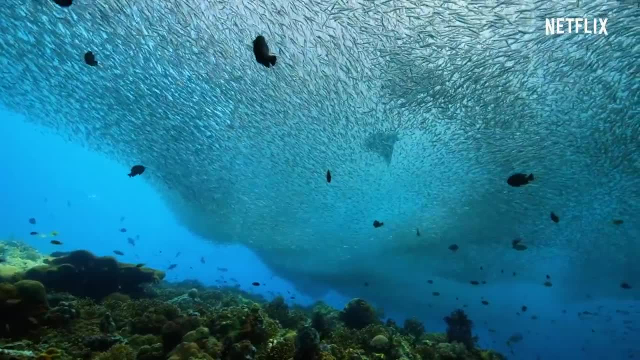 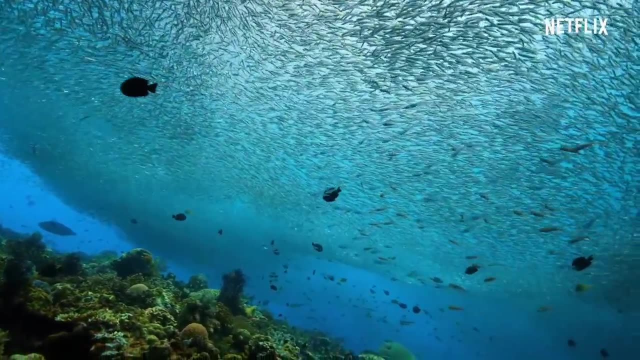 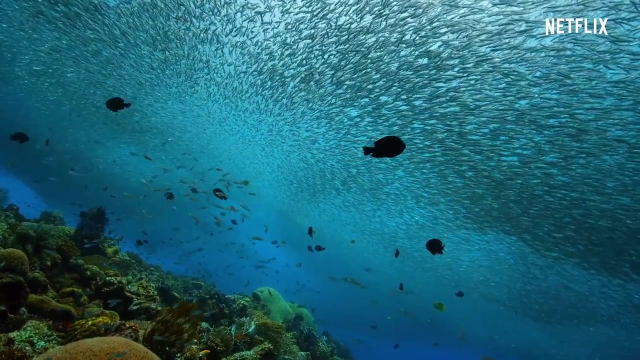 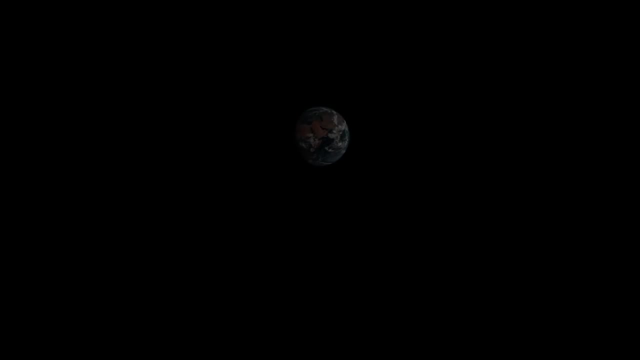 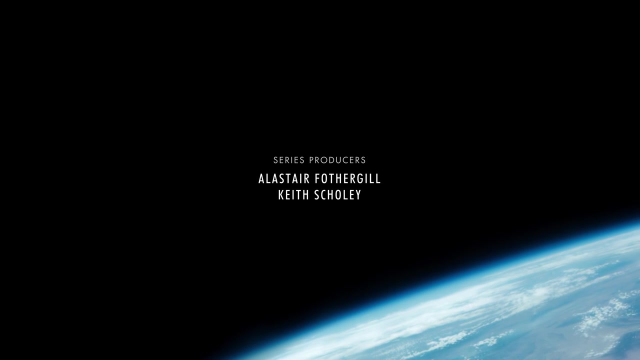 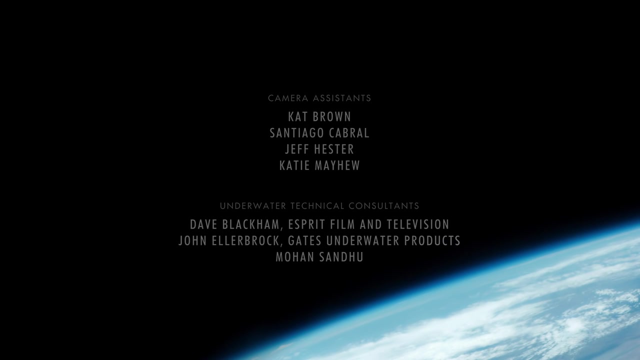 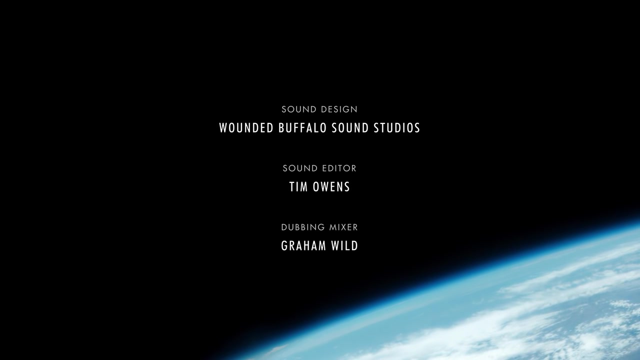 If we do that, our planet's fishing grounds would recover and help sustain both humanity and the rest of the natural world. Transcription by ESO. Translation by: —. Transcription by —. Transcription by ESO. Translation by —.